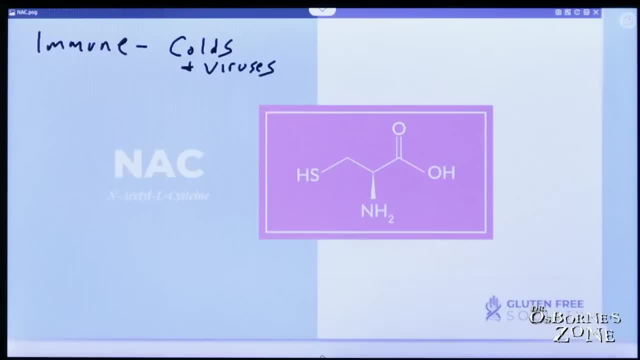 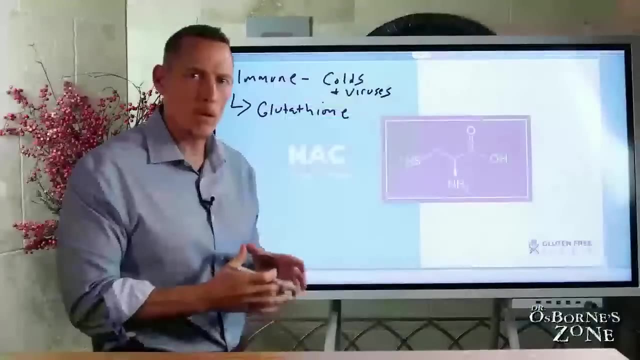 NAC is a primary immune system. it's a primary immune system driver for the production of something called glutathione. now, glutathione is a compound that your body produces. knack is the rate limiting ingredients. it's one of the main ingredients that goes into generating glutathione. when we think about what glutathione does, its primary role is to aid the liver in the detoxification of environmental pollutants and toxicants, and so when you don't have adequate glutathione, your liver basically can't do its functionality as well, cannot detoxify as well. this can increase the body's burden and therefore can increase the 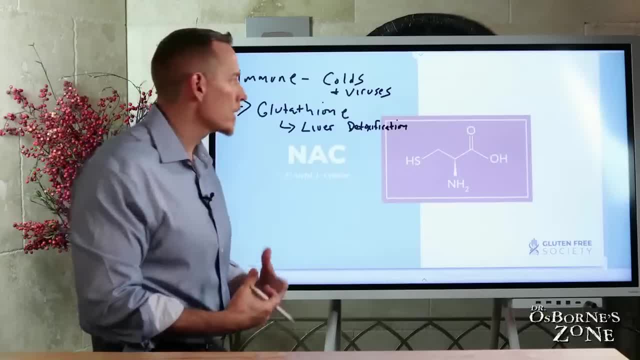 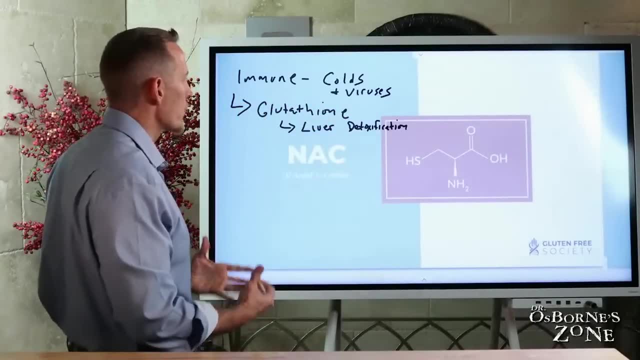 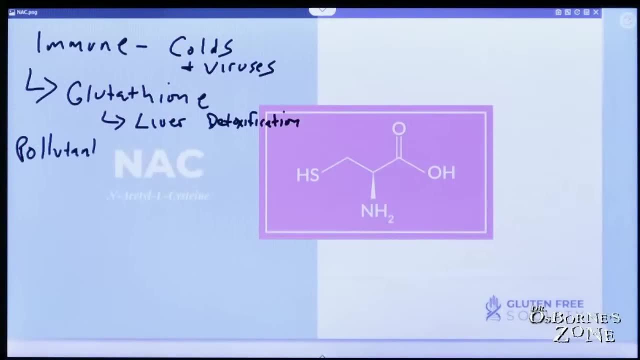 risk of developing things like chronic degenerative inflammatory diseases, autoimmune conditions. so we, the body, needs to be able to produce glutathione, and the problem with today's world is we're so overwhelmed with pollutants in the environment. so we got- we've got- things in the air, you know, you've got pollutants in the 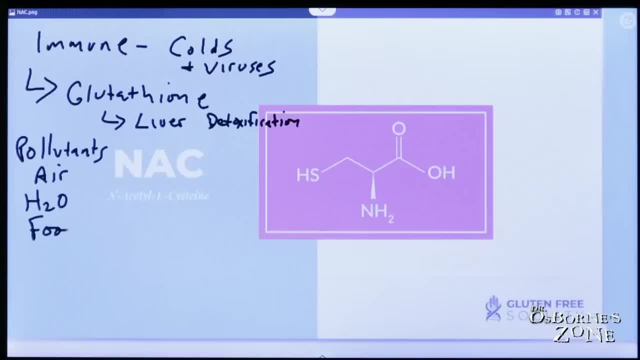 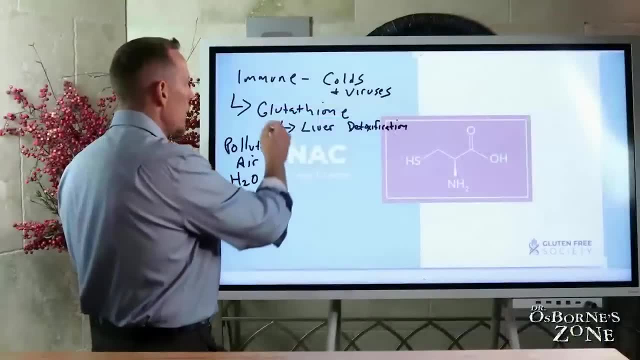 water. you've got a number of chemical compounds and additives, preservatives, pesticides and other things in the food. well, for all these things you're being exposed to, you need glutathione to be able to break those down and excrete them out of your body safely, and you're not going to. 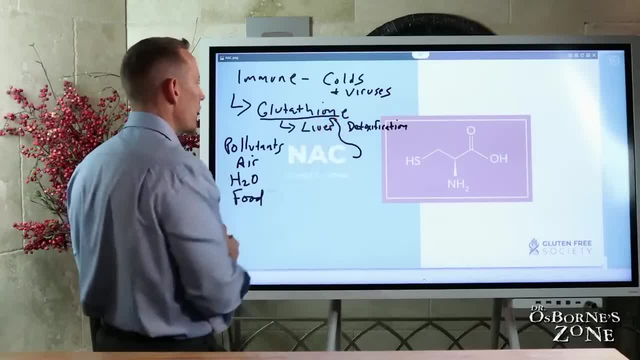 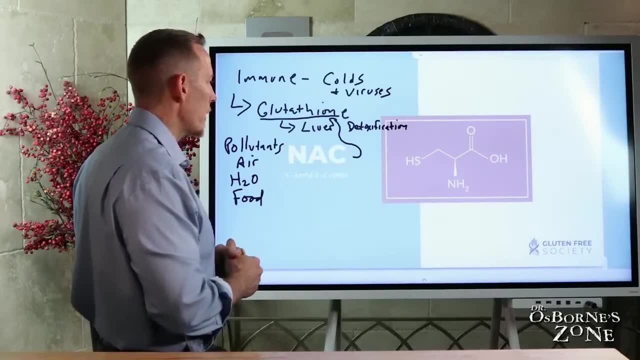 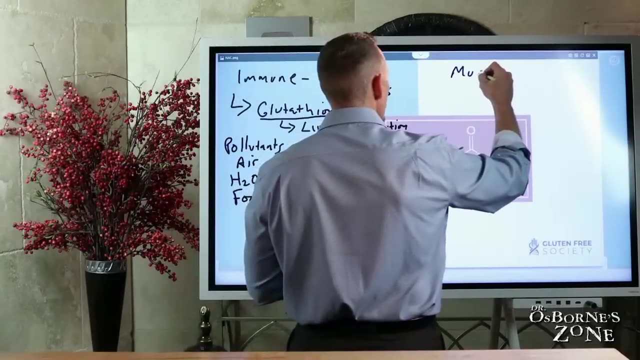 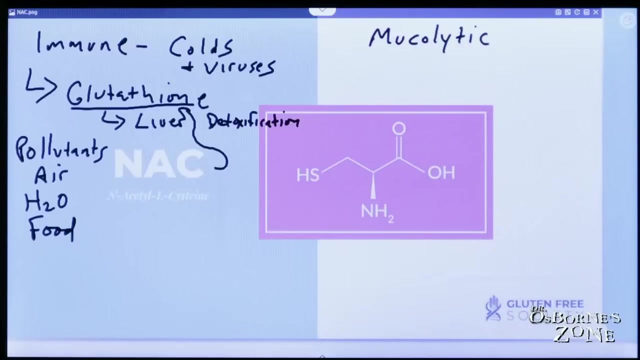 be able to adequately regenerate or supply the body with glutathione if you don't have enough in a pseudo cysteine or cysteine as an amino acid- again very, very critical, very, very important. now. one of its other major roles is in its properties as what's known as mucolitic. mucolitic means that it breaks down mucus. so those 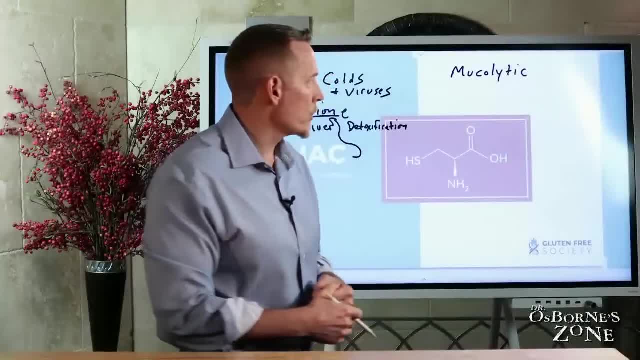 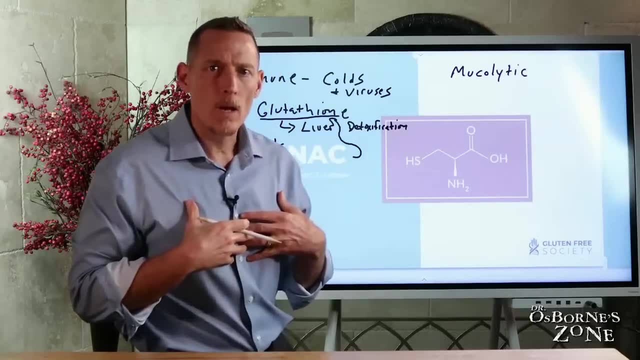 of you that struggle with any kind of chronic obstructive pulmonary issue. you know asthma, emphysema. if you've got a cold or flu and you've got heavy, heavy mucus in your lungs or heavy, heavy mucus in your lungs, you're going to have a lot of mucus in your lungs. 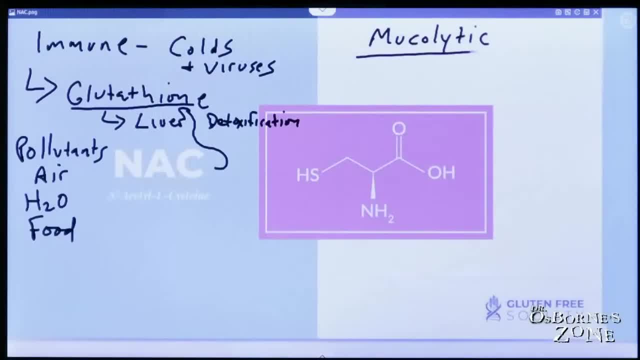 and you're going to have a lot of mucus in your lungs and if you have heavy, heavy sinus congestion, this makes in a pseudo cysteine knack. its mucolitic power is unmatched by anything else and this is very. this is a very, very powerful amino acid, meaning that you can go over and you can go over. 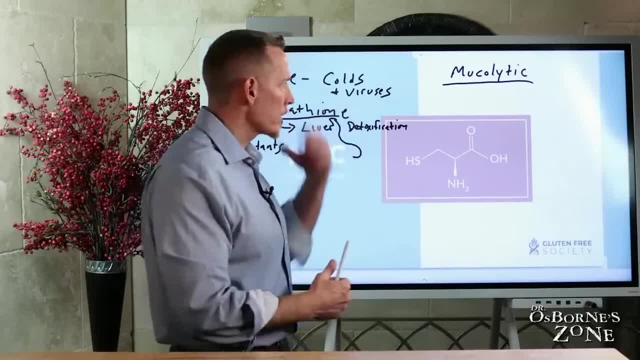 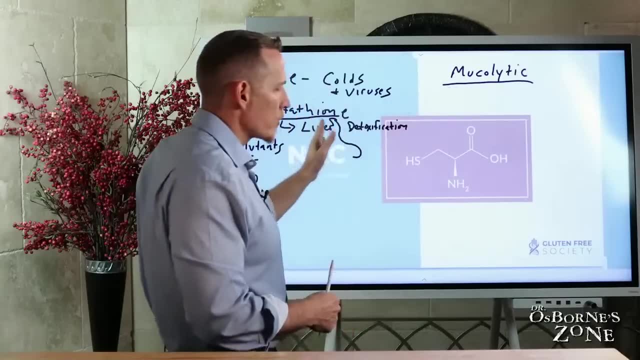 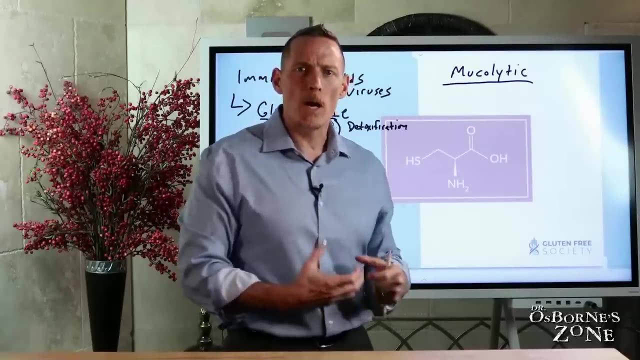 to the drugstore and you can buy a number of over-the-counter remedies you know, for sinus congestion and and for fluid retention, the lung, etc. but knack works better and it's natural and there aren't really any side effects and so there's no untoward other fillers or other ingredients. if you buy just a pure knack, you're. 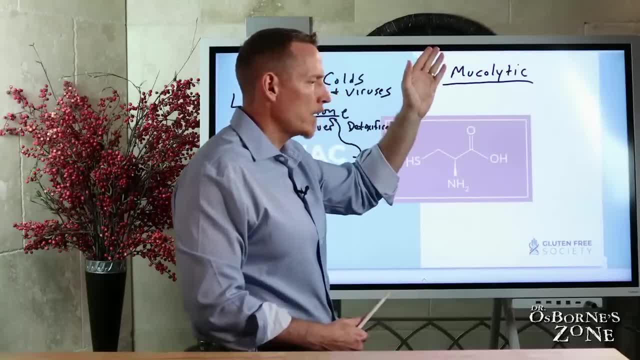 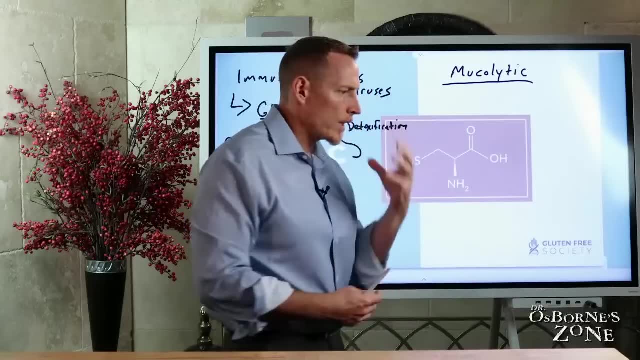 getting very, very powerful mucolitic without any downstream side effects that you obviously, that you wouldn't want, and and again a lot of people when they have that congestion, when they have that excessive mucus, one of the things that gravitate toward more than anything else in. 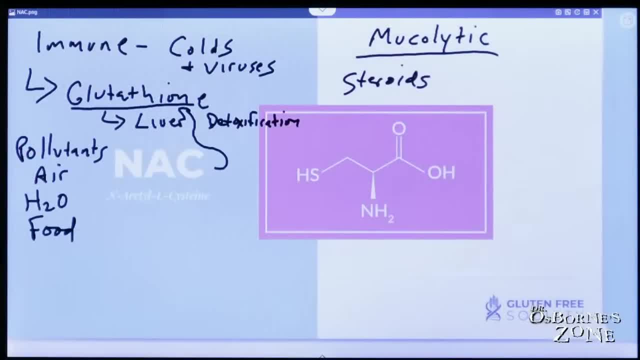 doctors a lot of times will prescribe steroids. and then of course you know steroids are anti-inflammatory, they they can help with that mucus production, but they depend on the body of your being. and so that's what steroids do? they deplete vitamin d and calcium. they deplete 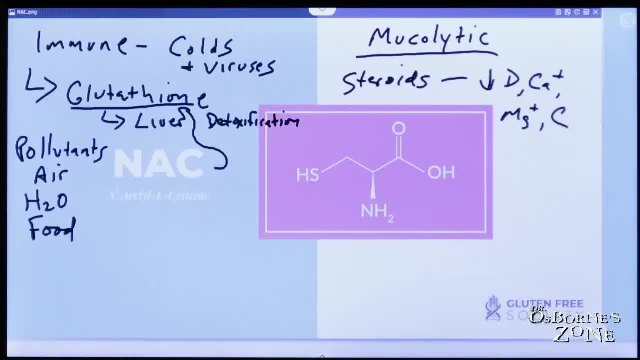 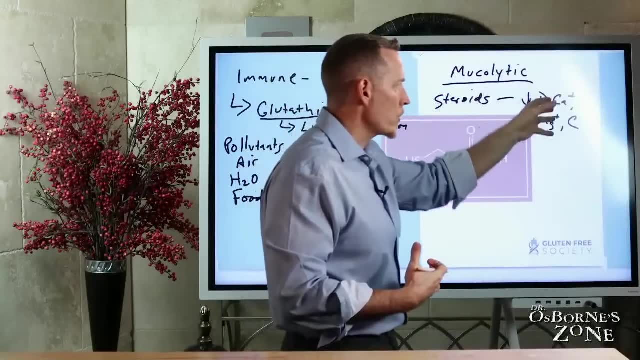 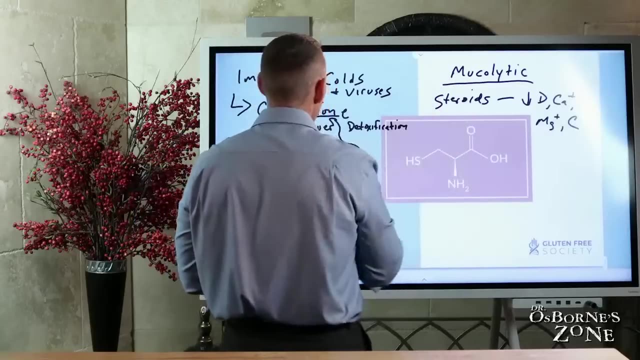 magnesium, you deplete vitamin c, and so if you think about, you know the consequences of causing these nutritional deficiencies. when we're trying to resolve an immune issue- and these nutrients are necessary for healthy immune function- you can see why steroids may not be as good of a choice as 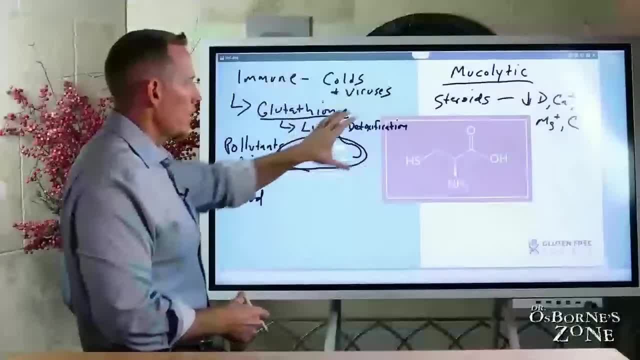 in acetyl cysteine as knack. so again it offers a natural way of managing the mucus around the body of the person. when they are just taking in their mucus, they reduce the mucus, or So again it offers a natural way to break mucus down and to improve upon immune support. 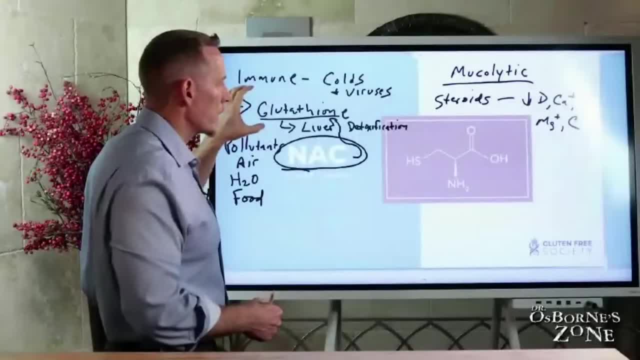 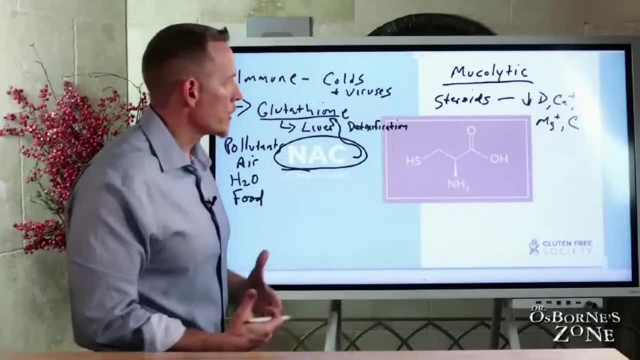 and function, but also a natural way to help with detoxification. So in my opinion, one of the biggest powerhouse amino acids therapeutically is in acetylcysteine. Now how much should a person take if, say, we're trying to get a mucolytic effect? If you're trying to get a mucolytic effect, 1,500 to 3,000 milligrams a day. If you're really sick, a cold flu, you can go that high upwards into that 3,000 range. If we're trying to just get good glutathione support, anywhere from 1,000 to 2,000 a day is a good place to start. So, again, easy to take, Widely available, over-the-counter and very, very powerful. 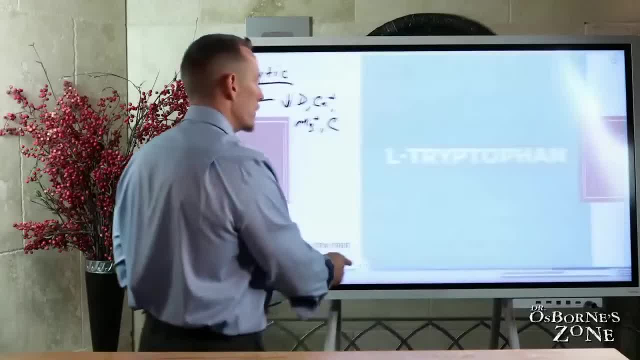 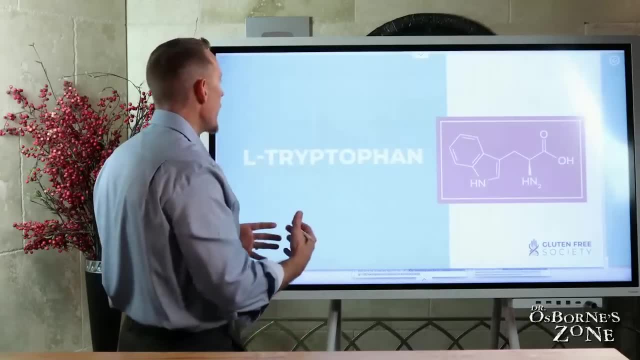 NAC is one you're definitely going to want to put in your home remedy arsenal. Now, next, let's talk about L-tryptophan. L-tryptophan is an amino acid as well, and its primary role it's got a few but one. 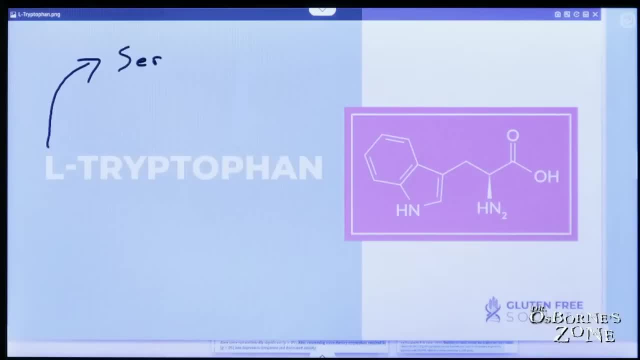 of its major roles is: it helps your body to produce serotonin. Might help if I Okay Spell that right for you. There we go. Serotonin is a neurotransmitter. that's predominant role. some people call it a happy neurotransmitter, so it plays a role in your demeanor. 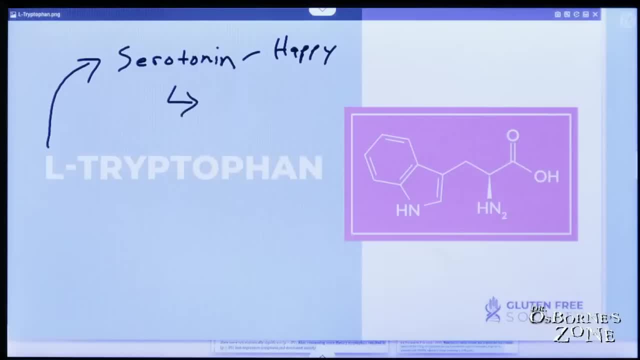 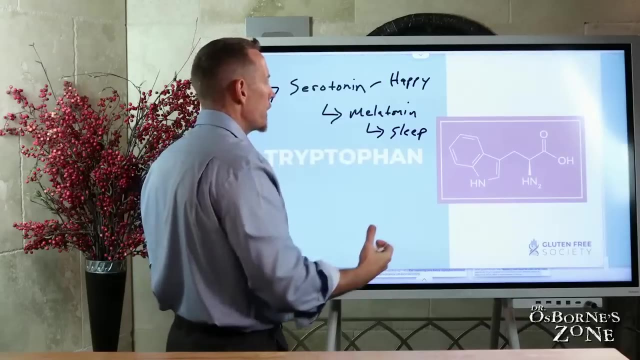 It's important, though, as well. from serotonin, we get something called melatonin, and of course, melatonin plays that primary role, That primary role in helping us fall asleep at night. and what happens when we have adequate melatonin and we go to bed at night? that melatonin shuts off the section of our brain. 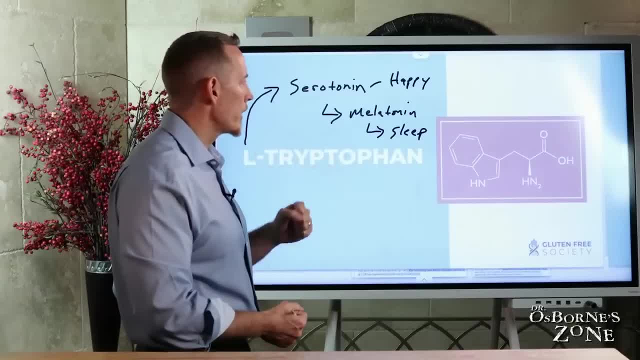 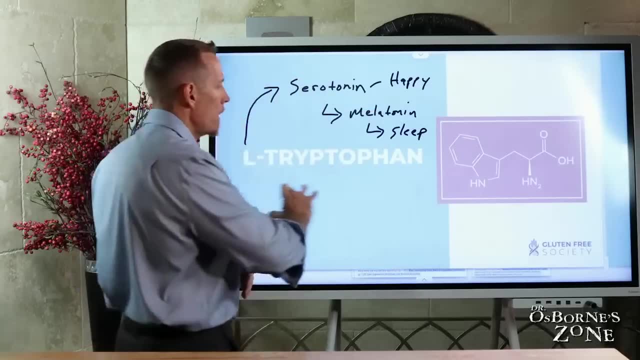 that produces cortisol, so that we can stay asleep and repair and recover and we can convert serotonin into melatonin. So, remember, tryptophan is a precursor to the body's ability to be able to do this, and so there are a number of studies that show that tryptophan is a precursor to the body's ability to be able to do this, And so there are a number of studies that show that tryptophan in the olden days was one of the sources of melatonin. fan taken, you know, between 500 and a thousand milligrams per day, can be an. 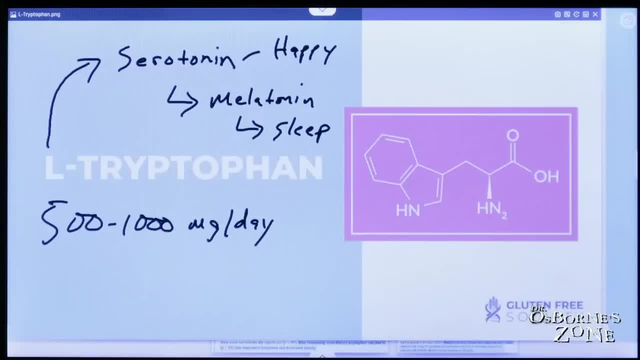 effective support for mood. there's some studies that show that there's a benefit for depression. those that suffer with depression- and if you think about, you know most antidepressants the doctors prescribed today. what are they? they are SSRIs- selective serotonin reuptake inhibitors- drugs like Paxil and Prozac. 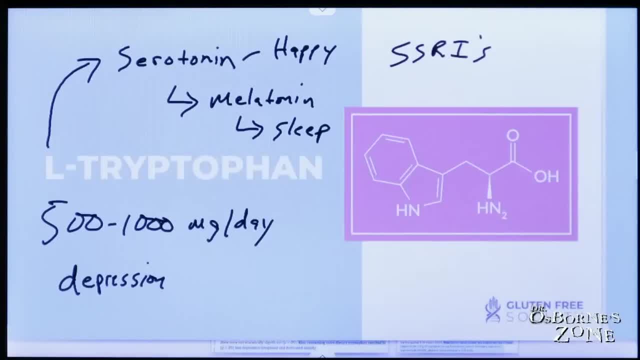 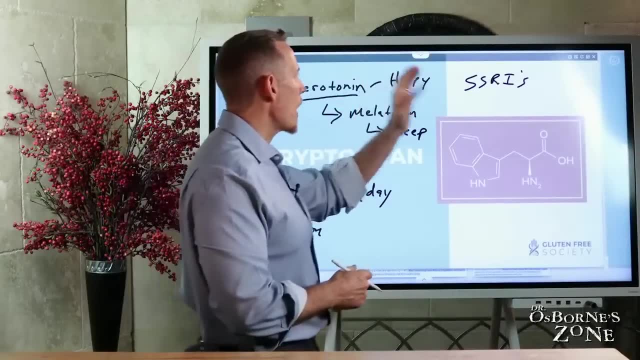 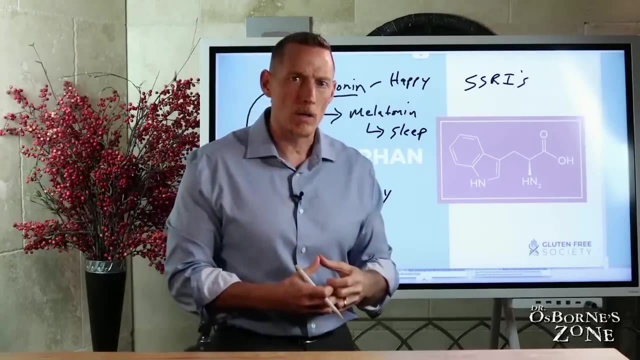 and these drugs are antidepressants right used in order to preserve serotonin. so so when we say selective serotonin reuptake inhibitor, these drugs stop the body from breaking down serotonin and recycling it, and so it keeps serotonin in the nerve cleft longer for the, so that the individual 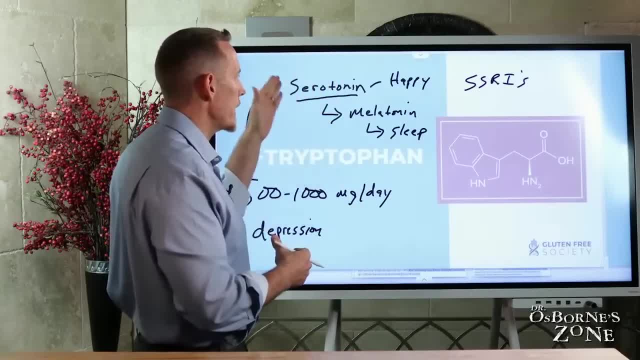 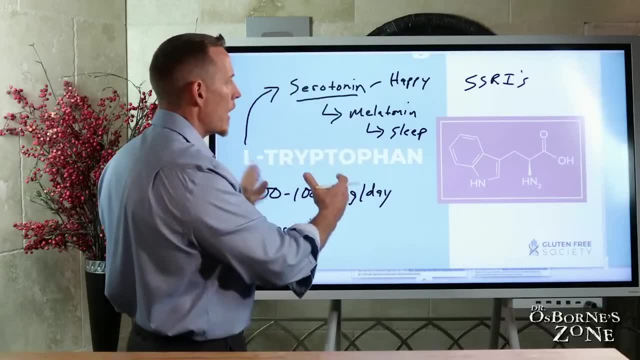 can get a look kind of a longer lasting amniotic fluid, and that's what we're talking about here. so we're talking about the impact or benefit of this area, the action of serotonin, and you know so if you're, if you're looking at tryptophan as an option, it's also important. 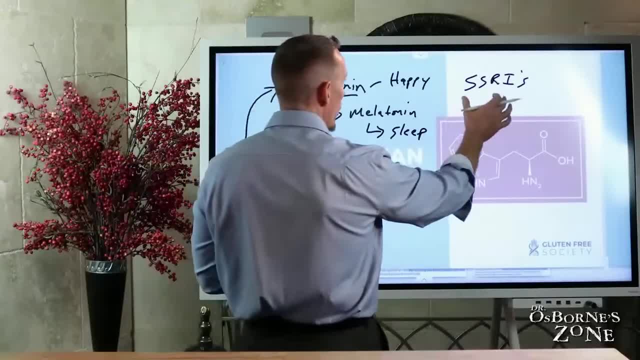 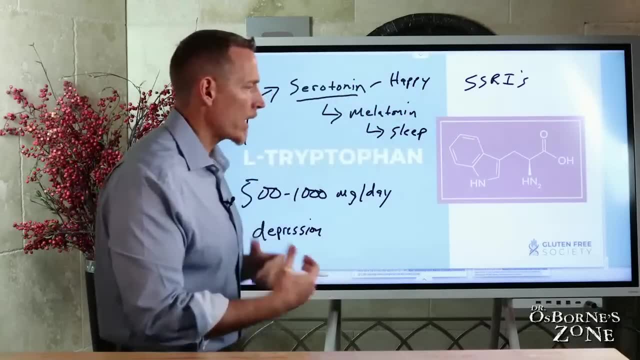 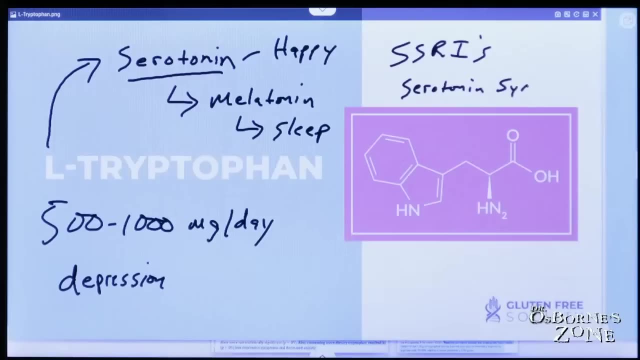 understand if you just start taking tryptophan and you're on one of these particular types of medications. tryptophan can enhance the functionality of an SSRI and there's actually something called serotonin syndrome which can make you sick. so you know, might be. it might be smart if you're on an SSRI and you're wanting to try to add some tryptophan again, tryptophan being a natural amino acid that you get- you can get from eating. you know protein predominantly, but you know you've all. probably the Thanksgiving thing, where people eat turkey at Thanksgiving and then they get tired, want to take a nap, and this is one of the reasons why is that there's a lot of l-tryptophan in turkey. other meats contain tryptophan as. 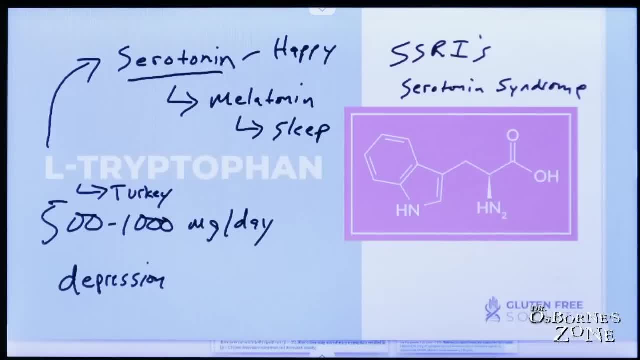 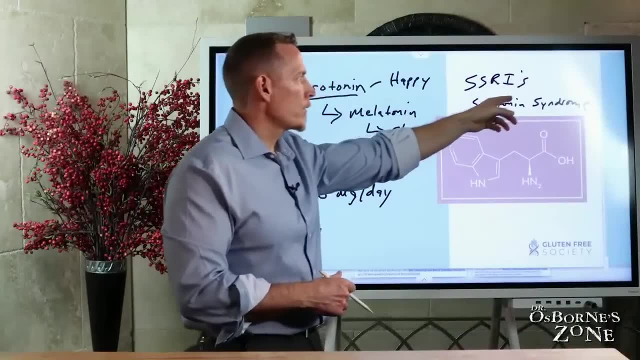 well, but, but turkey predominantly. one of the one of the biggest consequences of this is that it's a very high concentration of lipids. it's a very high concentration of lipids, and so you're gonna have to start taking tryptophan to maintain your concentration doses, naturally, but again. 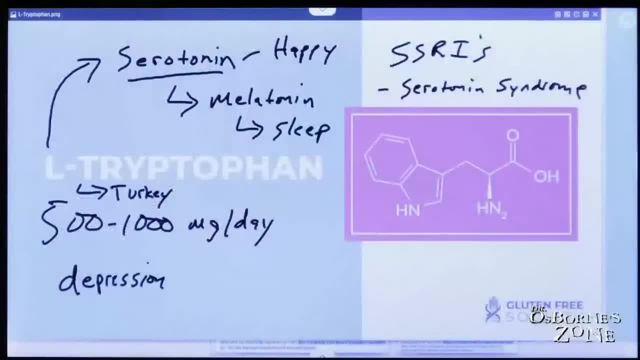 if you're taking tryptophan to try to support your brain, your anxiety or your depression, and you're on an SSRI as well, you got to be careful because the SSRI might start working too strongly and then you can end up with serotonin syndrome. so my advice there is: talk with your doctor. you know if you've got a good 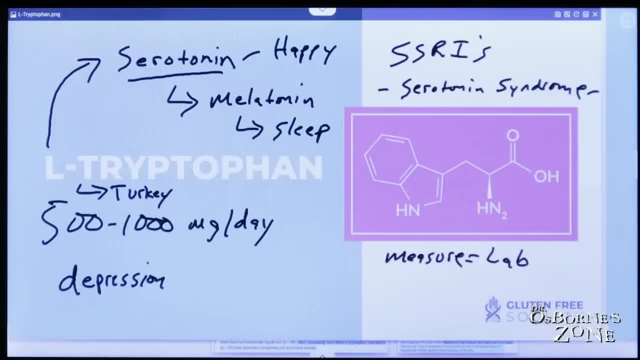 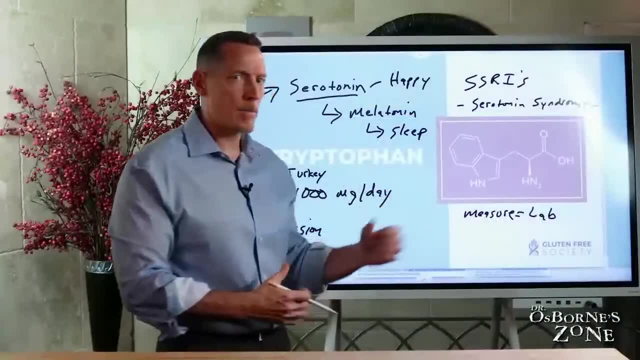 doctor, they can measure, make sure they're not going up too high and creating that. I've seen this a lot in my practice, where people come in and they're kind of playing with different amino acids- They've heard some of this information before and they're also taking SSRIs and we get 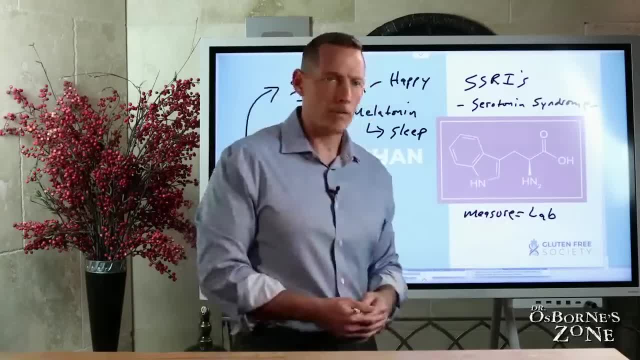 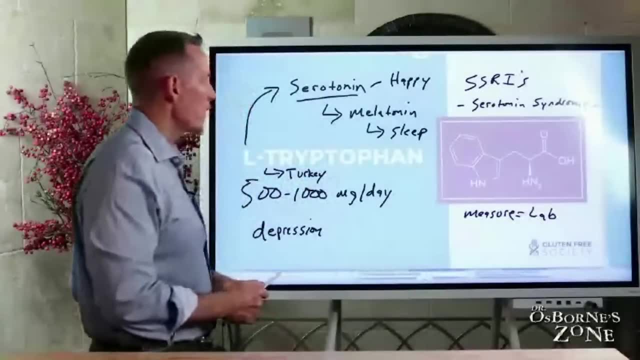 their serotonin labs back and they're off the chart and they're feeling terrible. It's because they've developed this issue. So you just want to be cautious that if you're going to start supplementing here with 5-HTP or with L-tryptophan, which is 5-HTP is 5-hydroxy. 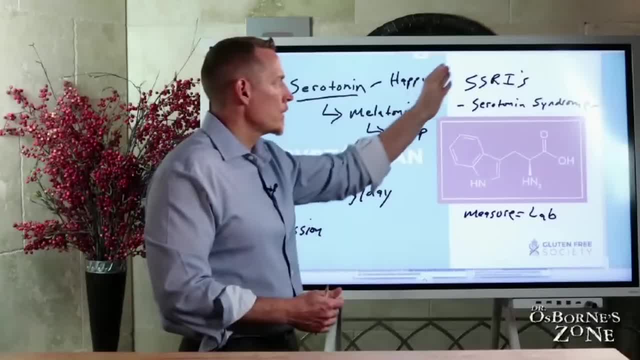 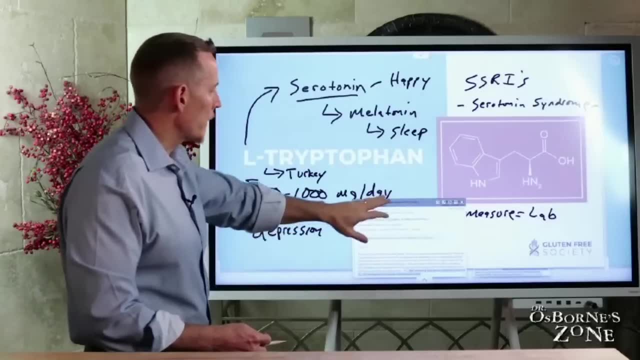 tryptophan. These two together a lot of people will use to help with serotonin. If you're on an SSRI, just be careful. Now there's some research I wanted to pull up here on this particular topic. You see the effects of dietary tryptophan on effective. 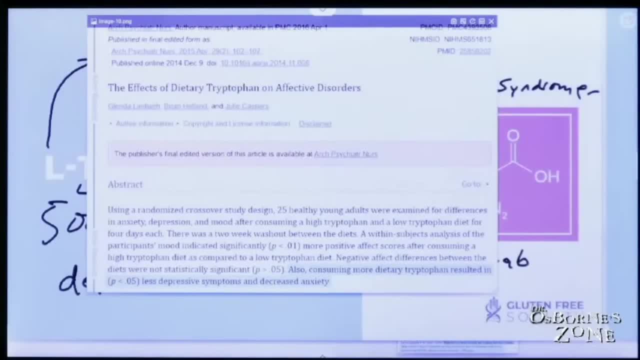 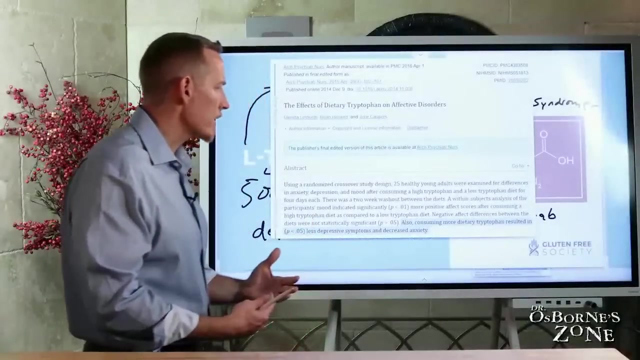 disorders, And so in this randomized crossover study, what they found is that those consuming more dietary tryptophan resulted in less depressive symptoms, as well as a decline in increased anxiety. So this small-scale study done on 25 young adults found that people that ate more tryptophan in their diet- basically that had an excess of, I think it. was 0.9 grams per day of tryptophan through their food choices, were less depressed and had less anxiety. So that's one very important aspect, just from food. Food is very powerful and sometimes people jump to supplements and forget the power of food. Don't forget. 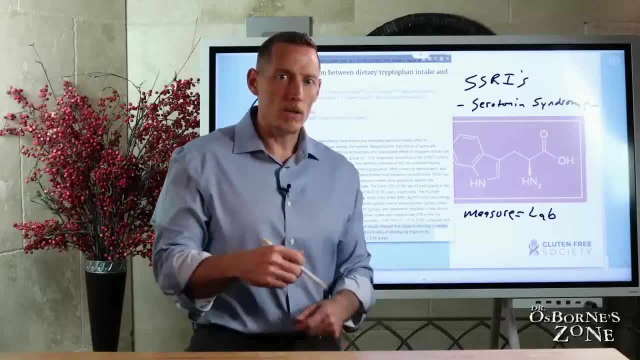 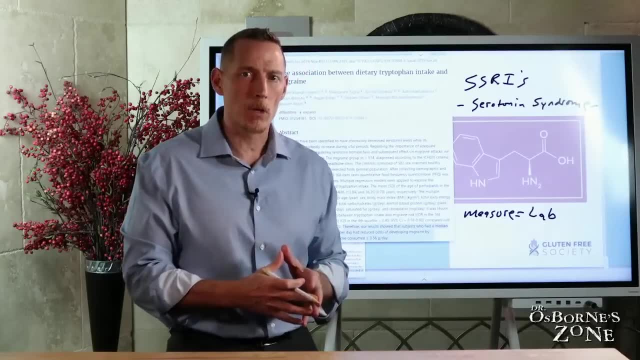 the power of food And this is why I mentioned earlier in the show all these people going plant-based having a really hard time getting some of these amino acids in high enough quantities in their day-to-day diet and they're suffering the repercussions of these deficiencies. And so again, here's another research study on the association between dietary tryptophan intake and migraine. And you see, here in this study our results showed that subjects who had a median intake of 0.84 to 1.6 grams of tryptophan per day had reduced odds of developing. 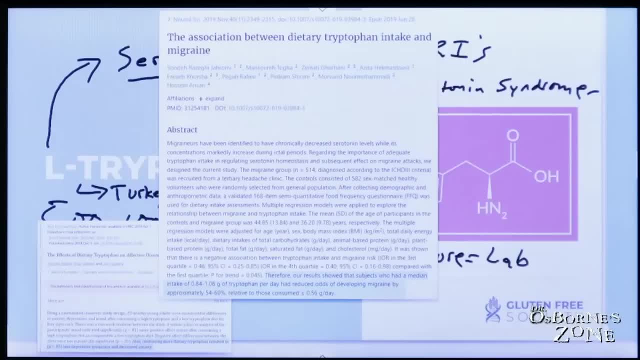 migraine by approximately 54 to 60 percent relative to those who consumed under a half a gram of tryptophan a day. So again, we're just talking about dietary consumption. We're not even talking here about the potential for supplementation. Now again, with all these, 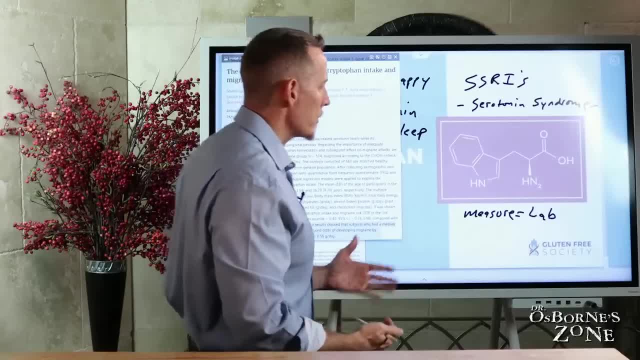 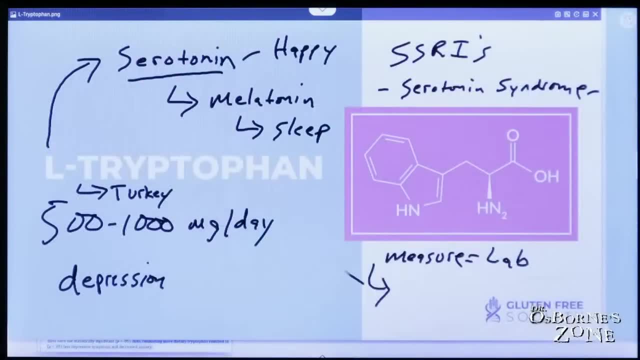 amino acids that we're going to talk about today. you can measure them all. I mean, aside from just measuring serotonin. you can measure serotonin, but you can also measure directly. you can measure tryptophan. So this may be one of those things if you're considering using some of these therapeutic. 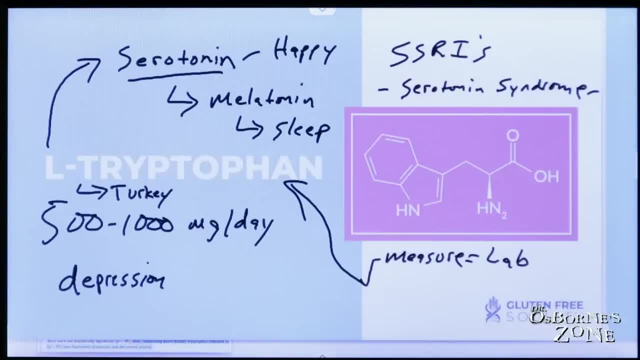 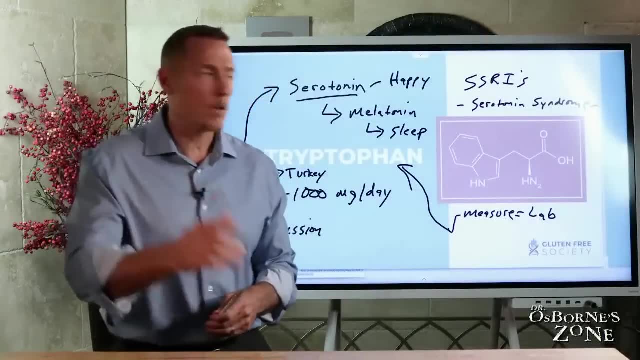 amino acids. you might just consider having your amino acid levels checked And again get with your doctor. If your doctor can order them for you, great. If your doctor won't order them for you, you might consider using some of our online testing services, where. 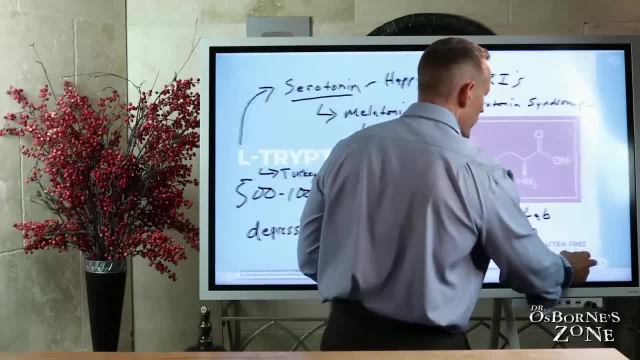 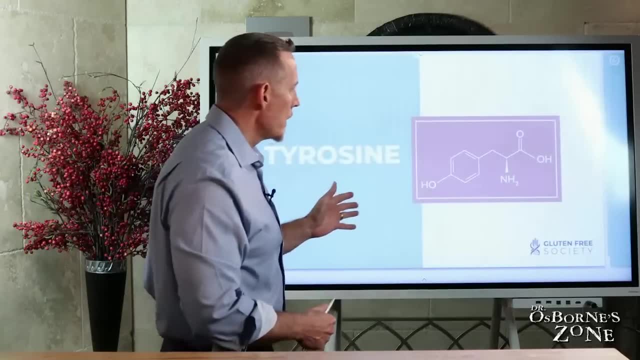 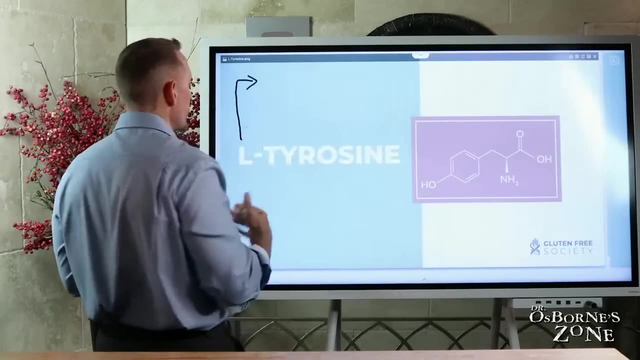 we do a lot of this deeper dive on vitamins, minerals and amino acids. Okay, let's next talk about L-tyrosine. Now, L-tyrosine is a super important amino acid. It produces, or it's a precursor to, the catecholamines. 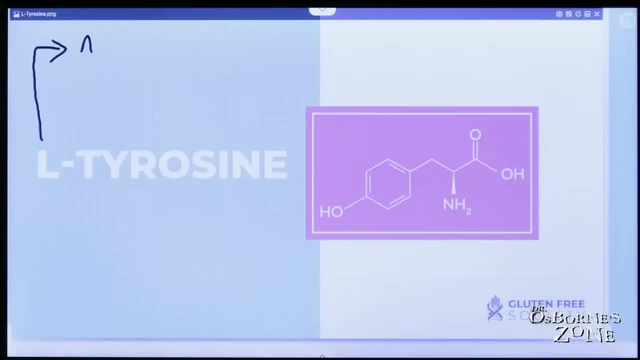 So catecholamines being adrenaline as well as noradrenaline- Some people call it epinephrine and norepinephrine- but also dopamine. So these are, you know, extremely important amino acids. Now we're going to talk a little bit more about dopamine. 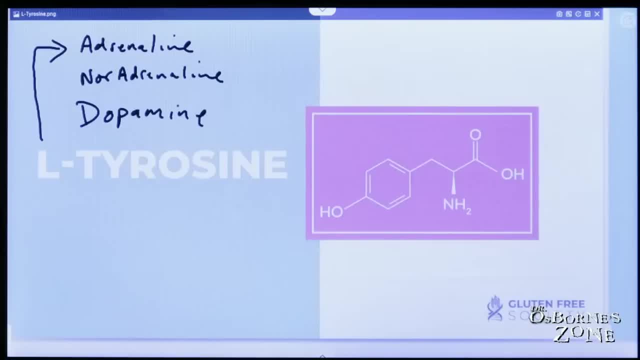 Now we're going to talk a little bit more about dopamine. We're going to talk a little bit more about dopamine. We're going to talk a little bit more about dopamine. These are important neurotransmitters. We look at the catecholamines here, We these. 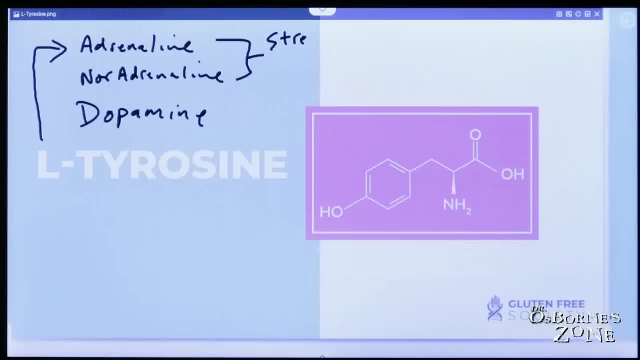 these are, you know, important for your ability to tolerate and handle stress. They're in, you know so. so again, when we're stressed out, we make more adrenaline to help us cope and adapt to that stress. Adrenaline gives energy. Adrenaline helps with brain clarity. So very important that. 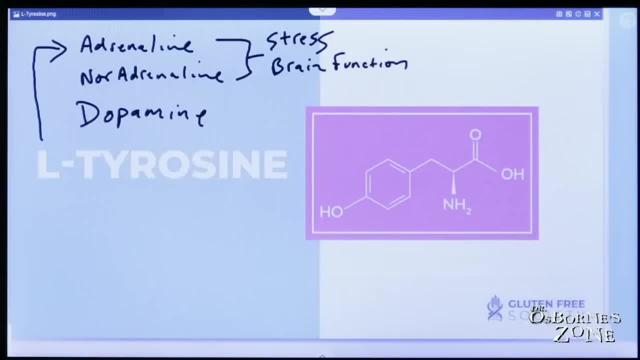 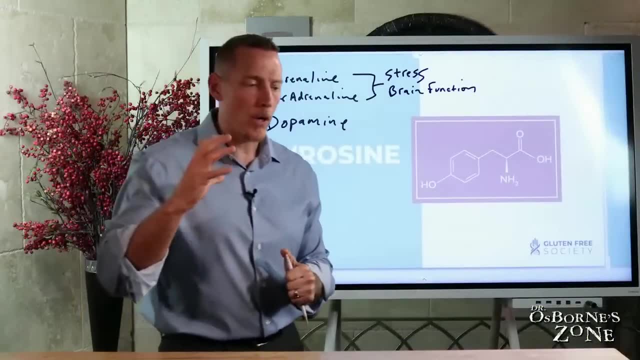 you get adequate tyrosine in your diet to support, especially when you're under more stress, and this is what, a lot of times, what we'll see when people- this is especially true of women, by the way- that when they're under tremendous periods of stress, their brain fog is one of the 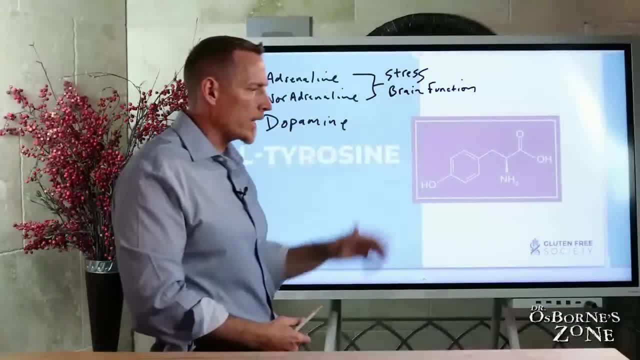 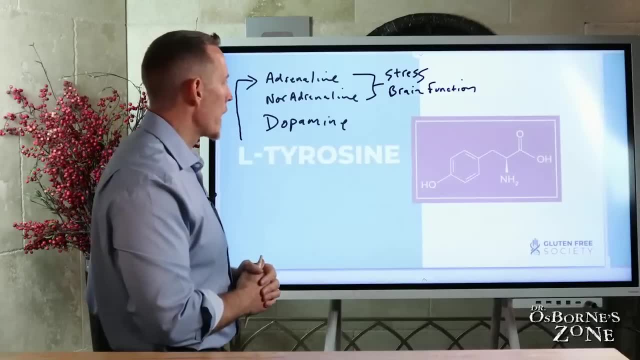 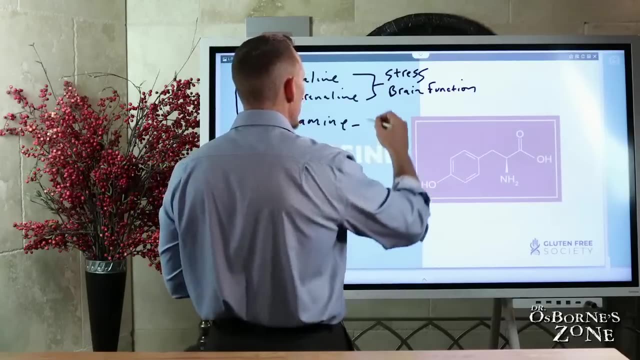 major issues. that happens. They end up with a lot of anxiety, and this can be as a result of the deficiency of the ability to produce adrenaline and noradrenaline, And also, as well, dopamine. Dopamine deficiency can cause those symptoms as well. Dopamine also plays a role in motor. 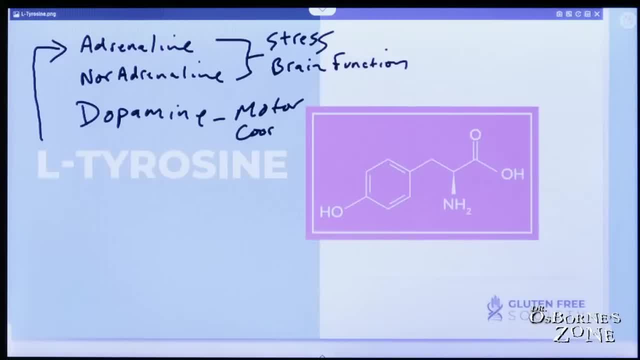 coordination. So that's muscles, how your muscles move and how well they're coordinated, We'll see. sometimes people develop tremors. If you've heard of Parkinson's disease, for example, it's a disease where dopamine production is diminished as a result of inflammatory 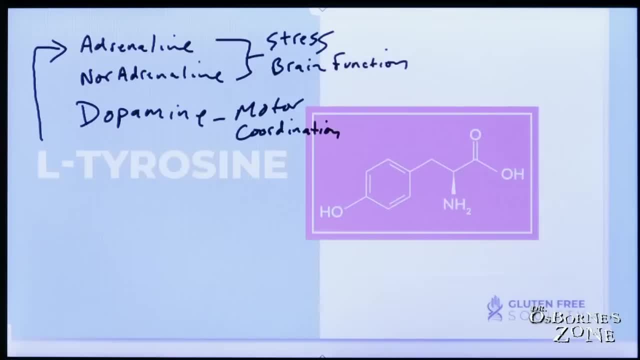 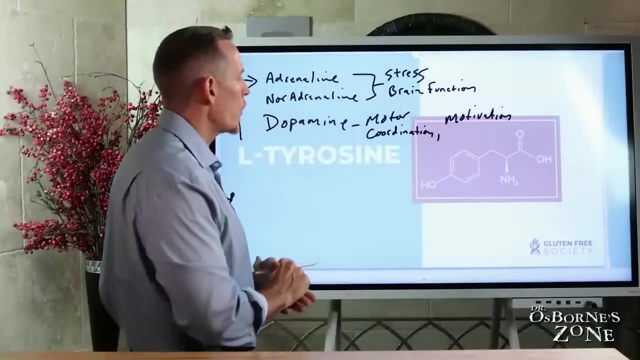 damage in the nervous system. So muscle-motor coordination, but also motivation. So dopamine very, very important. So dopamine deficiencies can lead to depression, apathy, lack of motivation, lack of desire, drive to want to do much, And so again, you can't make. 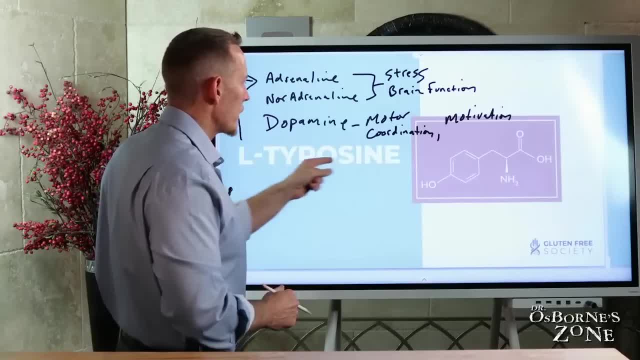 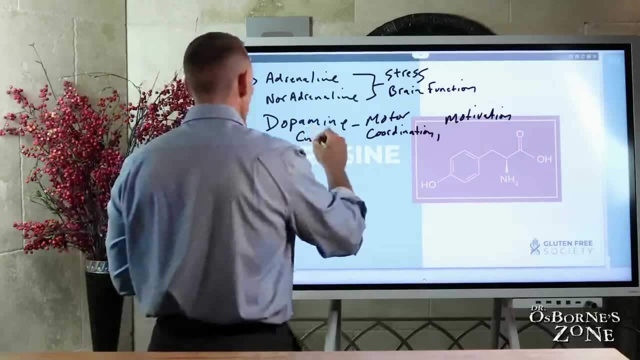 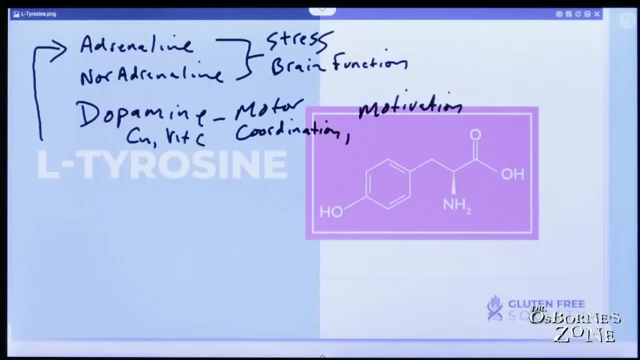 these three neurochemicals without tyrosine. Tyrosine is the backbone of these chemicals. Also, you need things like copper and vitamin C to take tyrosine through this pathway, But again, L-tyrosine very important in that regard. Now L-tyrosine is also extremely important. 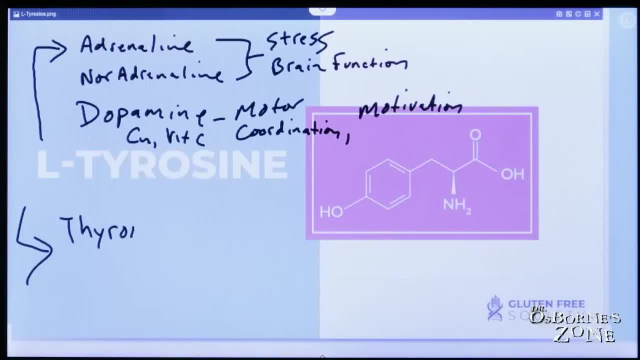 to produce thyroid hormone. As a matter of fact, the T and T4, so T4 is kind of an abbreviation. If you've ever had your lab tests done, your thyroid test done, T4 is thyroid hormone, right, So T4. 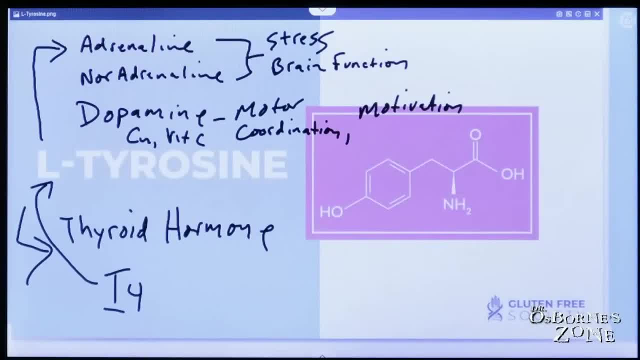 The T is tyrosine. And then T4 has to be converted into T3, which is the active form of thyroid hormone. Same thing here: The T is tyrosine. By the way, the 4 and the 3 represent. 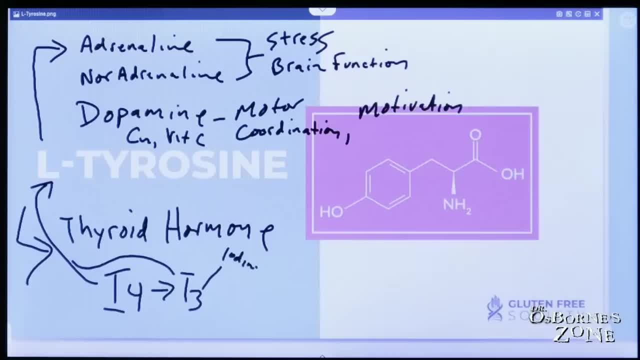 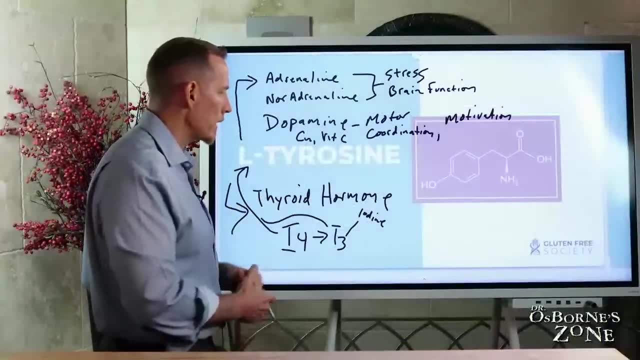 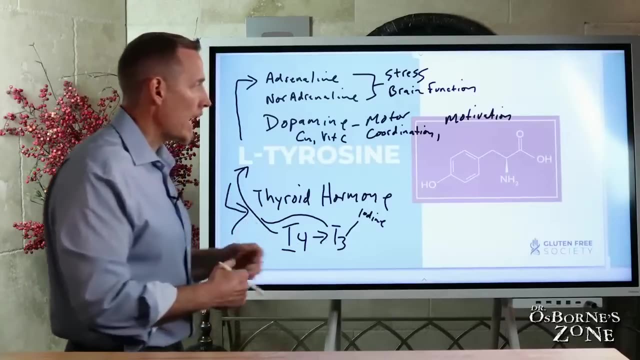 iodine, Those of you who are interested. iodine also an important nutrient that plays a role in thyroid hormone production, But lack of tyrosine will reduce your body's capacity to make thyroid hormone, Now super important If you're using tyrosine supplementally, if you plan on taking it and you're on thyroid. 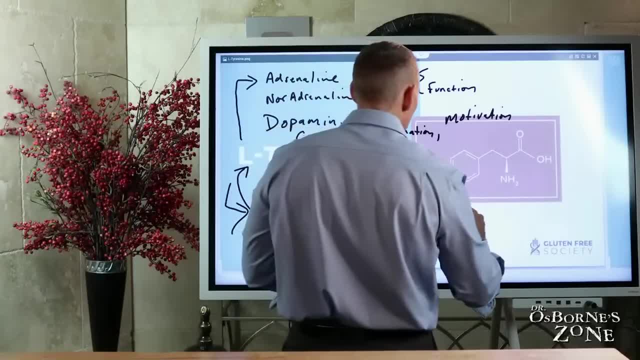 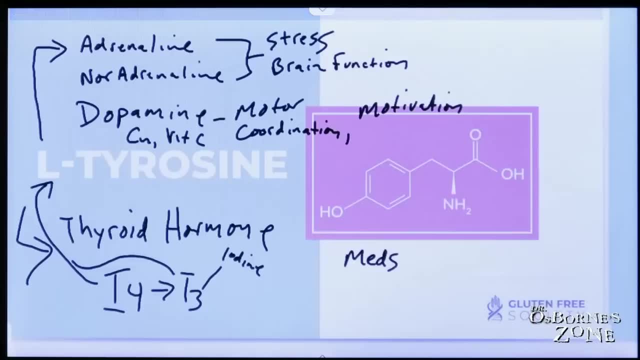 medication. So if you're on thyroid medication- maybe you've got a hypothyroid diagnosis- Hashimoto's- and you're on meds and you're going to start taking tyrosine- one of the things that can happen is it can increase your T4 and your T3. And, in effect, your medicine will work better. In some cases I would say: is it your medicine working better, or is it just nature helping you do what your body already knows how to do? Either way, you don't want to end up in a state where your thyroid hormone is now too strong. it's too high. This can create heart problems. 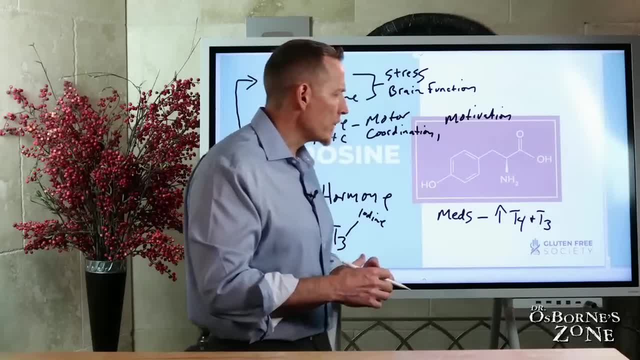 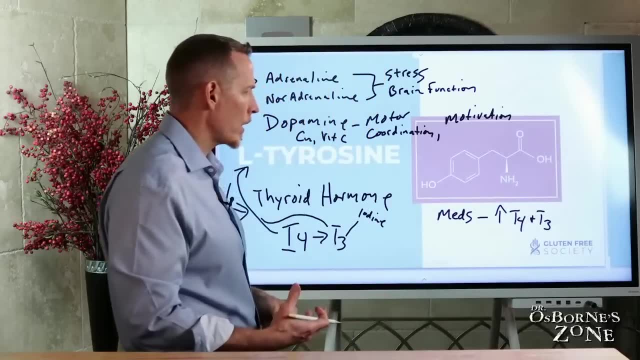 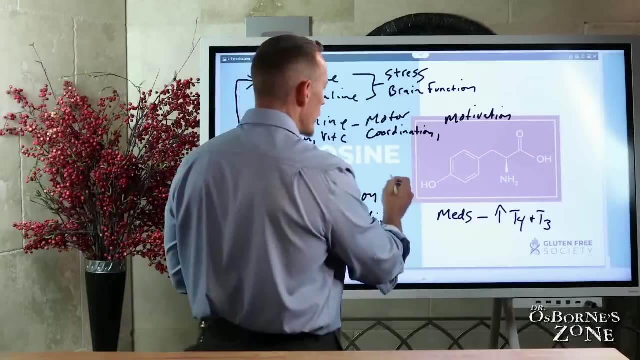 heart palpitations, night flashes, hot sweats, different types of symptoms associated when your thyroid medicine goes up or your thyroid hormone levels go up as a result of combining these two. So, again, if you're thinking about using this and you're taking the medicine, it's good to have a conversation with 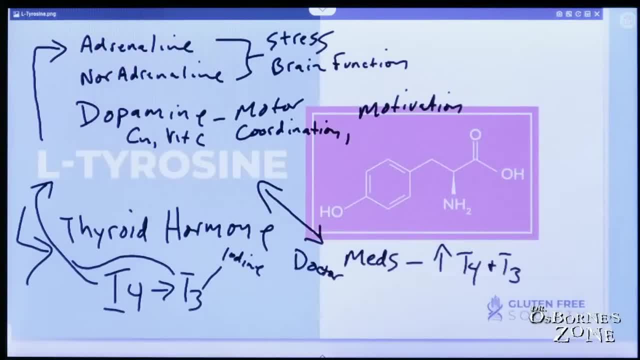 your doctor monitor Again. you can measure tyrosine before you even get started. but you can also monitor your TSH, your T3,, your T4, what I call, or what is called your reverse T3, and see. 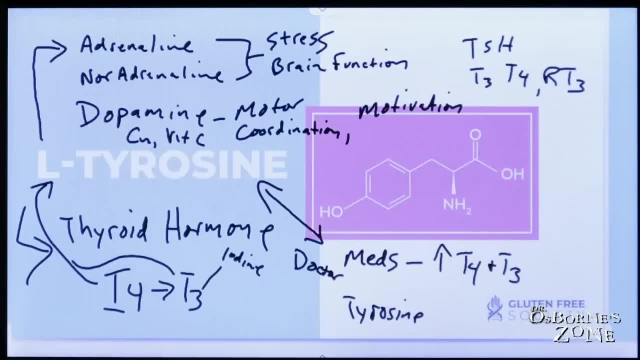 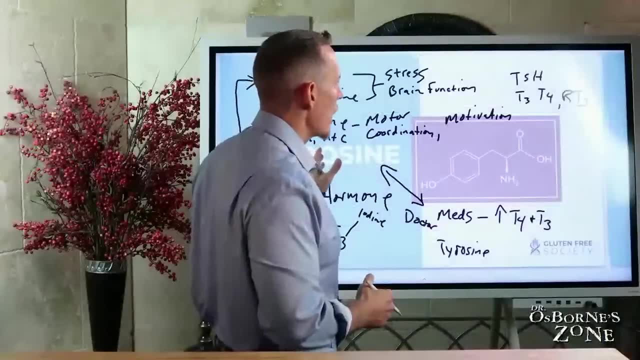 what's happening with these numbers as you start this? Because, again, this is just like I was talking about a moment ago with tryptophan and serotonin. It's that taking a lot of this can lead to more of this, which can make. 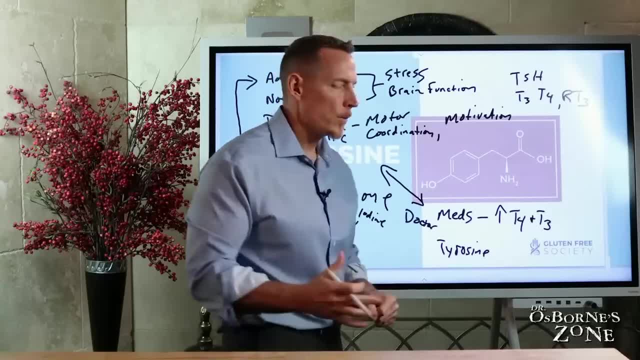 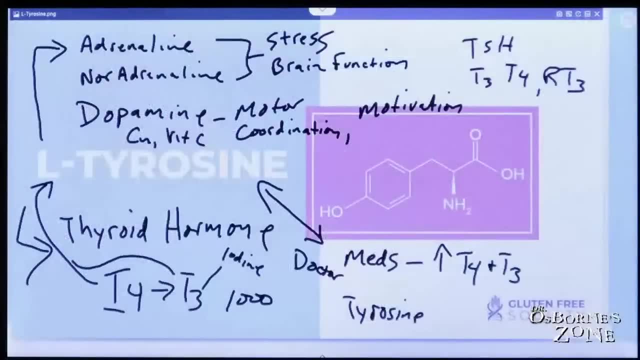 potentially for a toxic situation. So you just want to make sure, when you add this in you're monitoring. And as far as dosing is concerned, with tyrosine, a thousand to 1500 milligrams a day is a good. 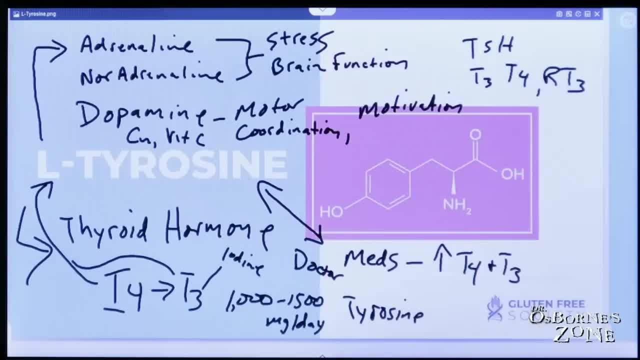 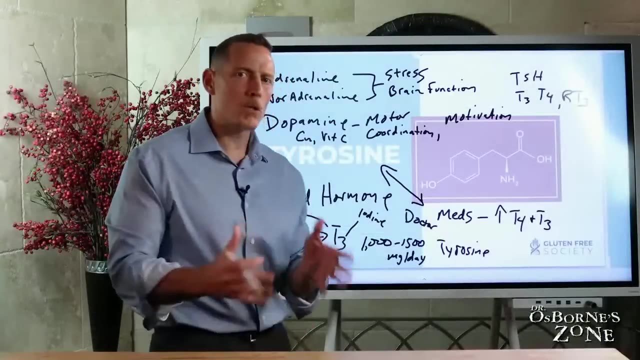 place to start for an adult Um Again. but if you're going to do that testing something, I would highly encourage you to do So. very simple, to get L-tyrosine over the. you can get it over the counter. I mean, it comes as a free form amino acid And, of course, 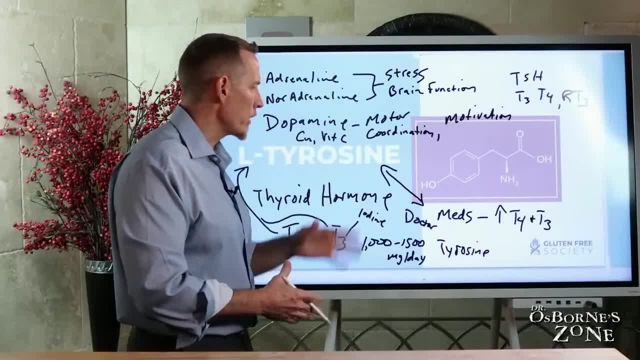 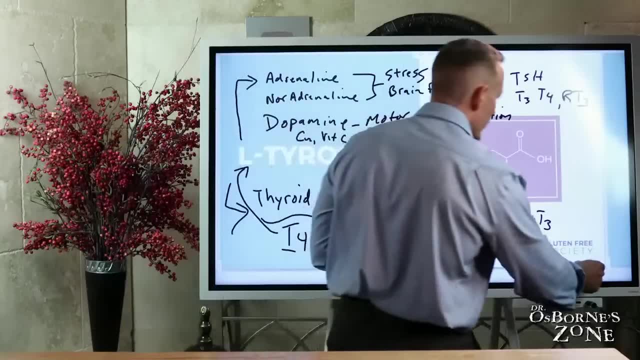 you can also make sure that you're eating enough ample quantities in food, and where you're going to get the bulk of your tyrosine from your diet is going to be in animal meats, And so, again, vegetarians if you're avoiding all animal foods, animal byproducts, definitely I would encourage. 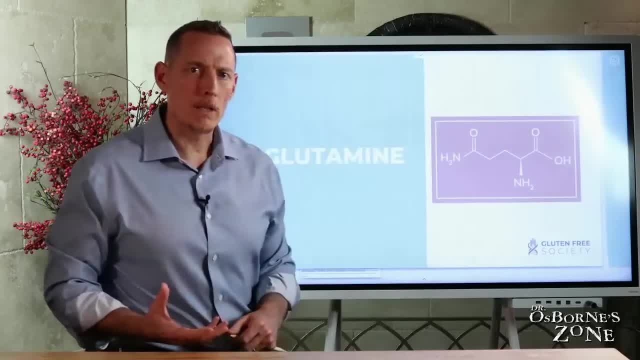 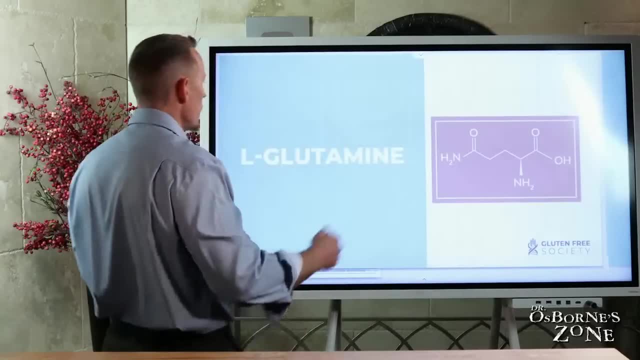 you to check your levels to make sure that you're not becoming depleted as time goes on. Okay, let's talk about L-glutamine. L-glutamine is an amino acid We were talking about earlier. we're talking about cysteine, or NAC, inositol cysteine. Well, glutamine is also part of what 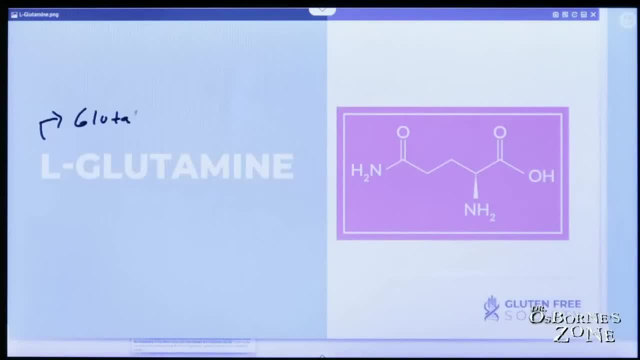 helps to produce glutathione. So I say glutathione earlier was NAC was one of the most important ingredients to go into producing that, But glutamine is also one of those important ingredients. So you need glutamine to make glutathione. Now glutamine is also very, very important as a fuel for immune cells. 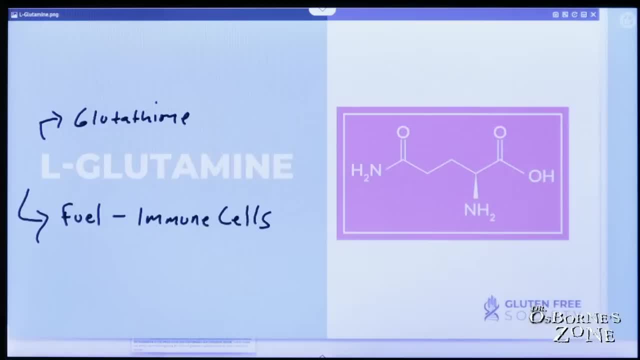 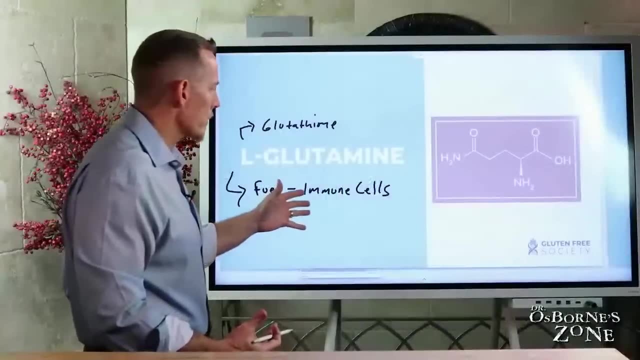 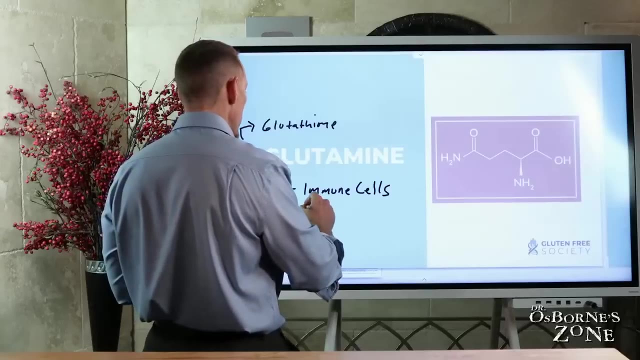 You know, most of the cells in our body require glucose as a fuel source to drive and generate enough energy to do their functions Well. your immune cells can use glutamine as a primary fuel source. Now, what's also interesting here is that so can 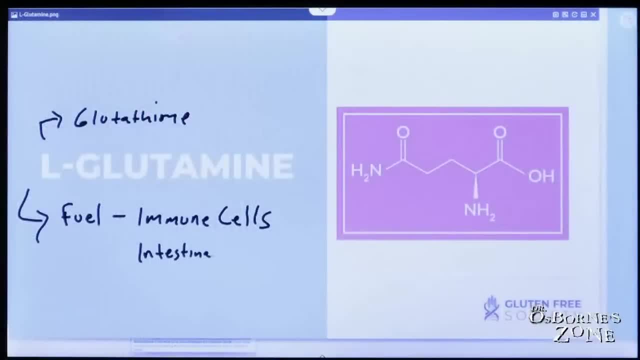 the cells of your small intestine. So your intestinal cells also use glutamine as a fuel source. We see this a lot. where people have immune problems, where their white blood cell counts are low- they're not producing adequate quantities- We use L-glutamine. boom- white counts start to. 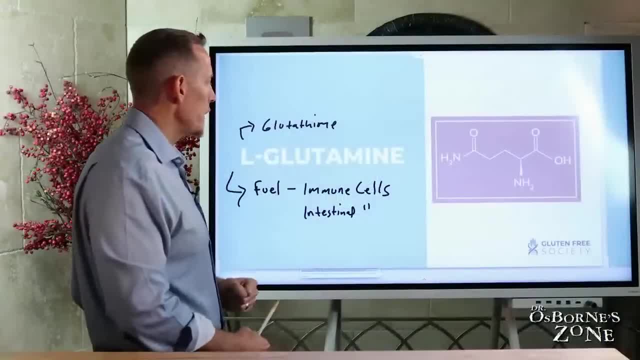 climb, they can start to go back up. It's because, again, glutamine can be used as a fuel source in the immune cells. Now, a lot of people- there's a lot of folks- that are using L-glutamine. 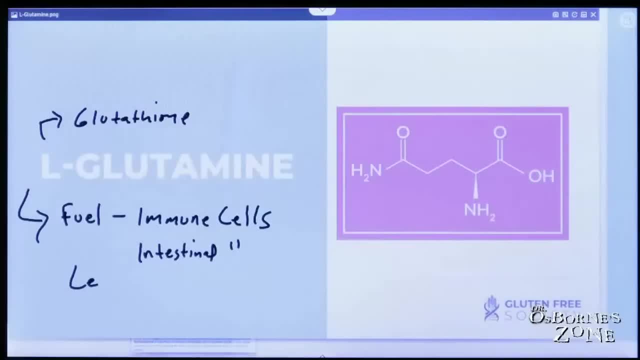 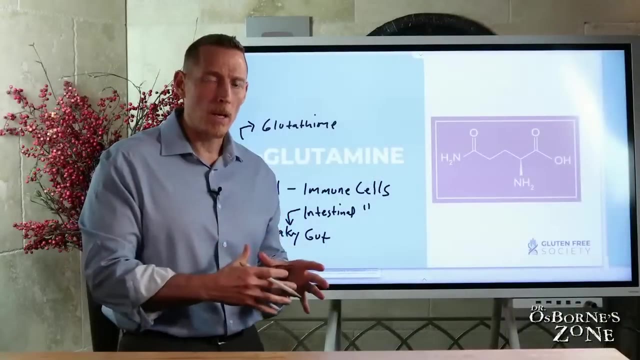 just talking about using L-glutamine for leaky gut, And this is the reason why The intestine cells, okay, need L-glutamine to generate or drive their energy production, And so if they don't have enough energy through glutamine, then those cells remember they have to turn over. they have 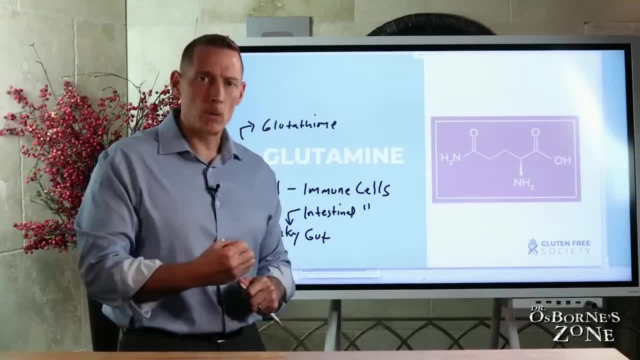 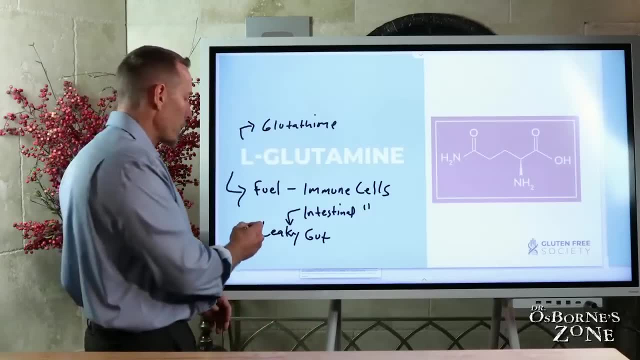 to recycle every two to seven days. If they don't have the fuel source they need, those cells get old. they become less effective at doing their work. We can get a breach of the intestinal barrier, so leaky gut can set in, And there are a number. 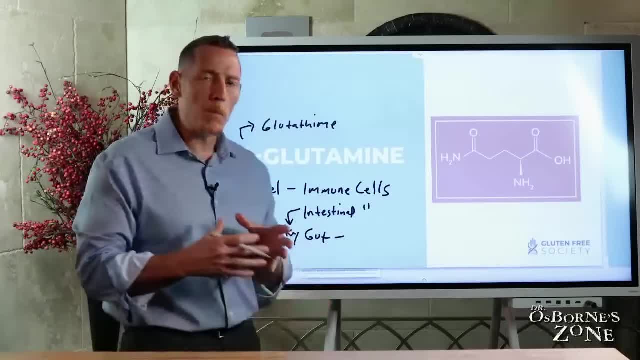 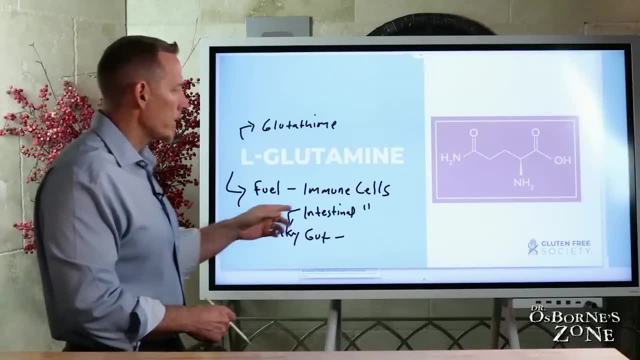 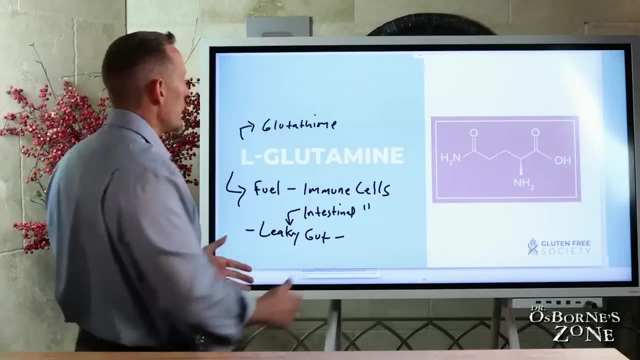 of research studies looking at L-glutamine with the barrier of the GI tract and looking at it for this very reason. So again, L-glutamine: very, very critical for the intestinal fuel, but also for immune cell fuel. Now one of my favorite ways to use L-glutamine is in 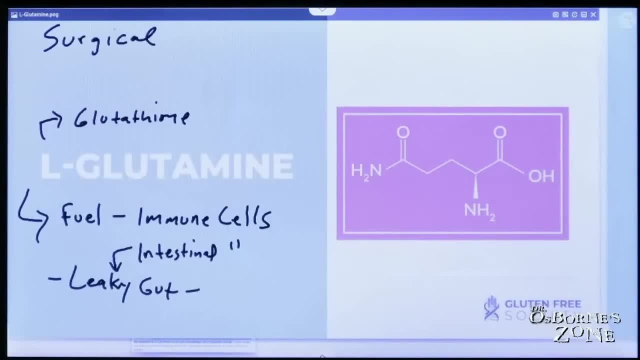 surgical Trauma. it's like a fracture, broken bone, but also in workout recovery. So if you've ever had a surgery, especially a major surgery like a hip replacement, where they have to cut deep and there's a lot of blood loss, there's a lot of potential for. 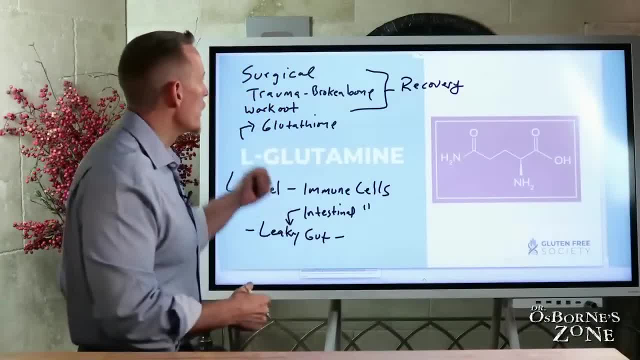 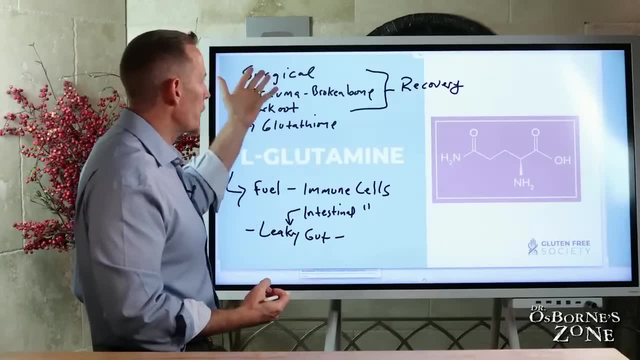 damage during the surgery. spinal surgeries can be the same way Your body needs to recover and repair. that you know. surgery is basically scheduled trauma, right, So it's a form of purposeful trauma, just like a broken bone requires a lot of nutrients. 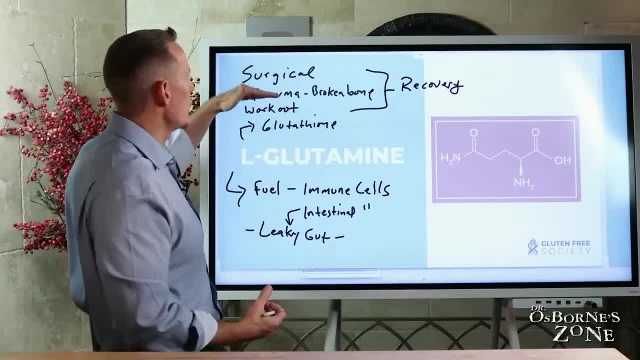 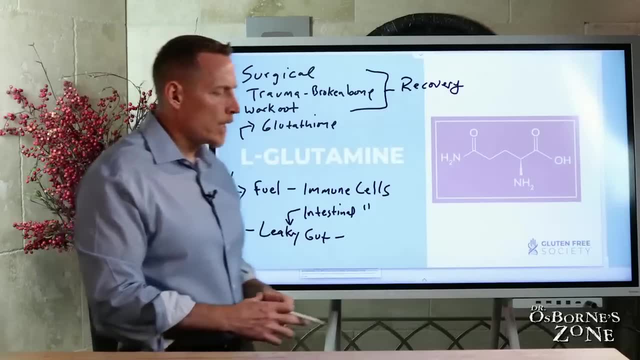 to heal and re-knit and repair that bone. So these two kind of we look at as the same for recovery, L-glutamine supplementation can be very, very powerful. As a matter of fact, I used to run a rehab clinic for a number of years. 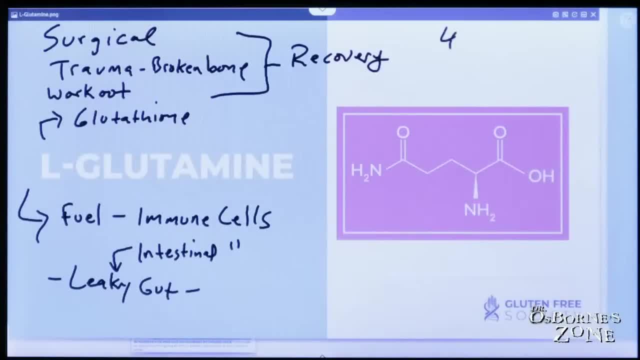 We would use L-glutamine. we'd use anywhere from four to five grams, in some cases a day, of L-glutamine supplement to help patients recover, And you know generally what we saw and we did comparatives. we saw people that would. do this would heal in the order of you know, anywhere from one and a half to three times faster, And people who would not do it, So it's very, very- can be very, very helpful if you've had trauma or if you've had surgery. 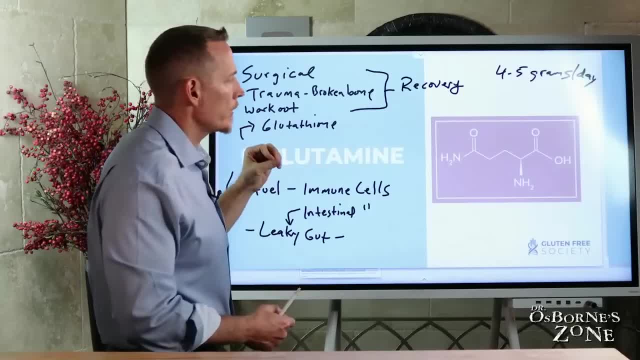 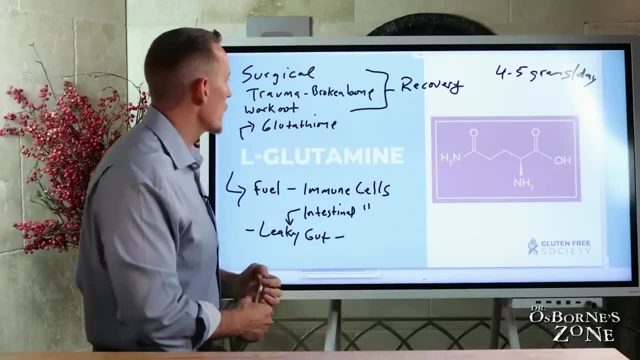 It's also very helpful for those of you who work out very aggressively and you're trying to find a way to reduce your muscle soreness, to improve your or reduce your downtime in terms of that muscle recovery. L-glutamine, even at the same dose, and you know there's some studies that show that- doses upwards of 30 grams a day are perfectly safe over long durations, although I would say be cautious With L-glutamine because you get the dose too high. some people get headaches, Some people have diarrhea. So you know this is relatively a safe range for most. 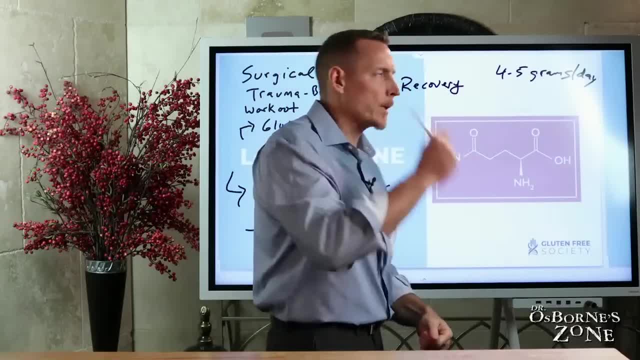 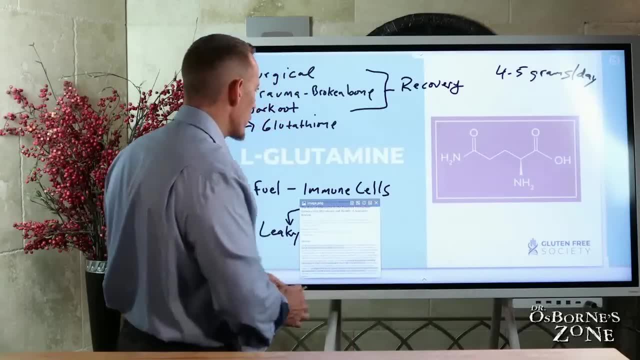 But if you're going to go higher than that, just be cautious and kind of slowly, incrementally, try to increase it And if you start getting symptoms you know to back off. But again, L-glutamine can be very helpful in this regard. 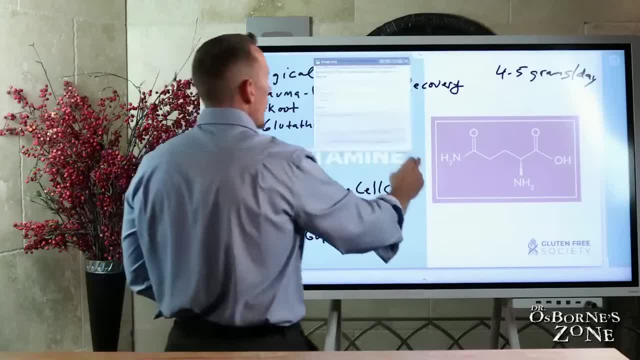 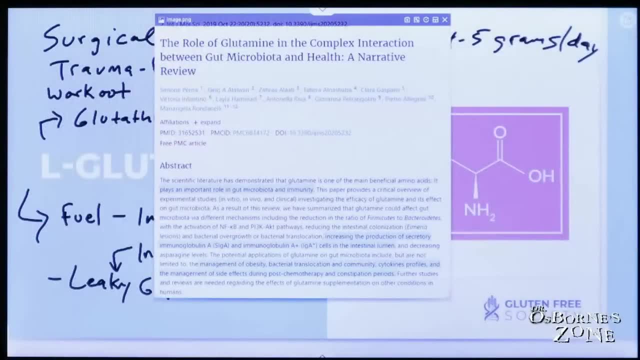 Now one of the things I want to point out. this is a great study just published a few years ago. It was a study on glutamine, the role of glutamine in the complex interaction between gut microbiota and health. So in this review- again the summary here- glutamine plays an important role in gut microbiota. 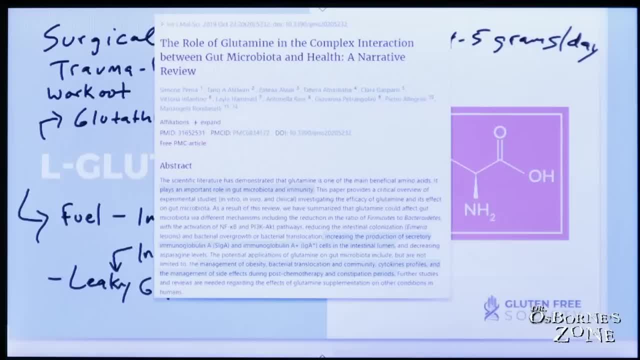 and immunity, increasing the production. One of its functions is it increases the production of something called sigatory immunoglobulin A or Sig A. So those of you that don't know what Sig A is, Sig A is anit's a protein. 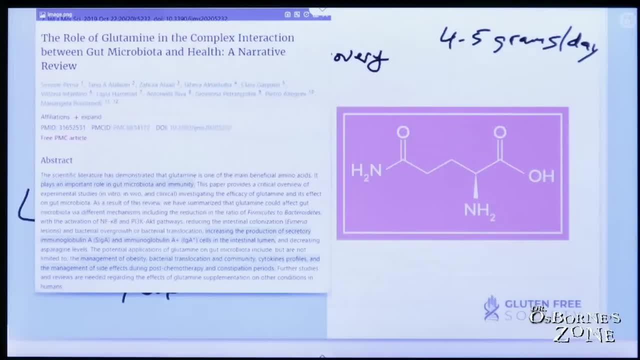 It's a protein, It's an antibody that you produce in your mouth. You produce it in your GI tract, It's produced in your lungs And what itit acts like a handcuff. So it's a general, non-specific antibody. 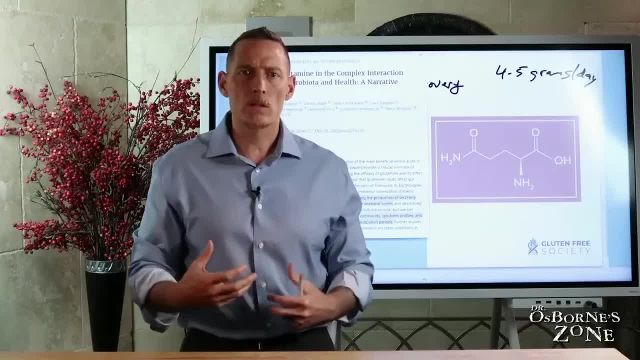 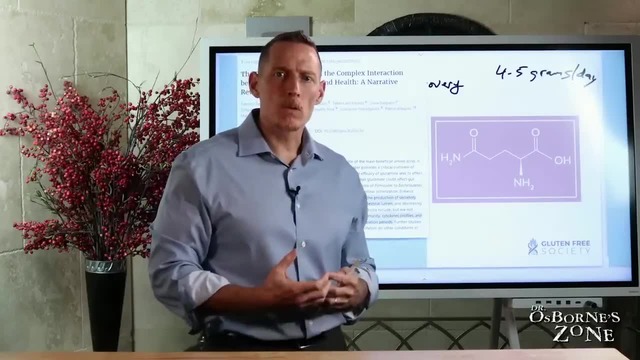 You know, every time we eat, every time we breathe, there's chemicals and toxins in the food we eat, in the air we breathe. Well, the job of IgA is to bind those chemicals, those toxins, so that we can neutralize them. 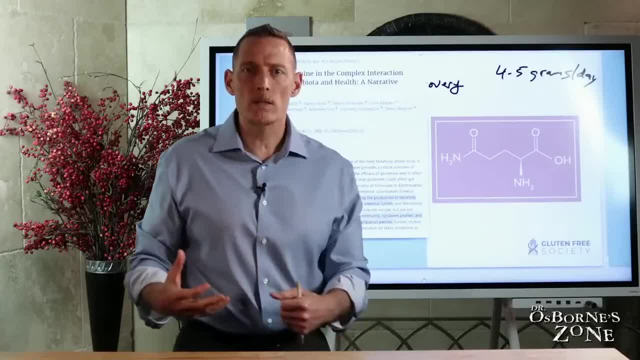 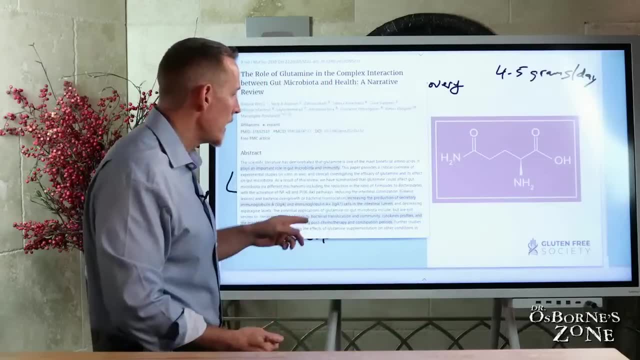 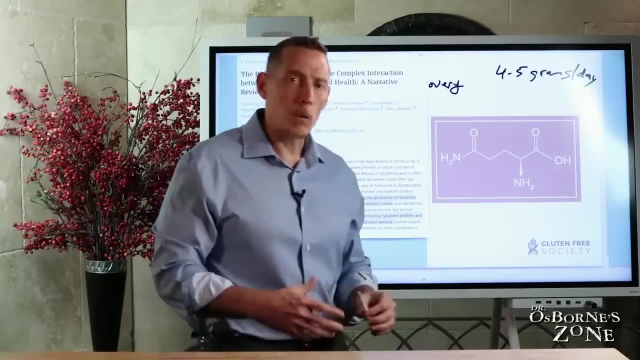 Like a handcuff neutralizes a bad guy. If a police officer is arresting somebody, puts them in cuffs so he doesn't have to fight them the entire way to the police station. well, your immune system uses IgA- sigatory IgA- as a handcuff of sorts to neutralize potential dangerous toxins and prepare them. for excretion or expulsion out of the body. So you need glutamine to properly produce IgA, sigatory IgA, as well as just pure immunoglobulin A, And you see, in this case they're talking about in the intestine. 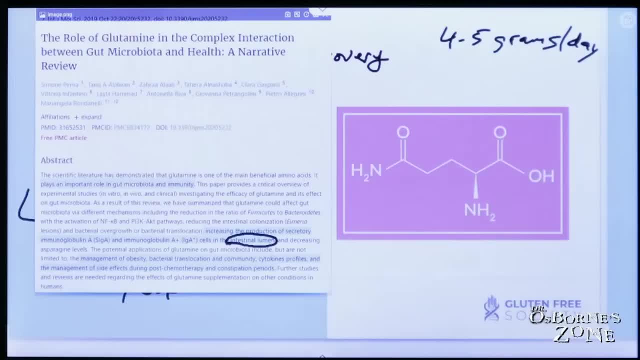 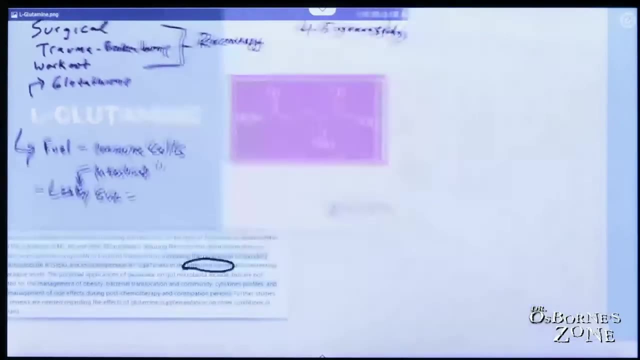 In the intestinal lumen, which again in the GI tract, Also in the management of obesity, bacterial translocation and community. So one of the things that can happen in a gut: if the gut's leaking, let's make some room and let's draw up. 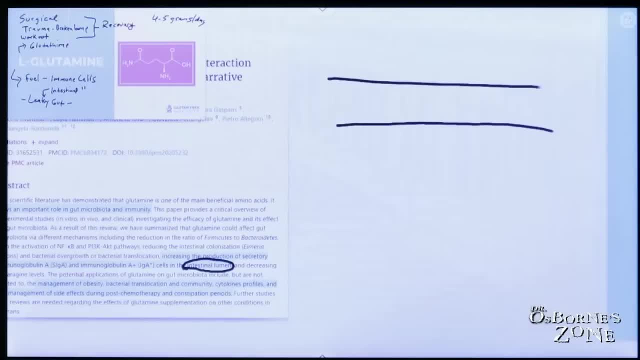 We look at, kind of generally, the gut. it's like a tube And it's lined with. It's lined with cells And if we have a gap in between these cells, that's what we call leaky right, Leaky gut or intestinal hyperpermeability. 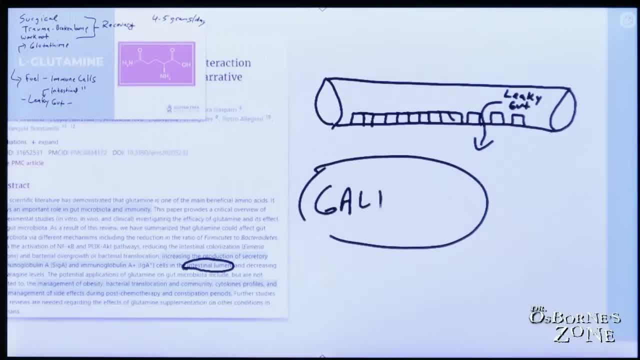 Now, behind the gut wall, you have this massive conglomeration of immune tissue called the gastro-associated lymphoid tissue. Inside the gut you have all kinds of particulate bacteria, bacterial toxins, But there's one kind of toxin called LPS, lipopolysaccharide. 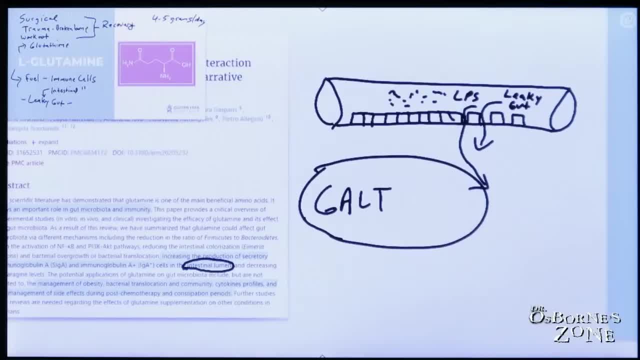 When it permeates through, it will stimulate the GALT, but it will also traverse to your liver through the portal circulation and it can damage the liver, increasing the risk for the development of what's known as non-alcoholic fatty liver disease. 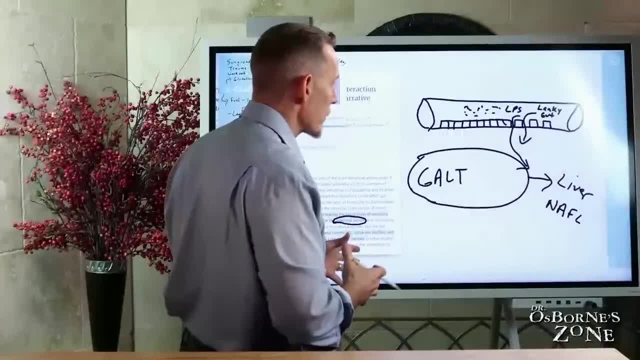 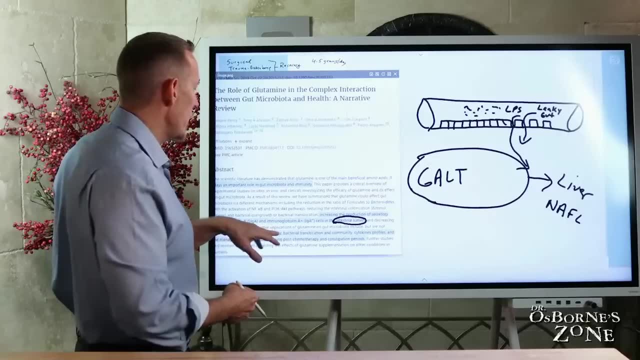 This is one of the ways that we can actually get fat stored in the liver. we can get preserosis to the liver, just damage to the liver cells in general. So what this is talking about here in this study is bacterial translocation would refer. 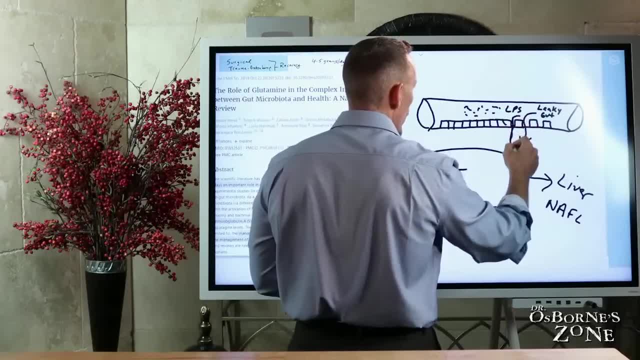 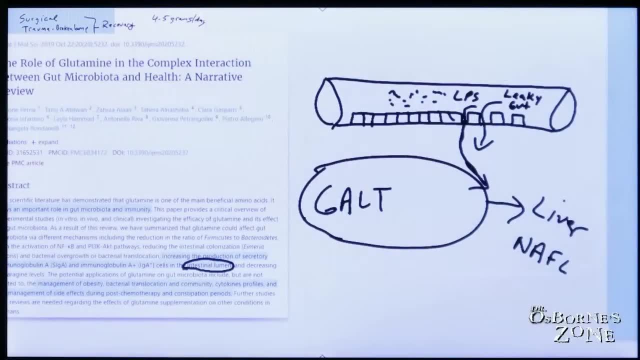 to bacteria crossing or translocating right Coming from the gut lumen into the GALT and then subsequently on into the bloodstream through the liver, but also the toxins that the bacteria produces. So we could get LPS in there. We could get LPS in there. 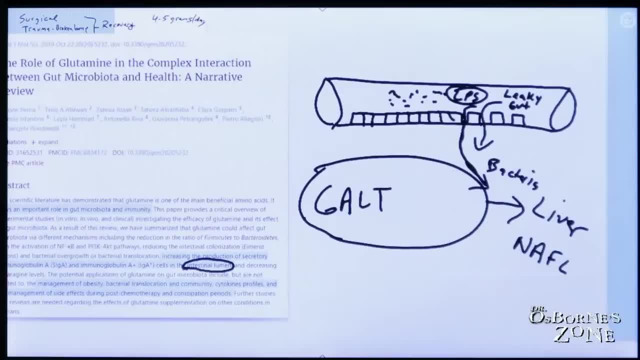 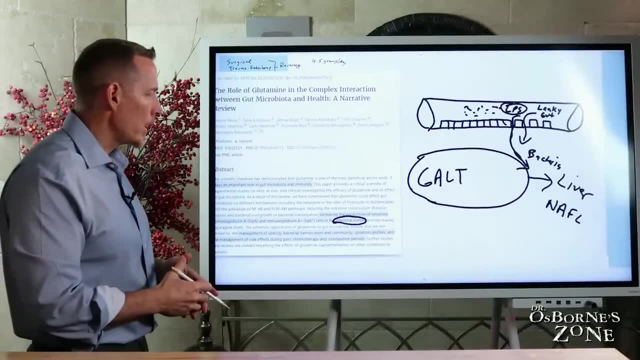 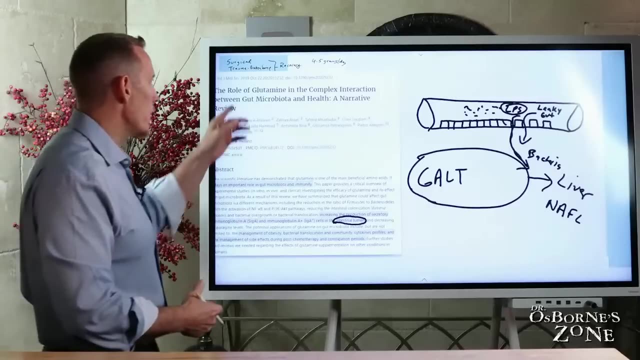 We could get LPS in there. We could also get different bacteria- and other bacterial toxins as well, translocating across the lumen of the gut and then getting access to the bloodstream, directly leading to this chronic and systemic inflammatory cascade. So we know that glutamine plays a role in maintaining this barrier. going back to the 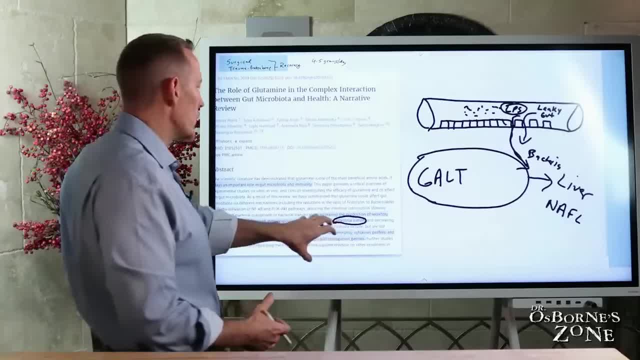 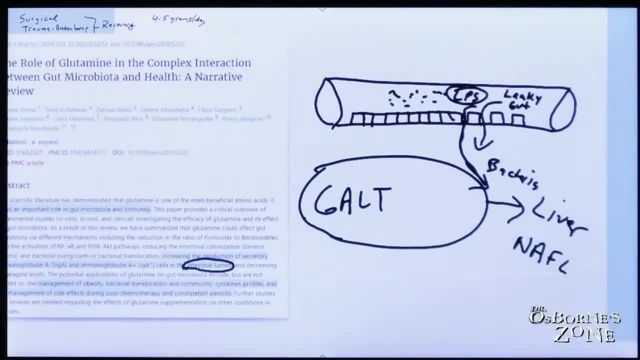 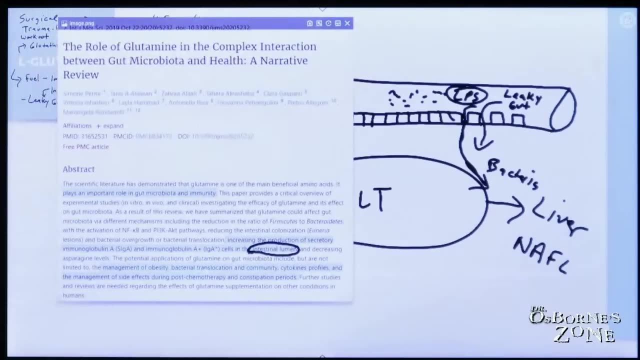 point here. This study also discusses how glutamine affects the cytokines, so the different cytokines that are produced to regulate and modulate inflammation, And glutamine plays a role in. it plays a modulation role in, but also this also discusses the management of side effects during post-chemotherapy and constipation periods. 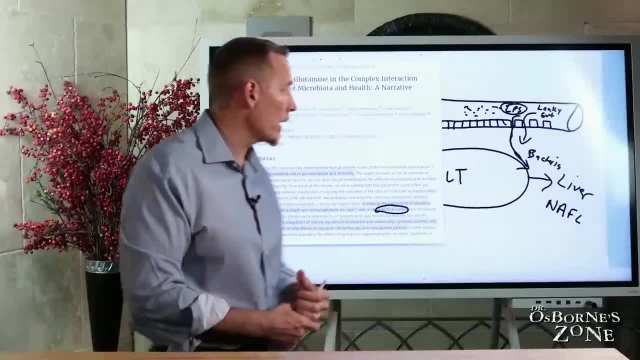 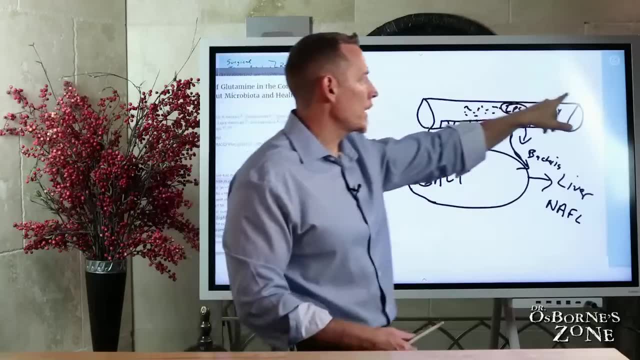 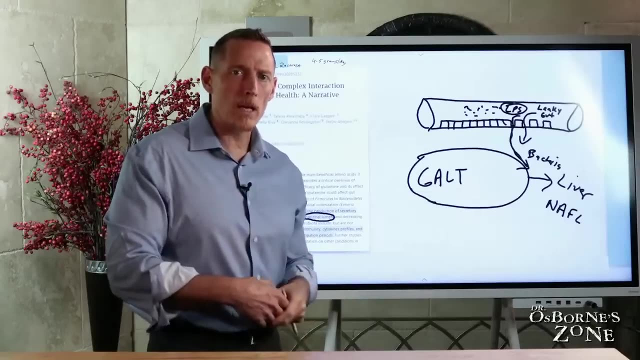 So patients that have gone on chemotherapy a lot of times they damage their gut, opening their gut up for this type of again translocation and the importance of glutamine here to seal that gut back up to prevent some of that damage. So many of you may be out there watching this getting treated for cancer. 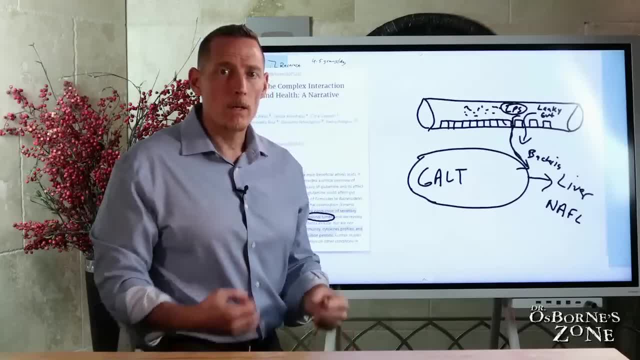 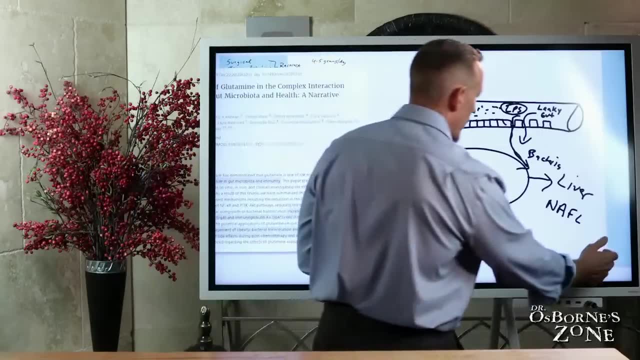 You know you're post-chemotherapy, your gut's blown open, your immune system is reeling from the chemo and you're trying to make a recovery. You might look at glutamine as a potential ally to help that recovery, to help support. 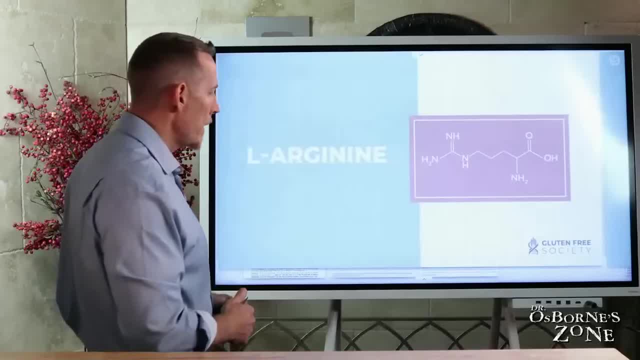 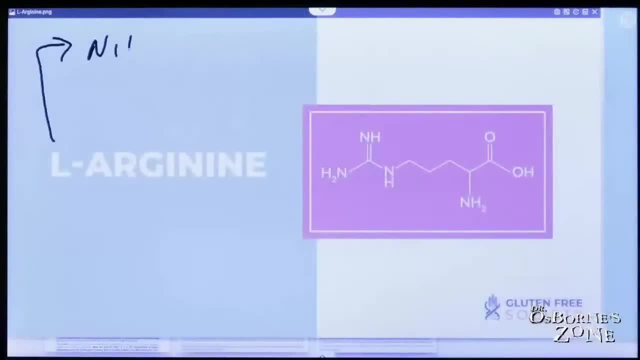 it. Okay, Let's talk about L-arginine. L-arginine is another amino acid and it's one of it's major roles is in the production of a compound called nitric oxide. This compound, by the way, is called nitric oxide. 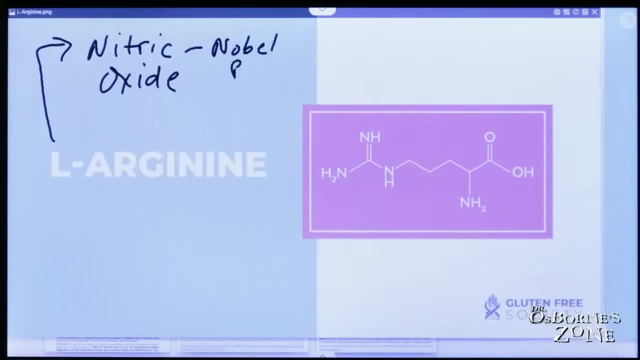 Okay, They won a Nobel Prize in science for the understanding of how it regulates blood pressure. Nitric oxide helps with blood vessels. So again, look at a blood vessel. It's a blood vessels made out of a collagen outlie and a matrix of muscle, right? 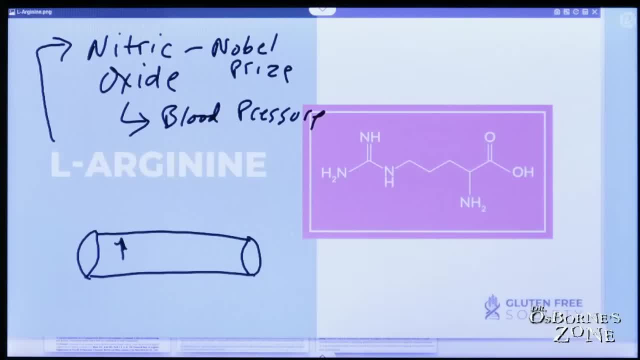 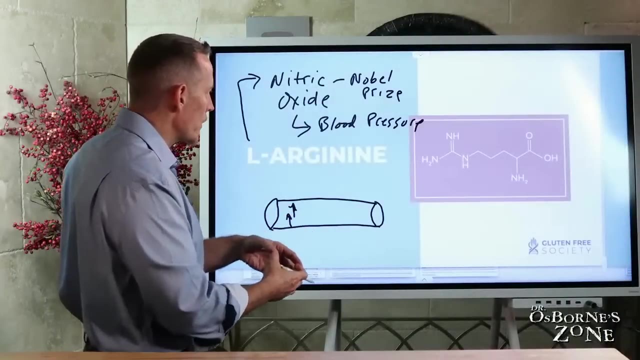 And so this blood vessel will, It will contract and relax, So it will open and it will close. It will open and it will tighten up, And so that vasoconstriction, vasodilation of a blood vessel in large part is regulated. 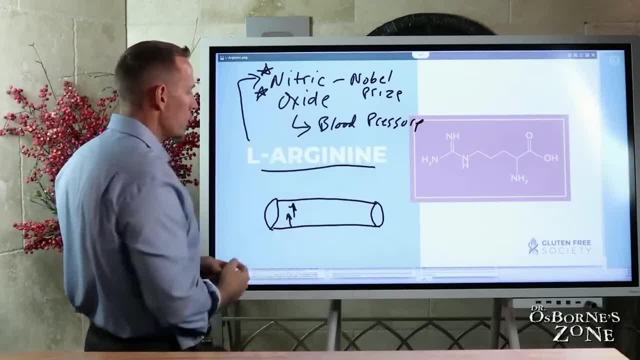 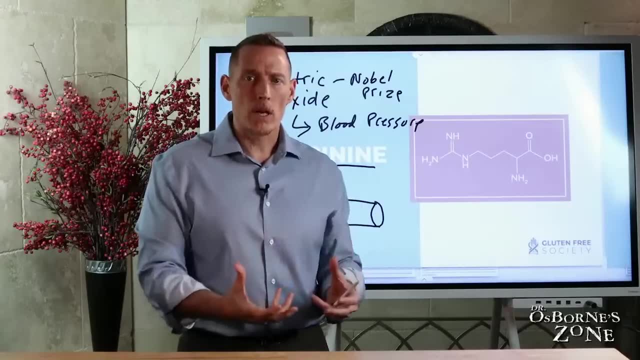 by this substance, right here, this nitric oxide, which again L-arginine is required to make So one of the side effects, potentially of L-arginine deficiency, when your blood vessels can't properly dilate and constrict. Okay. 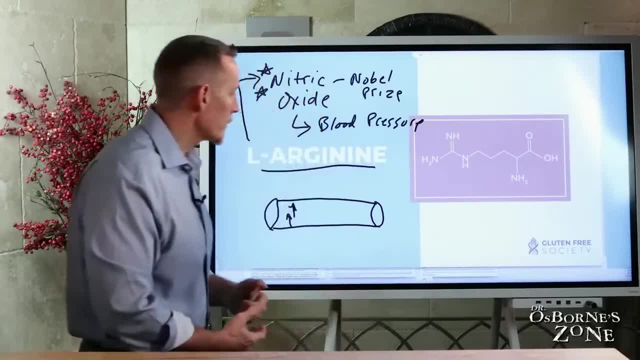 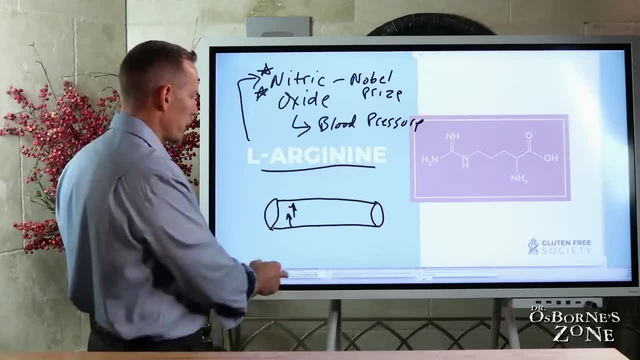 So it's just a matter of elevations in blood pressure And we see that play out in a number of individuals, a number of research studies. So major, major role of L-arginine is in that regulation of blood pressure. Let's talk about some of the research on this. 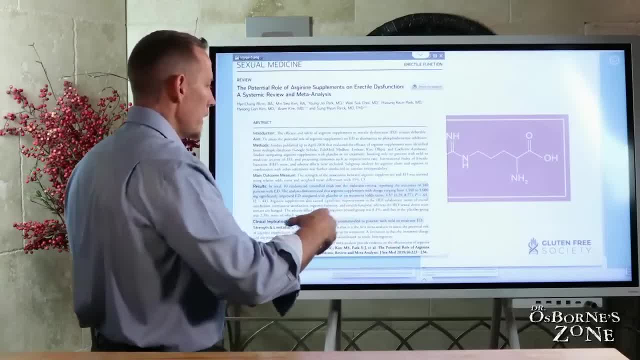 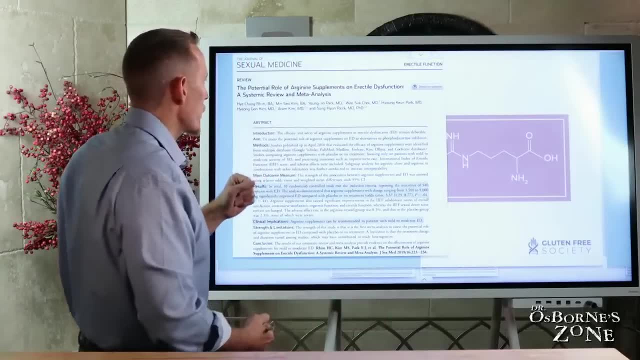 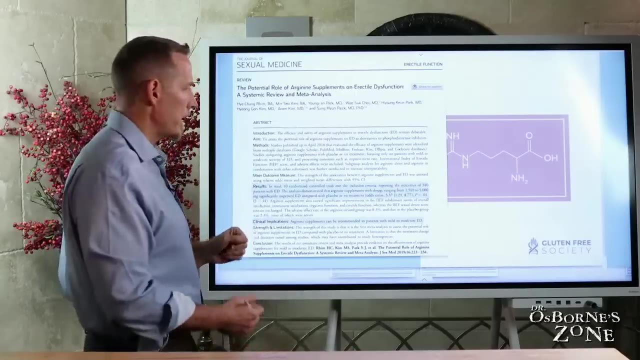 So, as we were talking about a minute ago the blood vasodilation effect we talked about in this particular study published in the Journal of Sexual Medicine on the role of arginine supplements- Arginine supplements on erectile dysfunction, And so this was a systematic review and meta-analysis of a number of different trials. 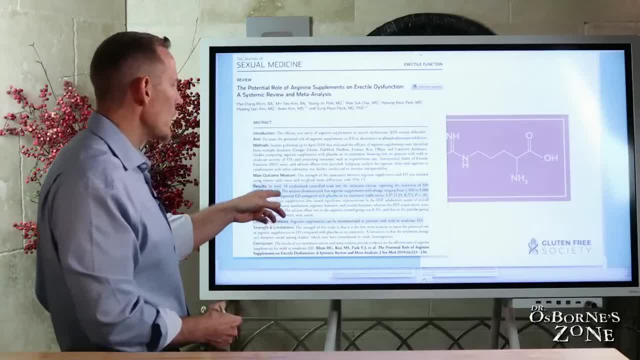 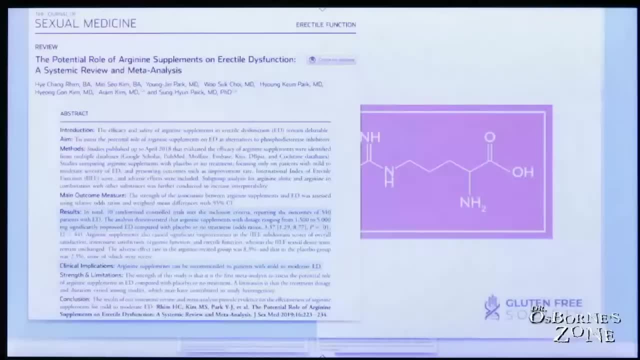 In this case, 10 different studies were looked at. The analysis demonstrated that arginine supplements with dosage ranging from 1,500 to 5,000 milligrams significantly improved erectile dysfunction compared with placebo or no treatment. P-value greater than 0.01 means that's an extremely statistically significant increase. 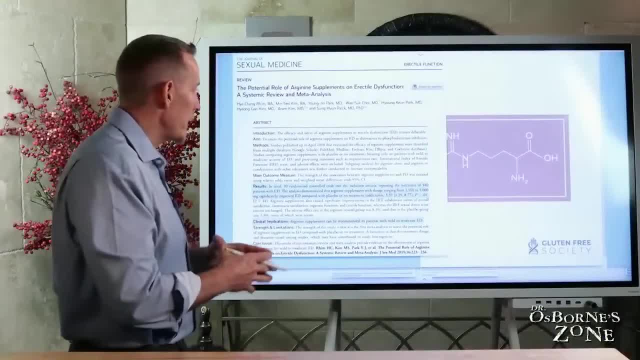 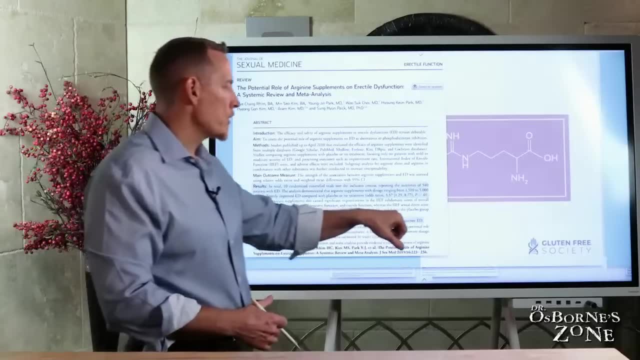 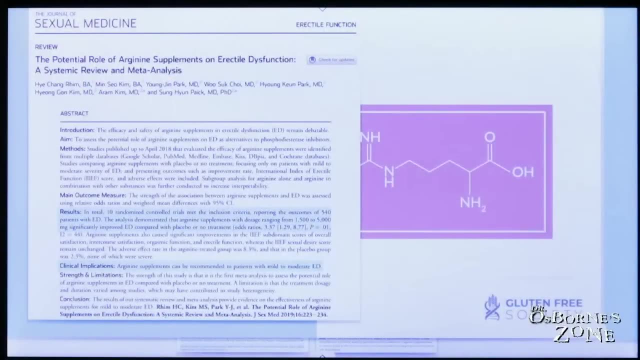 Okay. So this is a very significant correlation, meaning this: definitely, arginine definitely works in this regard. So arginine supplements can be recommended to patients with mild to moderate EDs. kind of the clinical implication. finality of this study. How many of you, how many of you men watching this, you know, ever gone to your doctor? 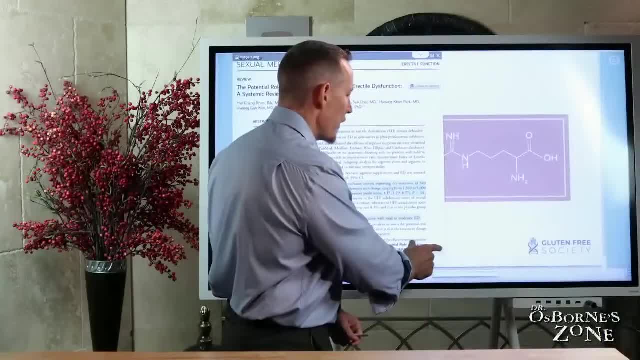 maybe you don't want to talk about it on YouTube or in this video, but how many of you have ever gone to your doctor and instead of them saying, hey, let's measure your arginine, make sure you have the basis to produce no arginine? 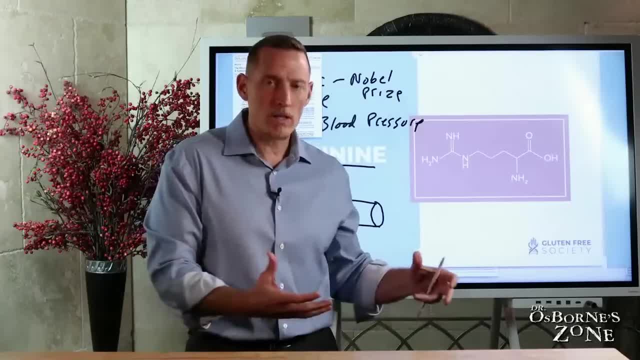 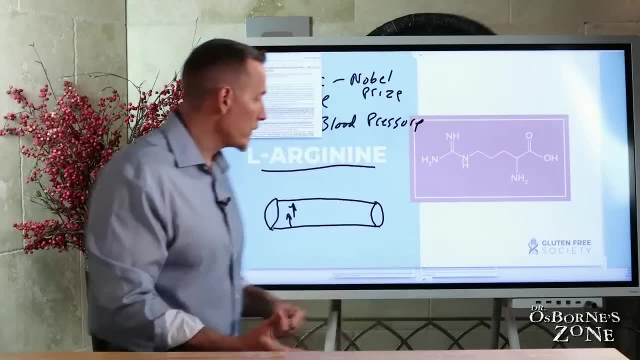 Okay, Let's make sure you have the basis to produce nitric oxide, so that your you know your dysfunction is not necessarily being caused by malnutrition, or they just give you a pill, right? They just give you one of those pills. 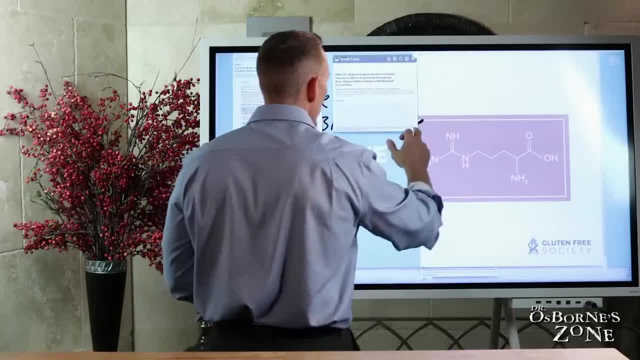 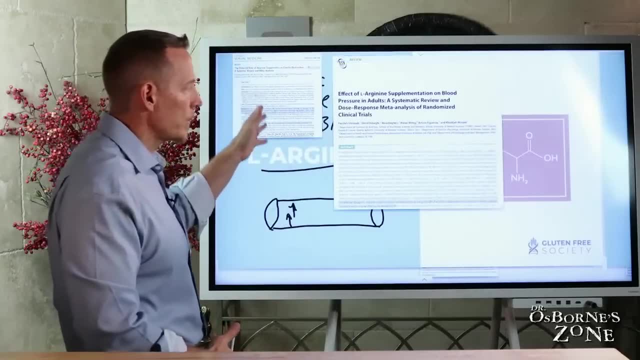 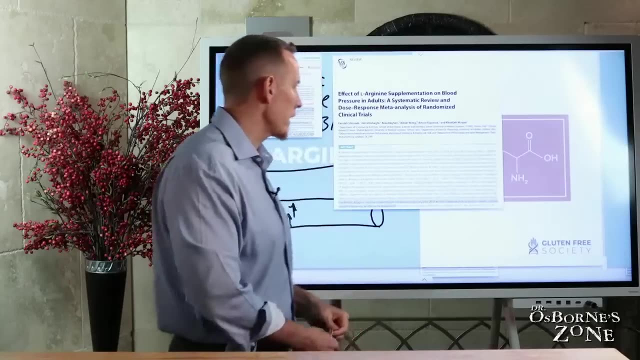 You guys know the ones, you know the pills to resolve erectile dysfunction and really, and it's the chemical manipulation versus the natural correction of a problem, I always like to go with the natural correction of a problem because the chemical interferences, the chemical medicines, they don't come without. 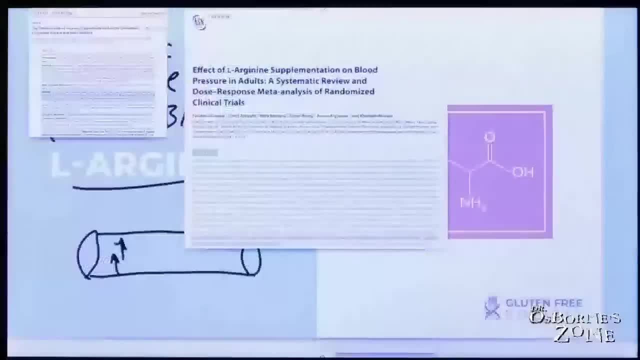 They're side effects. Here's another study on blood pressure. You see the effects of L-arginine supplementation on blood pressure in adults. Another systematic review and dose response meta-analysis of trials: you see the effective dosage of L-arginine supplementation was detected to be approximately four grams a day for systolic. 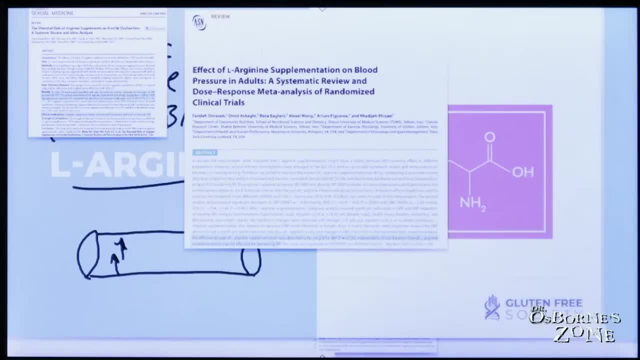 blood pressure. So four grams a day with lower systolic blood pressure, independent of duration. Overall arginine supplementation may be effective for decreasing blood pressure Again. So if any of you guys or gals have been to a doctor, your blood pressure is high. the 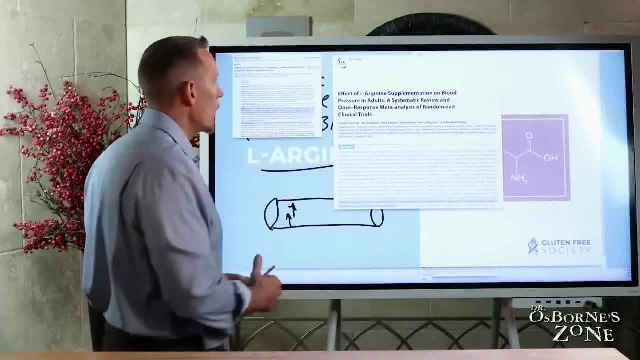 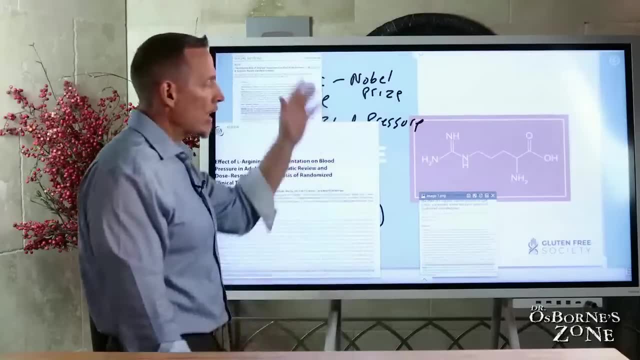 first thing they want to do is put you on blood pressure medicine. They didn't test whether or not you were producing nitric oxide. They didn't measure your arginine levels, which, again, this can be a cause. Remember, arginine is an amino acid. 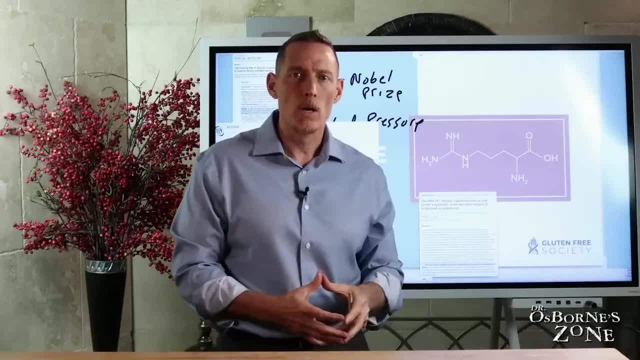 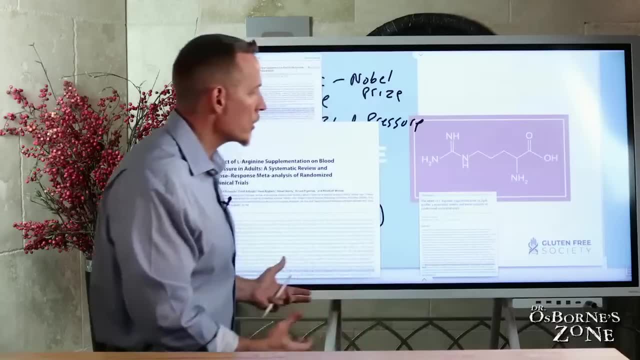 It's a nutrient the body needs in order to properly function. So this is why I always come back to nutrition, because if your body's not getting what it needs nutritionally, it will malfunction. In the case of arginine, that malfunction can manifest. 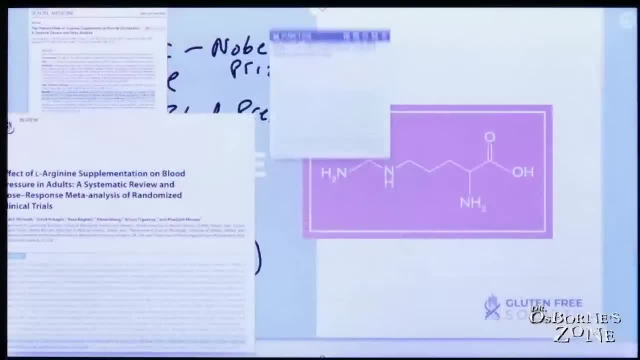 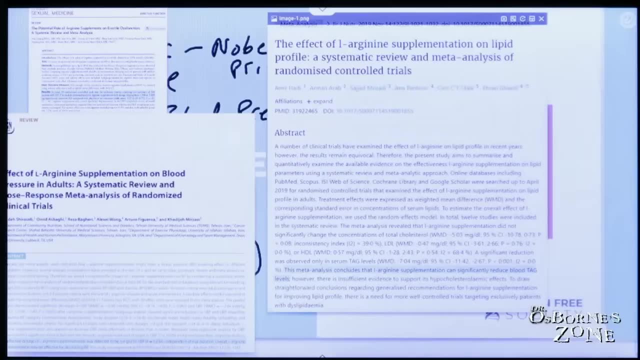 It's a rectal dysfunction and blood pressure problems. So again, take the drug or figure this part out. It's easier to figure this part out, in my opinion. This study the effect of arginine supplementation on the lipid profile. So another systematic review and meta-analysis. 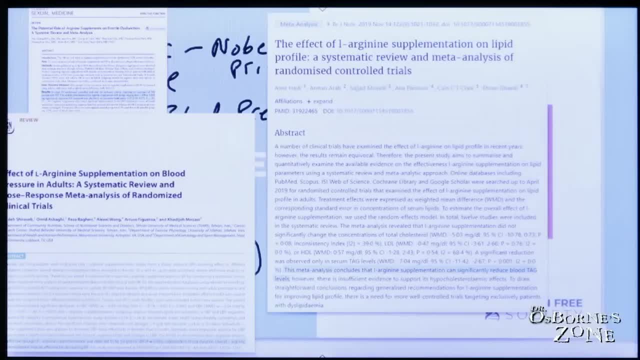 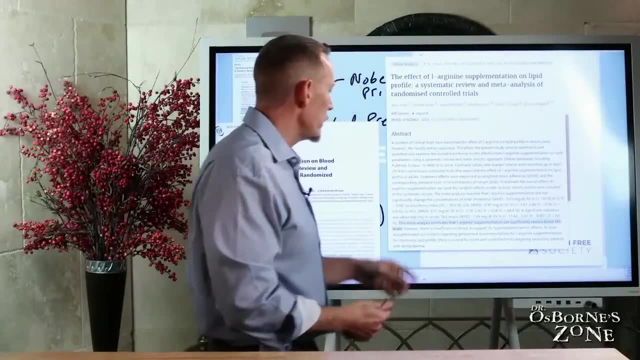 So, guys, these are systematic reviews and meta-analysis. This is a study on a conglomeration of all the studies to look at how effective something is therapeutically. You can see in this. meta-analysis concludes: Okay, Arginine supplementation can significantly reduce triglycerides. 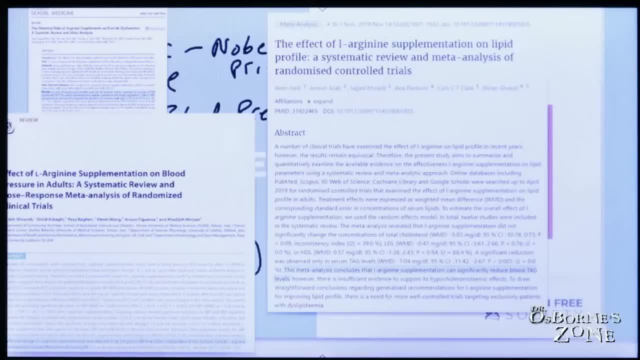 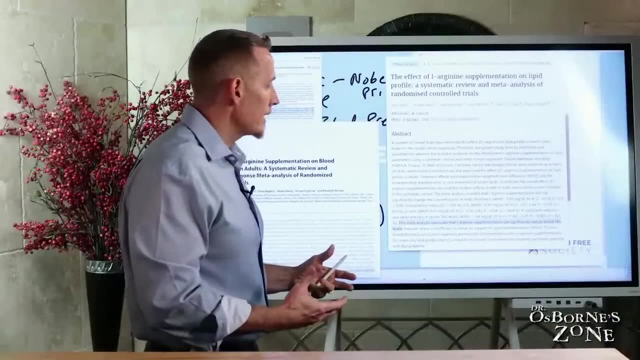 T-A-G stands for triglycerides. So how many of you have had high triglycerides? You go to your doctor. your triglycerides are high. That usually stimulates, even though the statin drugs, the cholesterol-lowering drugs, don't. affect triglycerides. A lot of times, if you have high triglycerides, your doctor wants to put you on statins. Don't ask me to try to explain that. I can't speak for why your doctor would want to do that. 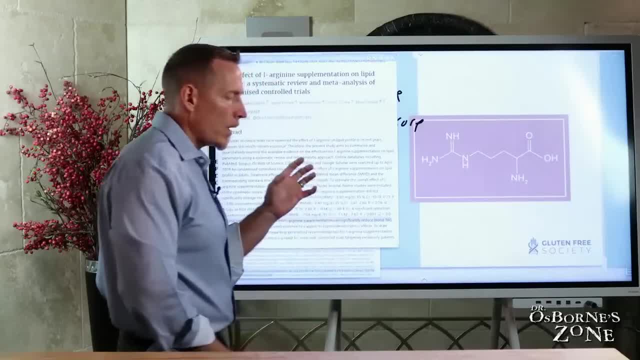 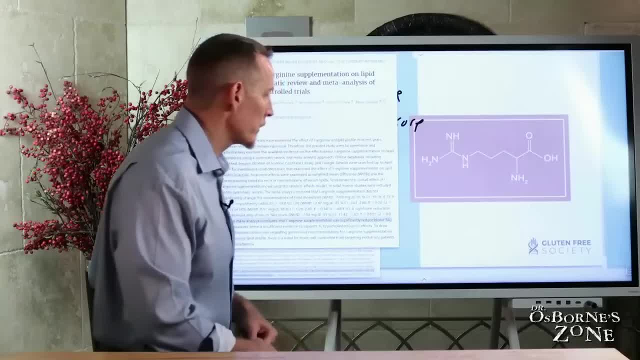 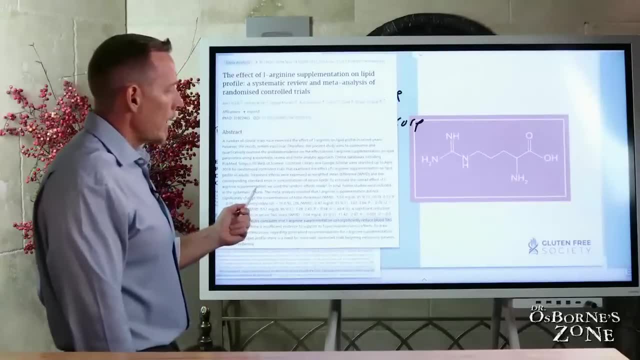 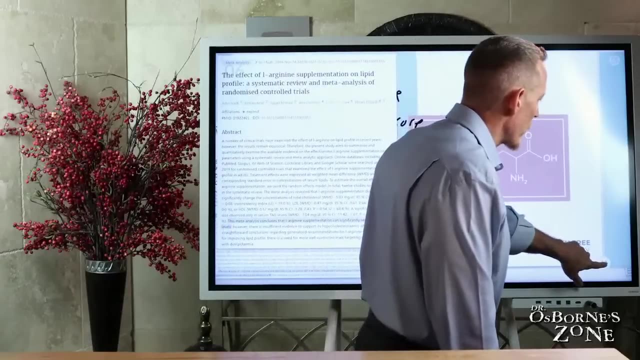 into your liver, thus compromising its ability to function, detoxify the blood appropriately, leading to all kinds of inflammatory problems. So again, arginine as a supplement, showing the ability for it to reduce that triglyceride. Reduce triglyceride levels as part of its role in regulating fat synthesis or metabolism. 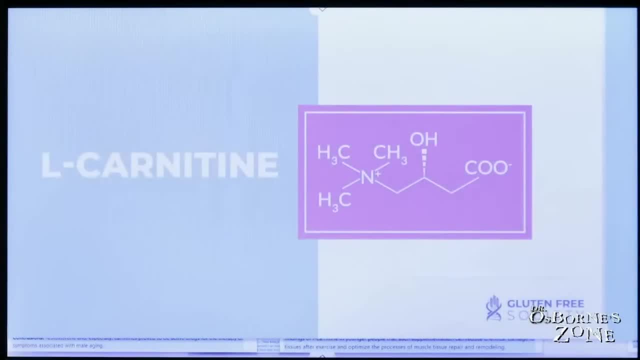 All right. next, let's talk about carnitine. Carnitine, very important amino acid. One of its primary roles is in this process called beta-oxidation. Now, beta-oxidation is the breakdown of fat into energy, ATP. 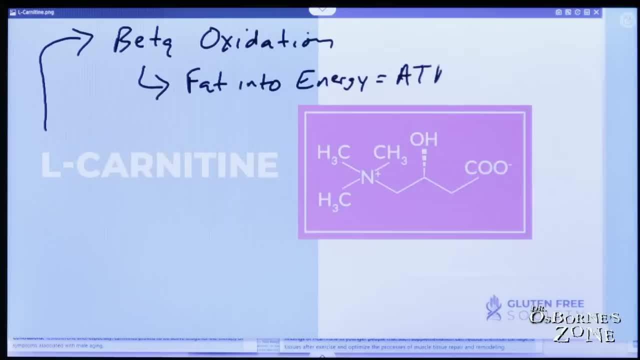 So if you've never heard anybody use that term- ATP, adenosine, triphosphate- we take fat through this process, break it down. What carnitine is is? it's the shuttle. It helps shuttle fat into the proper area of the cell to get to this beta-oxidation point. 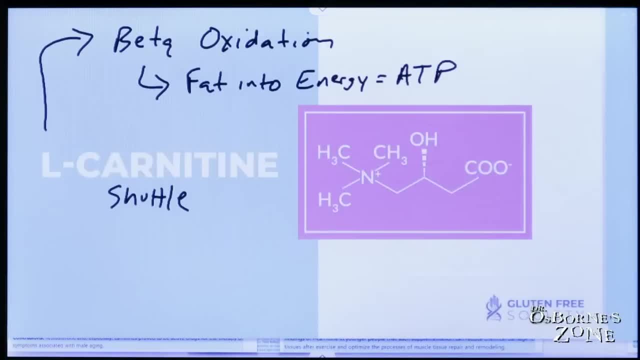 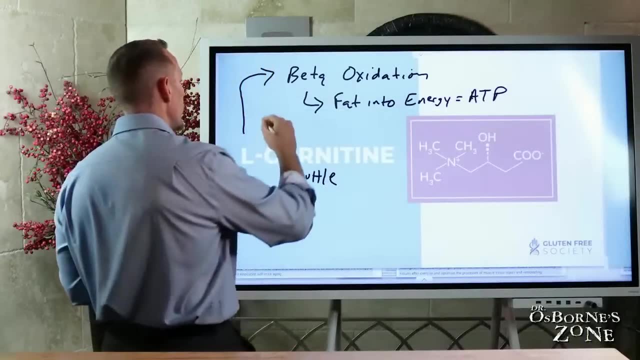 So low levels of carnitine can hinder your body's ability to burn fat as fuel. Now where this might be important for you watching is if you're following a keto like diet, especially those of you that are like doing keto green. 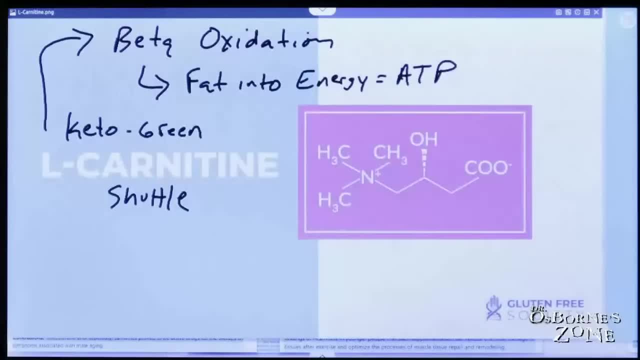 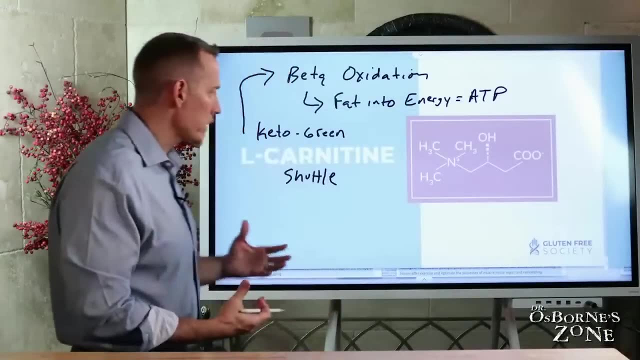 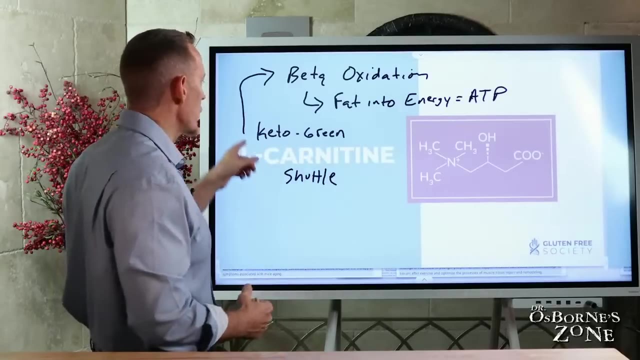 There's a movement out there which is to go high-fat diet, low-carb, but also to reduce the quantity of animal food consumption. Remember, most of our carnitine comes from animal meats. Carnitine right, That word carn just like carnivore, right. So we get our carnitine predominantly from meat. So if we're increasing our fat dramatically but not getting adequate carnitine, If you increase your carnitine through animal meat consumption, then you could end up with a problem generating energy. 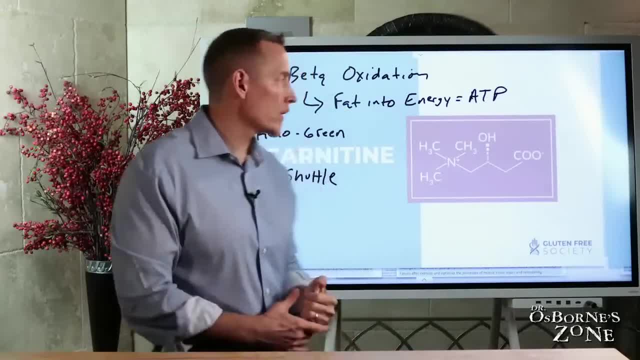 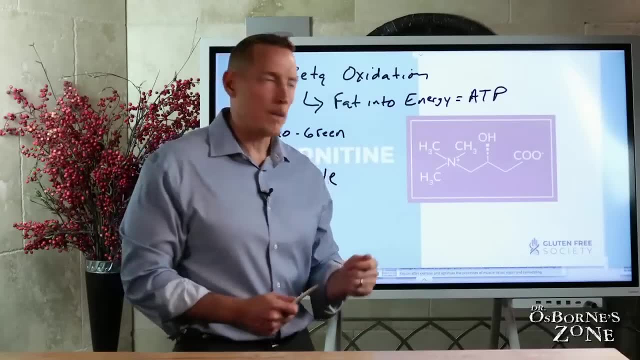 And I've seen some people who do really, really poor when they're trying to go keto, especially again in this style where they get really lethargic. They don't know where their energy went. They have no get-up-and-go. 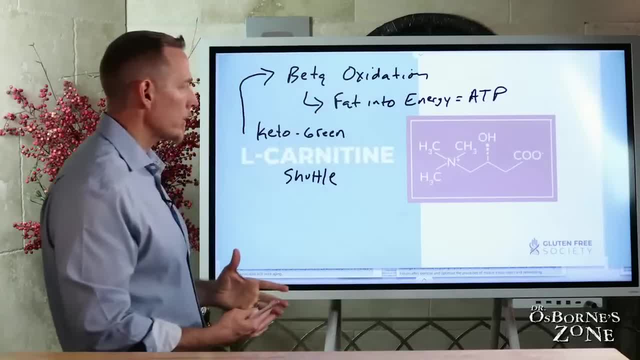 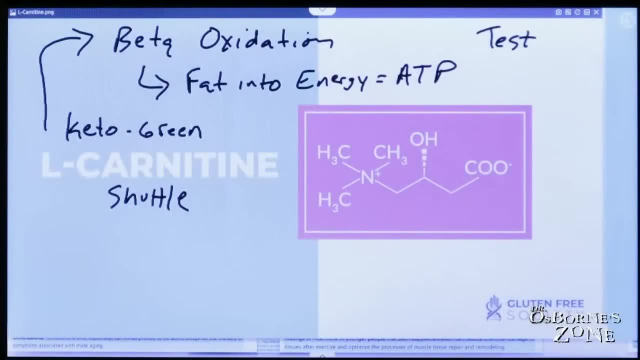 This could be part of the problem. So you might just look at carnitine And one of the simplest things is just test for it, right? Have your doctor test your carnitine levels. If they're low, you can supplement. 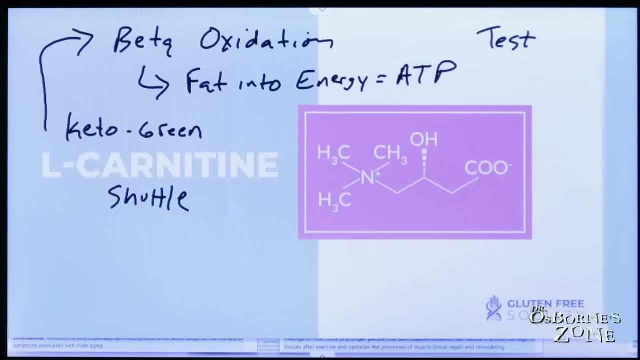 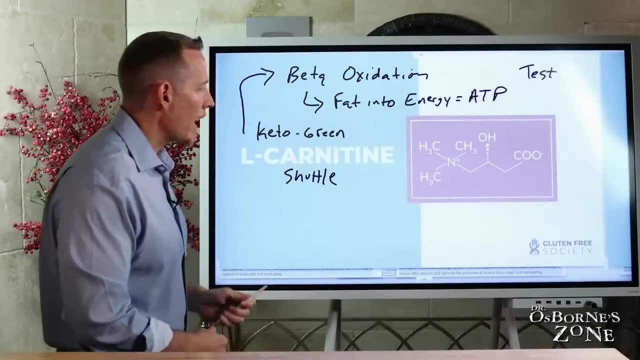 Or you can change your diet a little bit, maybe incorporate a little bit more animal products that are rich in carnitine into that, so that you're better at burning that fat as a fuel source. Now, carnitine has a lot of other different functions. And there are a number of studies that have come out on benefits of carnitine supplementation, And this particular one published in Urology. they used carnitine, as well as testosterone, in the treatment of sexual dysfunction, depressed mood and fatigue associated with male aging. 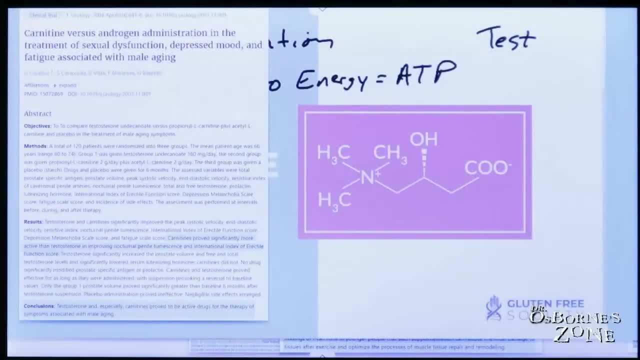 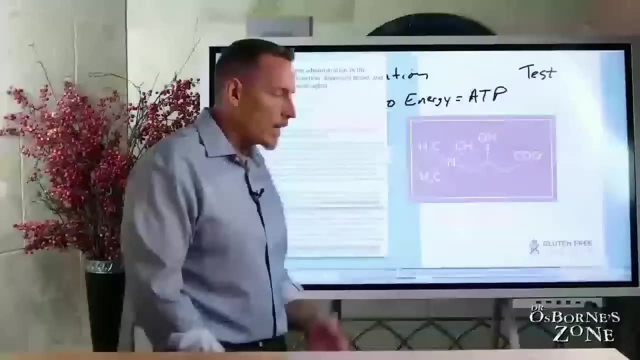 So, guys, Guys, pay attention. And what they found is that carnitine's proved significantly more active than testosterone in improving nocturnal penile tumescence, and international index of erectile function score worked better than testosterone. So again, I keep saying this: 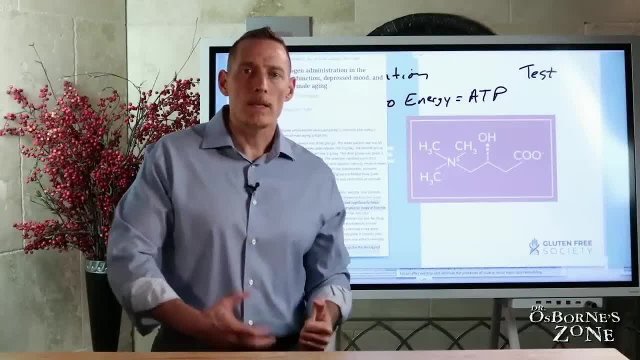 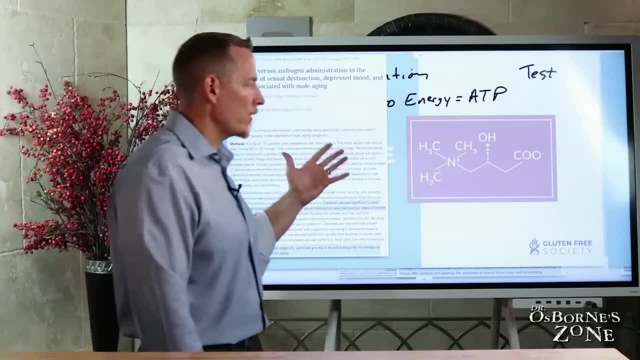 How many of you have gone to your doctor with a symptom? First thing you do is pull out the prescription pad. Here we have an example of something very, very natural and very available through your diet. It might have the potential. It might have the potential to impact you in a very positive way without having to grab. 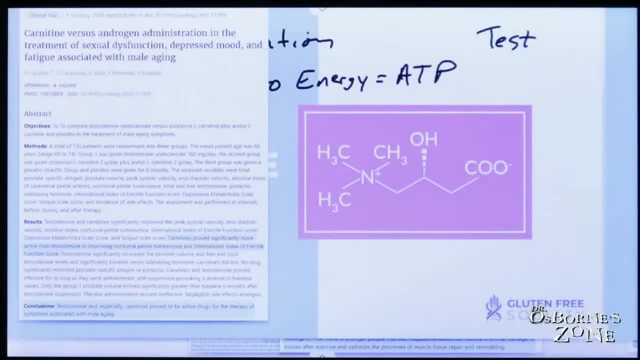 for drugs. So again, conclusion here: carnitine's proved to be active drugs. They're calling carnitine drugs- although I don't know that it would be called carnitine drugs But carnitine to be active drugs for the therapy of symptoms associated with male aging. 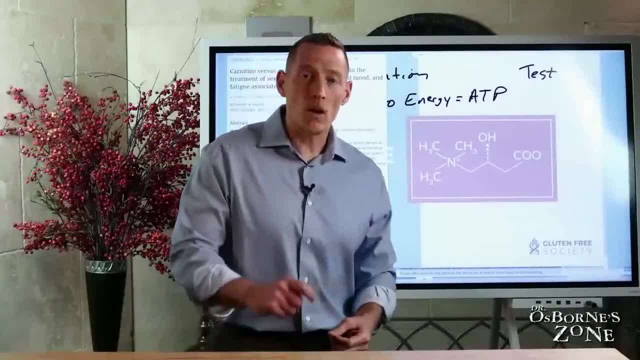 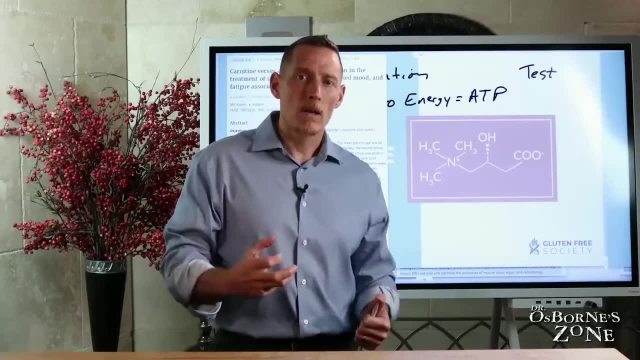 So, guys, are you getting enough meat? Are you getting enough protein? See this all the time in a lot of my male clientele is: they're coming in and their wives are trying to make their husbands go on a plant-based vegan diet And their husbands are trying to make their husbands go on a plant-based vegan diet. Their husbands are trashed, Their energy's low, They don't feel well Again: sexual dysfunction, depression and low energy. So if that's you, you might want to consider. carnitine is dropped as a result of that diet change. 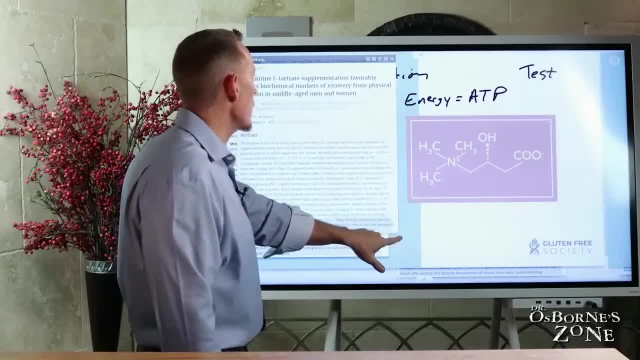 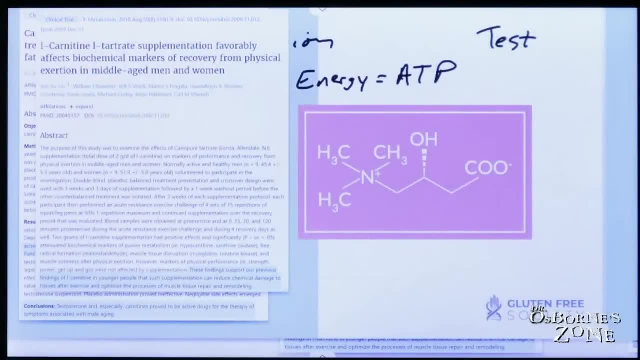 So again, simple changes, big impact. Another study here on carnitine supplementation being favorable for markers of recovery from physical exertion in men and women. So these findings support our previous findings in youth that such supplementation can reduce chemical damage to tissues after exercise and optimize the process of muscle tissue. 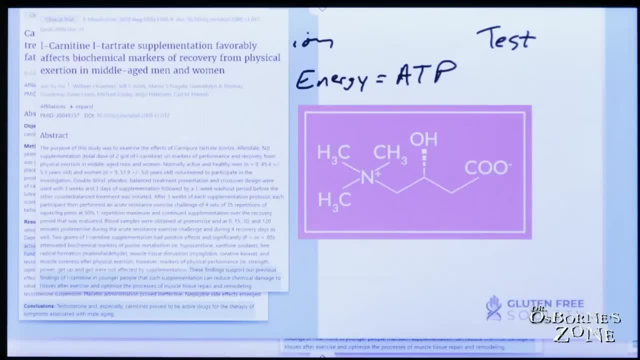 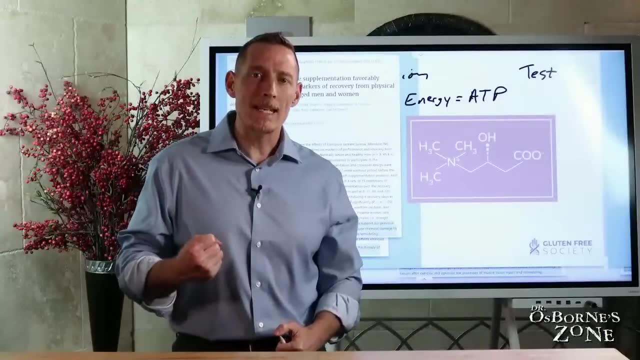 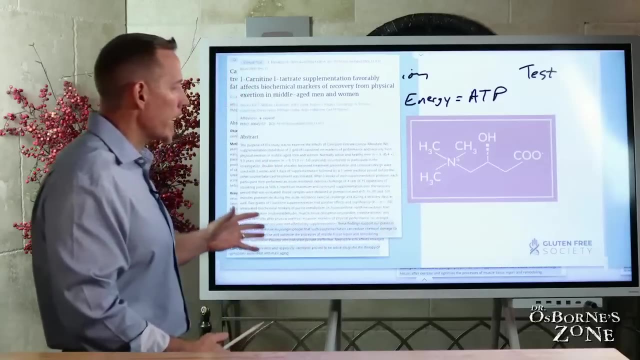 repair and remodeling. So the takeaway there is: let's say, you're working out on a regular basis, You're having a really hard time recovering. You're having a really hard time getting your body to repair appropriately. There's this potential for carnitine, post-workout right. 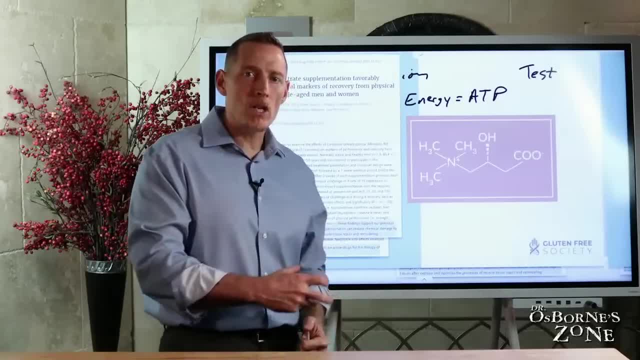 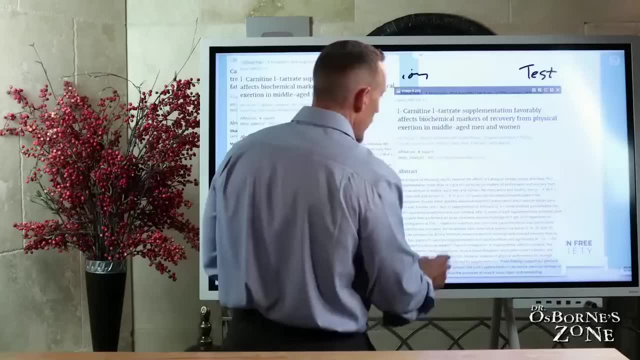 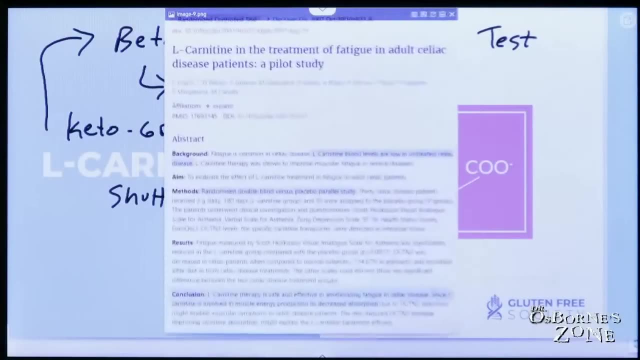 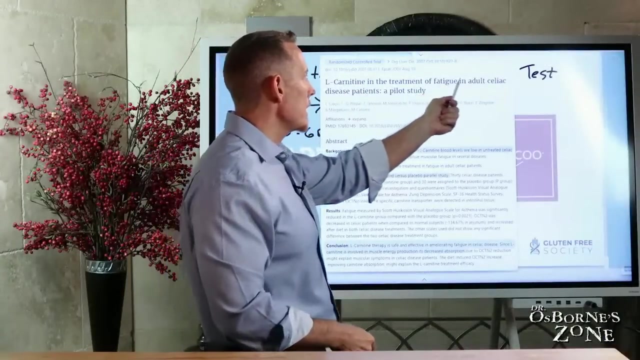 To help in that recovery, to help reduce the potentiation of the damage from the exercise. So carnitine supplementation might be very indicated in those types of individuals. So I would be remiss if I didn't include a study on gluten. So you can see with carnitine in this study, carnitine in the treatment of fatigue in adult. celiac disease patients. well, first of all, what they found was that carnitine blood levels were low in untreated celiac patients and this is a very common symptom or side effect of gluten on the GI tract. Remember it damages the villi, leading to malabsorption, and that damage, of course. 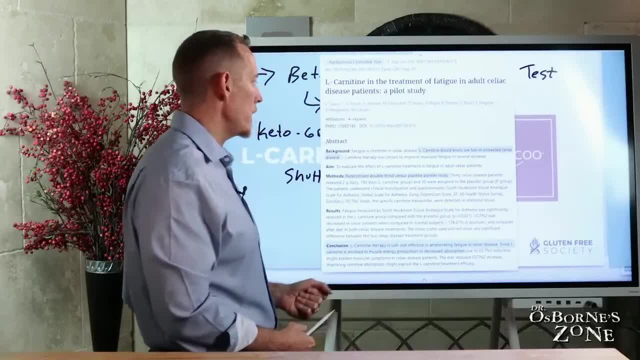 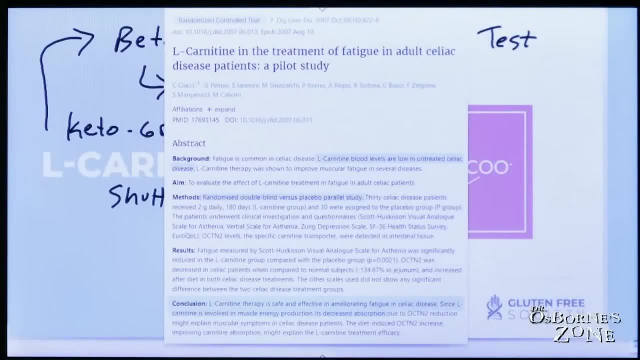 causes all kinds of nutritional deficiency, carnitine just being one of the many. But this study went on to find that carnitine therapy is safe and effective in ameliorating fatigue in celiac disease. So if you're gluten-free, you're going to have a lot of pain. 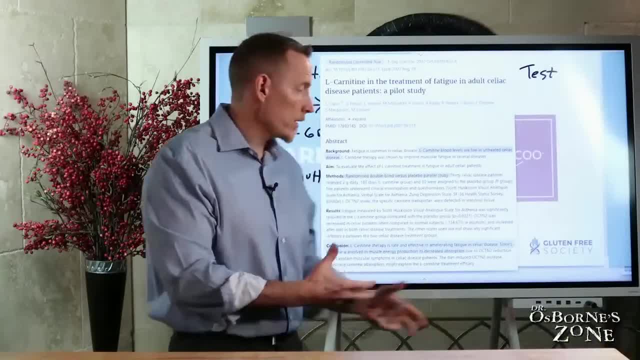 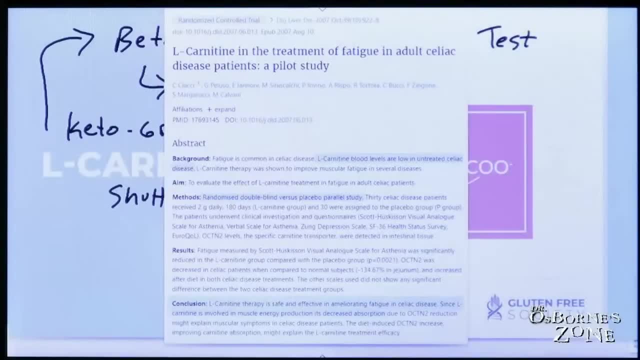 You're going to have a lot of pain If you're gluten-free, think you're gluten-free and struggling. you might want to look at carnitine. You might want to have your doctor measure the amino acid levels for you. Since L-carnitine is involved in muscle energy production, it's decreased absorption. 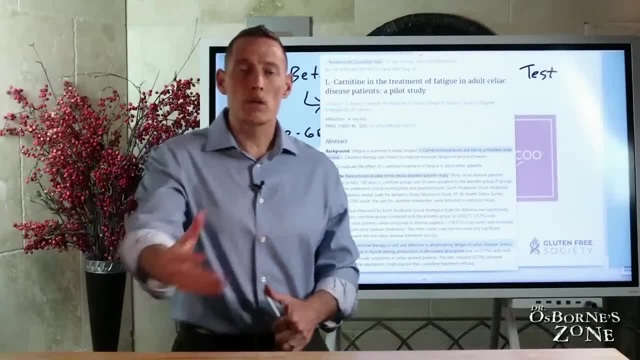 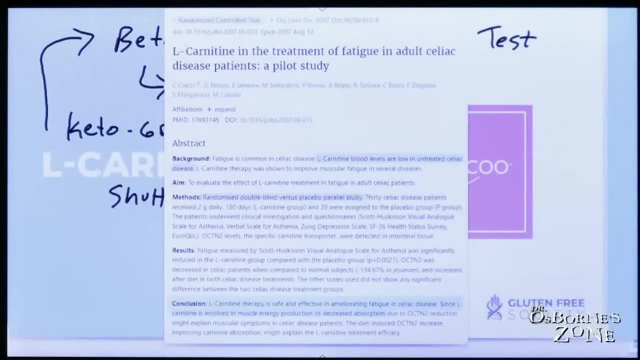 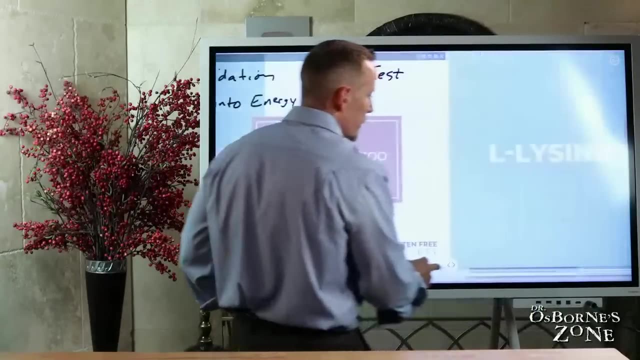 So, again, if you're celiac and you're still struggling, maybe your diet's gluten-free- you might want to have your carnitine levels measured and looked at, because it might just help you with a recovery. Okay, Okay. So let's move on to L-lysine, very important amino acid. 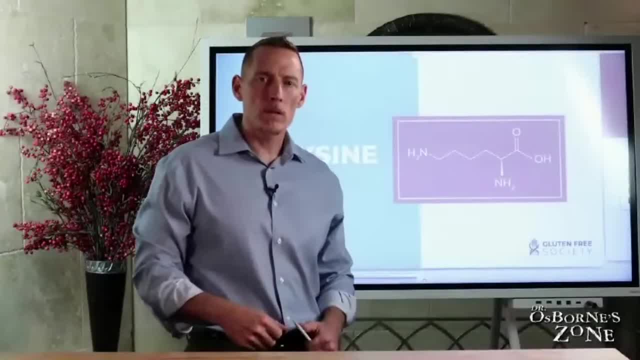 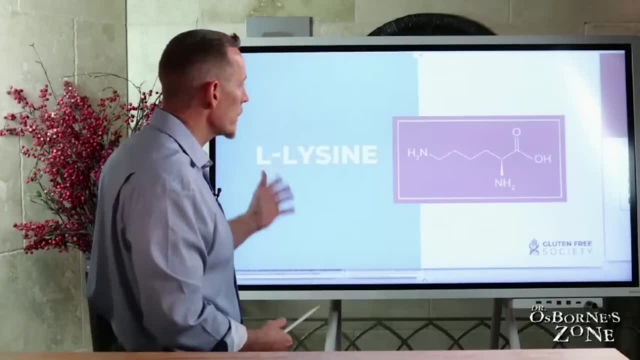 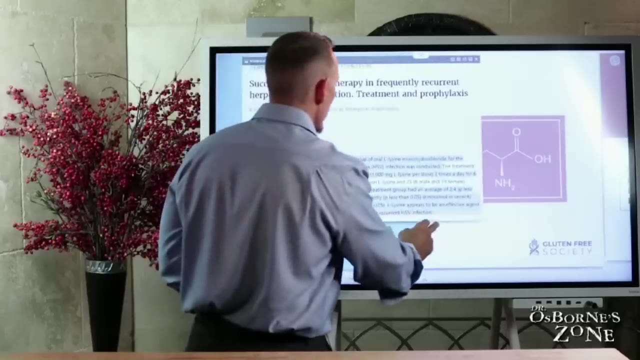 It's commonly used as an over-the-counter remedy for herpes simplex viruses. Those of you that suffer with aphthous ulcers or fever blisters- lysine- again a common ingredient in a number of those products. If we look at some of this research, the research goes pretty deep on this, but success of L-lysine. 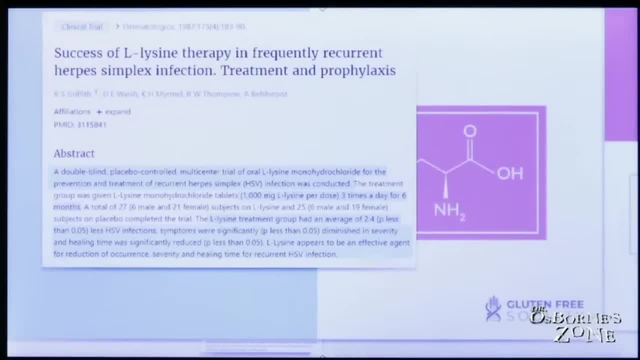 therapy. L-lysine was used to treat recurrent herpes simplex infection treatment in prophylaxis. You can see this double-blind, placebo-controlled, multi-center trial using L-lysine for the prevention and treatment of recurrent herpes virus infection was conducted. 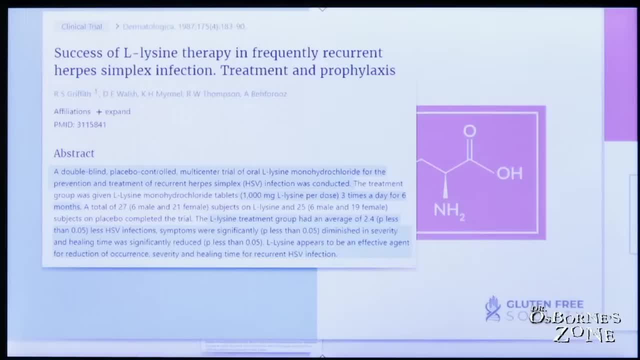 They used 1,000 milligrams of lysine three times a day for six months. Now the outcome was that the treatment group had an average of 2.4 less infections. symptoms were significantly different, Herpes was significantly diminished in severity and healing time was significantly reduced. 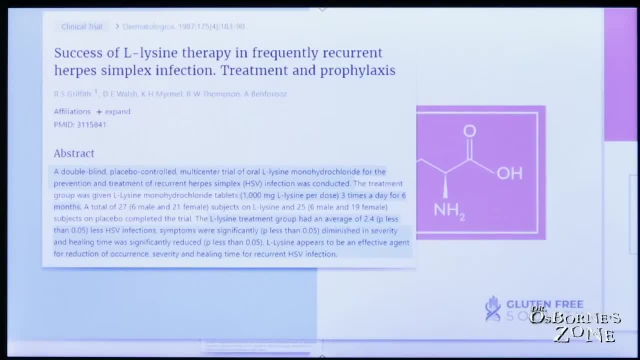 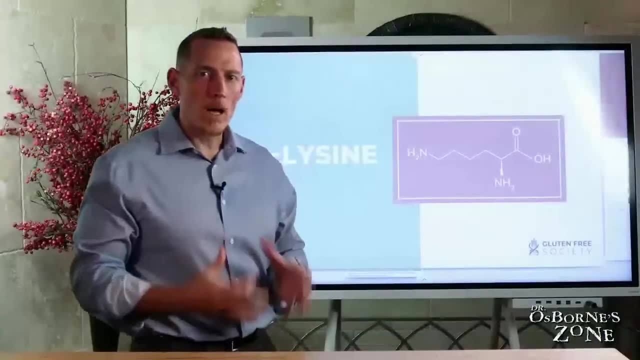 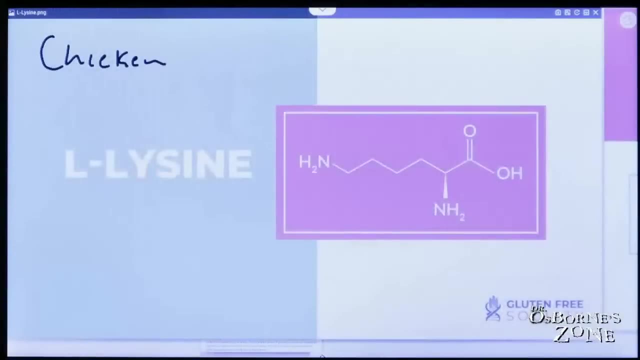 L-lysine appears to be an effective agent for the reduction of a current severity and healing time for recurrent HSV infection. Now, remember what is herpes simplex virus. Now, what a lot of you want to realize is that the herpes simplex virus family includes chickenpox. 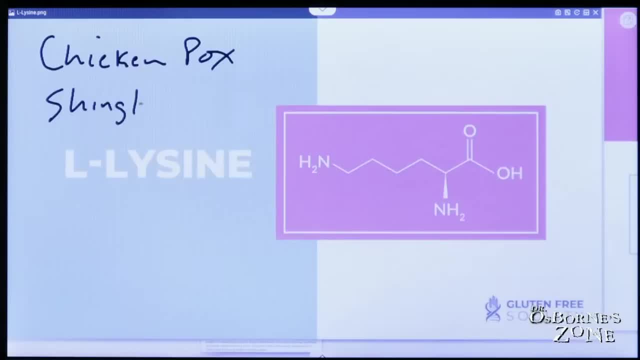 It includes adult chickenpox, otherwise known as shingles, Shingles, Shingles, Shingles, Shingles, But it also includes people, again, that get recurring mouth sores or mouth ulcers. So if you're one that you know for years, chronically, periodically, you get just sores. 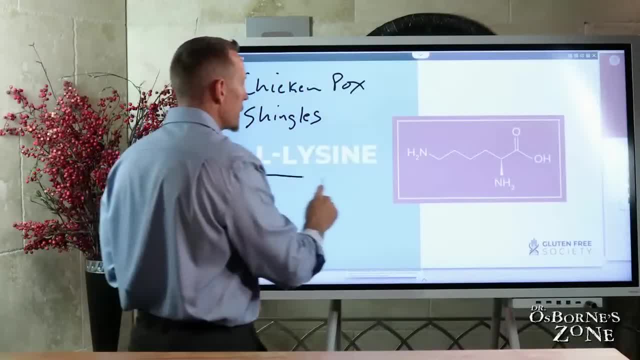 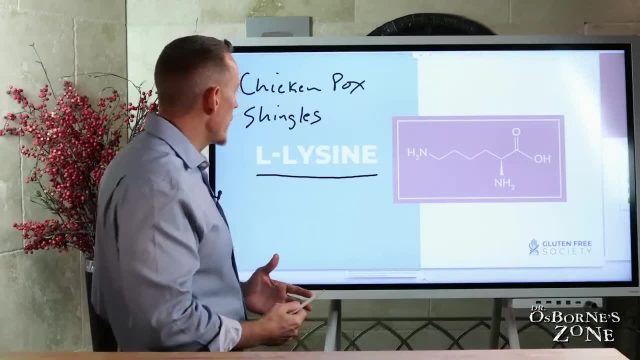 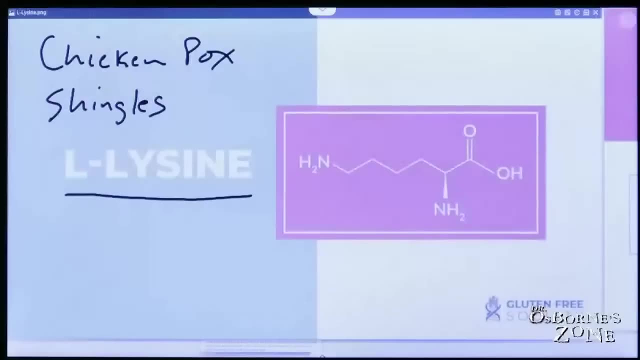 in your mouth, ulcers in your mouth. this is lysine. Lysine is your go-to. Again, in the research study it was three grams a day was what was given. Now what many studies also show if you look at lysine in combination with things, so in 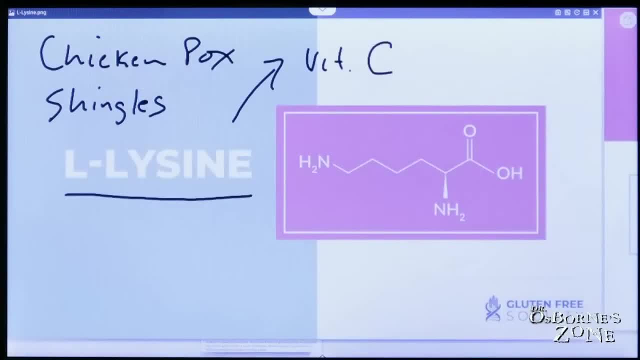 combination with things like vitamin C. ễ Trying to get this one. Anyway, if you look at this, the mouth ulcer of backcountry symptoms- if that is normal, if it is возможно, forgun когоbe, if that are mounting or not, it gets even more efficient. 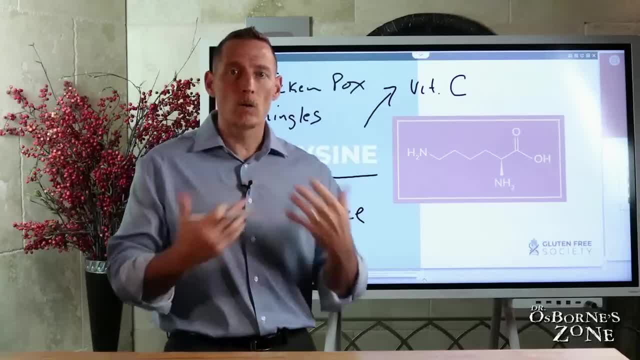 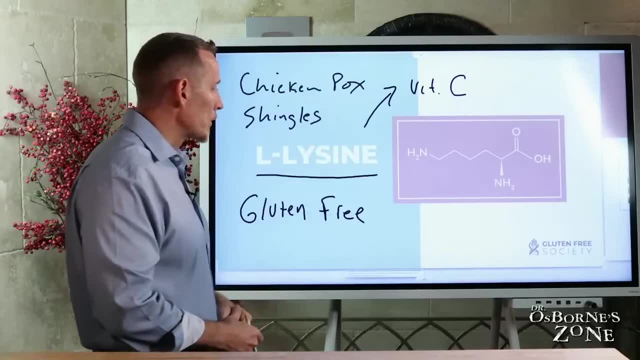 and even more effective, going gluten-free, saying I no longer get fever, blisters or mouth sores at all since I've gone gluten-free. remember gluten- if you're gluten sensitive will. basically it's a pressure on the immune system. and what? why do viruses happen? 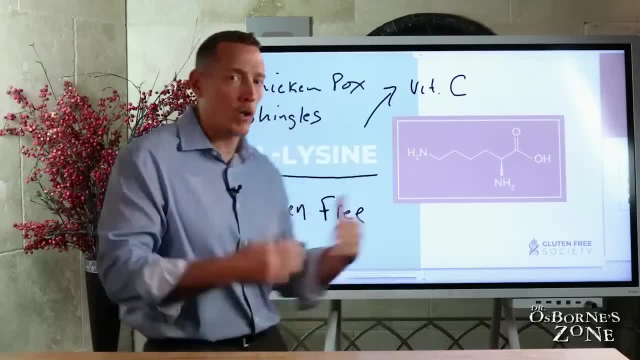 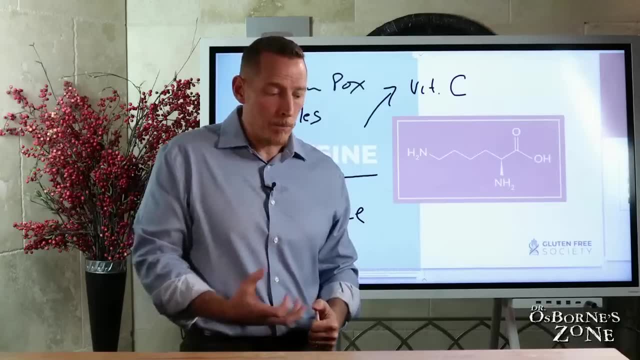 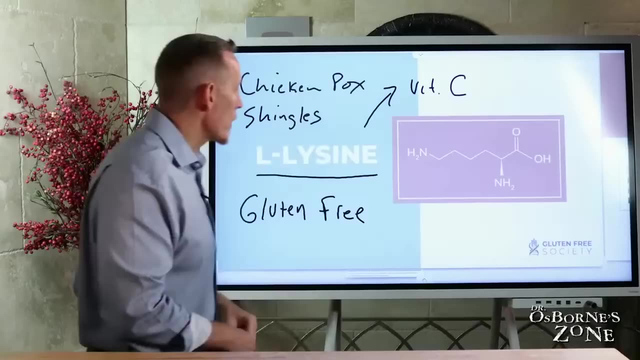 why do we get outbreaks of viruses? these are viruses that live in all of us. we all have inside of us shingles or herpes simplex type viruses. they're there, they're basically. they're dormant and they live in our, in our drg, our dorsal root ganglia, in the nervous system and when our immune system takes a great tax. 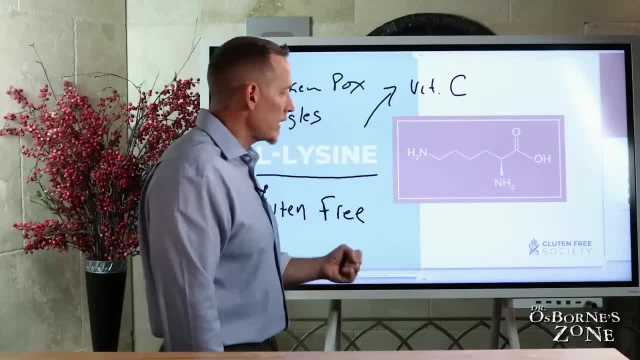 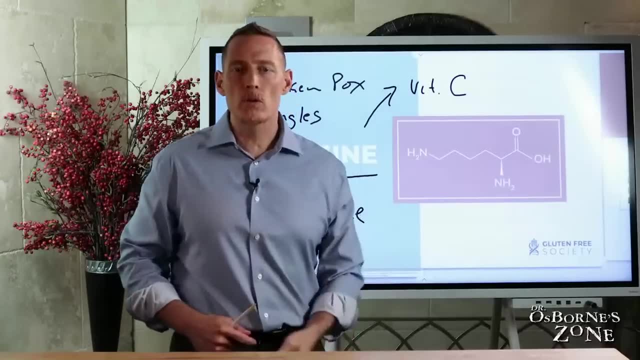 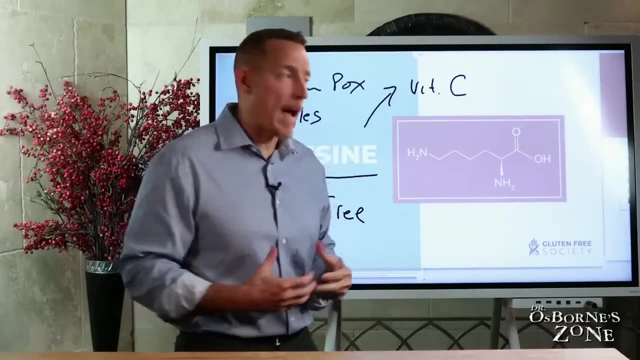 or a great stress, those viruses can be activated and that's when we'll pick up something like shingles or that's when we'll get mouth ulcers. so big periods of stress, eating the wrong food, exposure to toxins can all be triggers for virals, for viruses that are dormant to become active, and l-lysine helps to. 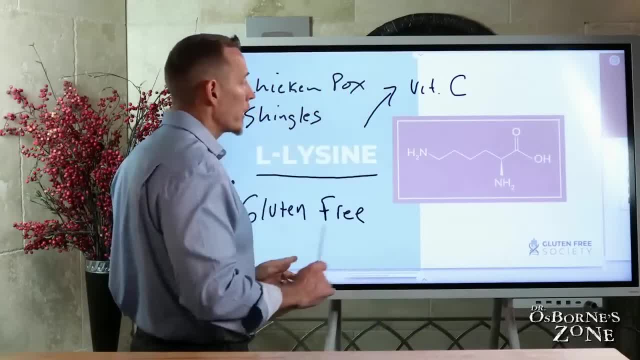 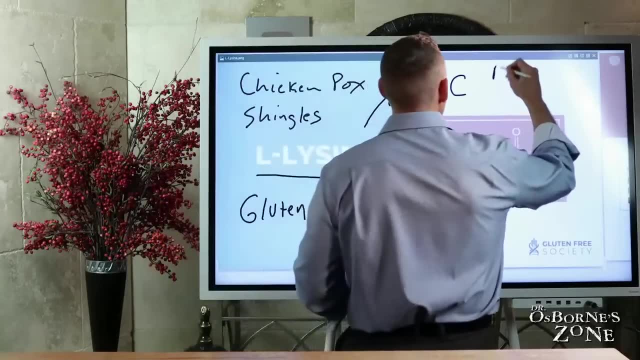 you prevent their activation now? yeah, I mentioned earlier I didn't say this, but I wanted to. I want to say this- I'm going to back up a little bit, because we're talking about arginine earlier and one of the things I want you to understand is arginine. we said it improved blood pressure and arginine can help with. 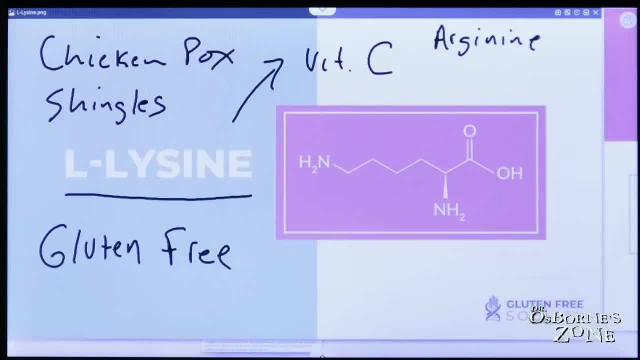 erectile dysfunction, among other things. but if you're taking high doses of arginine it's going to impact your lysine and I've seen cases where people were taking- especially men- for like erectile dysfunction, taking high doses of arginine start to break out with fever blisters, increase and increase their potential. 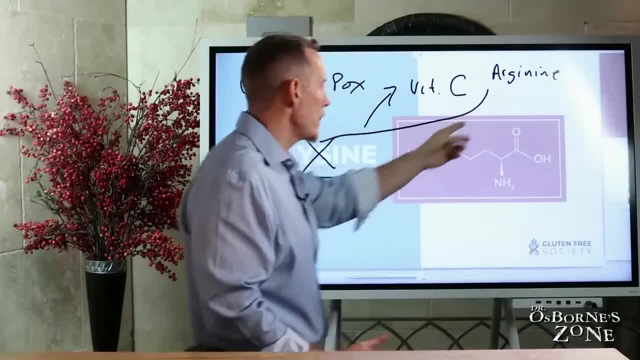 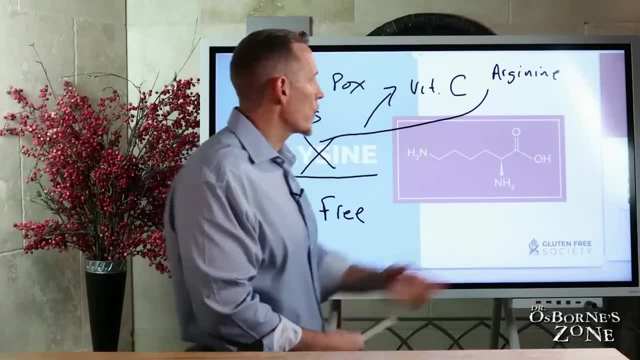 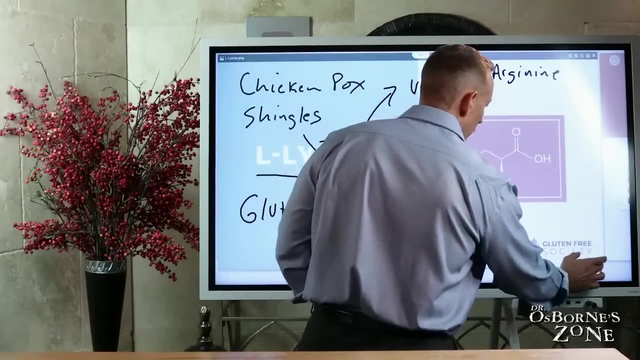 chance of developing shingles. so if you're using high doses of arginine, just be very, very cautious. if you have a history of herpes outbreaks, that that it may not be the best move for you in that regard, but again, lysine can be very, very important in the in the viral realm of helping inhibit viral replication. so 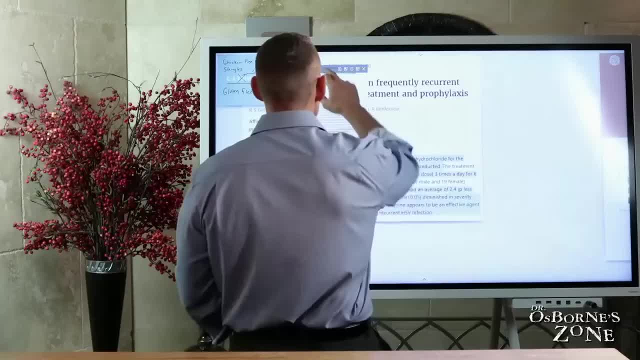 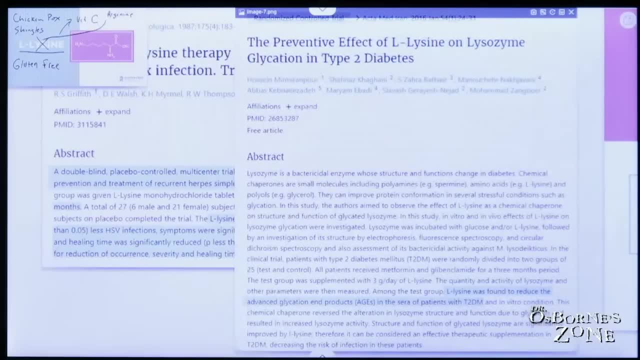 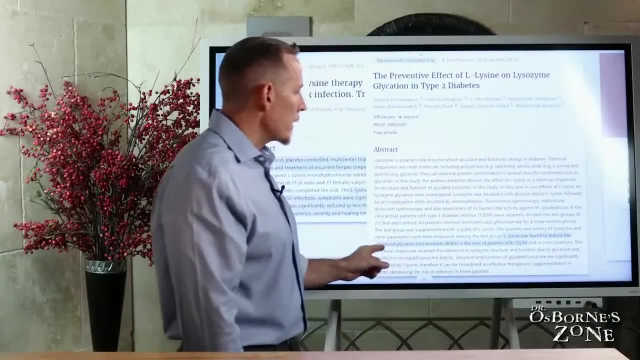 let's pull up this next one. here you can see the preventative effect of lysine on lysozyme glycation and type 2 diabetes. so just another important component to lysine that's been studied is it was found to reduce the advanced glycation end. 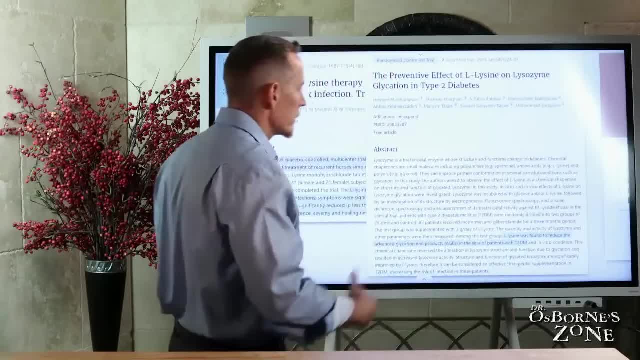 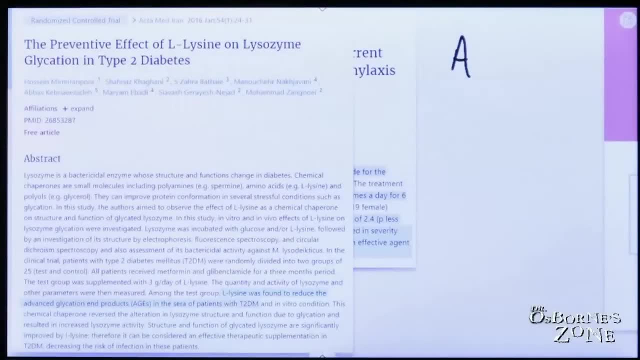 products in the serum patients with type 2 diabetes. now what does that mean? let's make that sound like English. we say advanced glycation end products, also known as ages. these are basically when sugar moieties attached to proteins in the blood. so what happens with type 2 diabetics or blood glucose levels are high? that 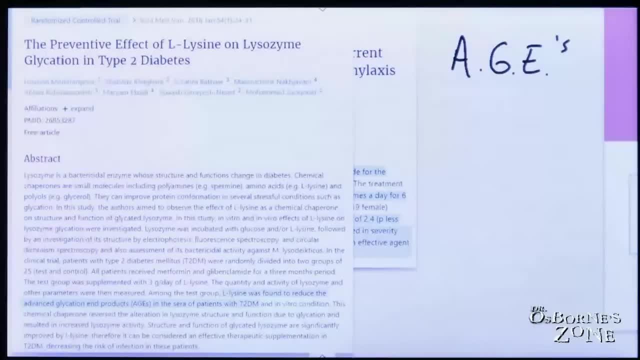 glucose interacts and it binds to proteins in the blood, forming these age compounds, these advanced glycation end products. these are the things that we believe contribute to dementia and vascular damage, increased risk for stroke and heart attack. one of the reasons why diabetes, you know, is in that chain and because of these advanced glycation end products. and so what this study is saying again is that lysine was found to reduce how many of these products occurred in type 2 diabetes. now they didn't elaborate. I don't think we understand fully the pathway of how this works, just for for clarity's sake. but we know that it does happen. so lysine very. 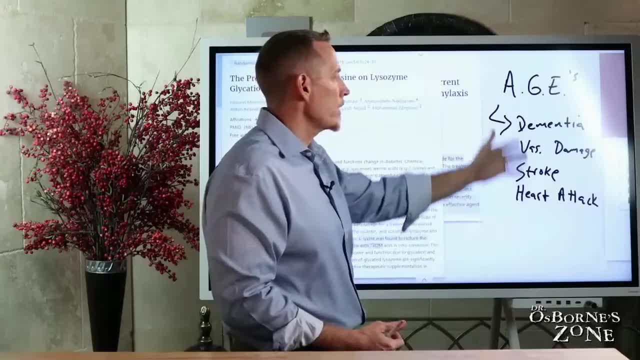 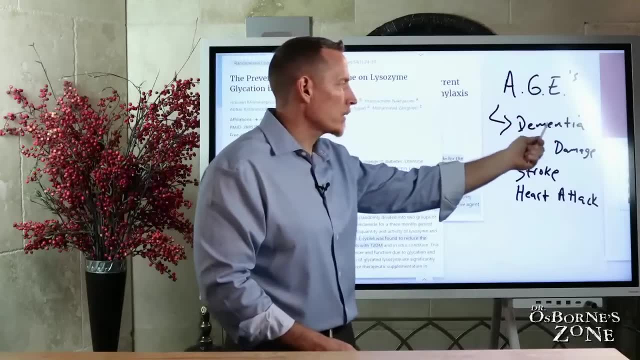 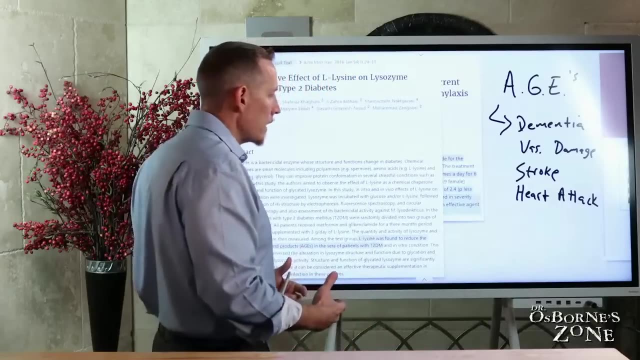 beneficial for the, for the reduction of age formation or, at begin, advanced glycation end product formation. these are the compounds and diabetics that increase the risk for a number of different diseases. so just another reason why lysine going to be important now. at the end of the day, what's the 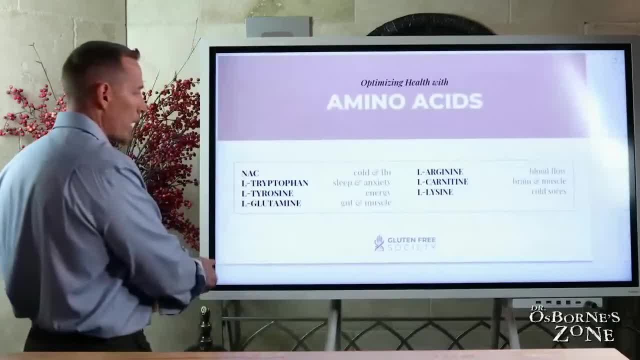 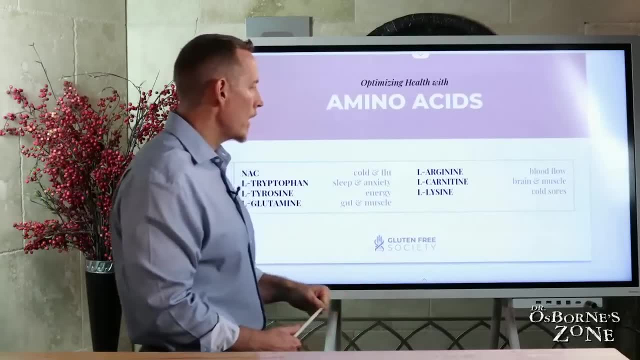 take-home message: we've got all these different therapeutic amino acids. I only covered a handful of them today, but you know NAC, tryptophan, tyrosine, glutamine, arginine, carnitine, lysine, all have tremendous, tremendous. 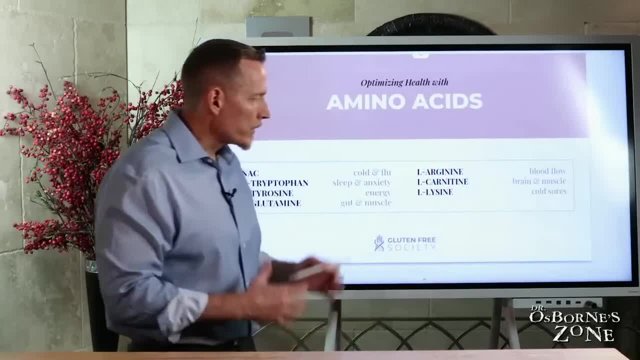 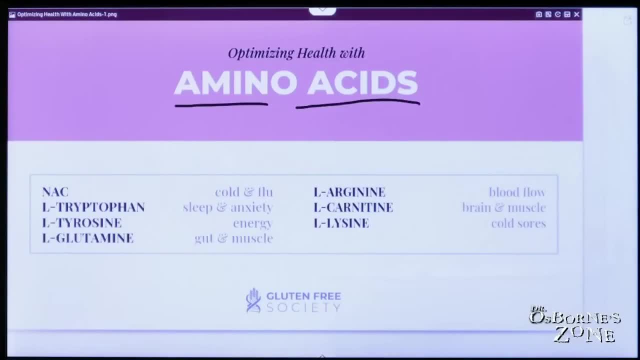 benefits and potential impacts and effects. The take-home message is number one. you've got to make sure you're eating so that you can get amino acids. Again, there's a huge rhetoric right now that, in order to save the planet, you somehow can't. 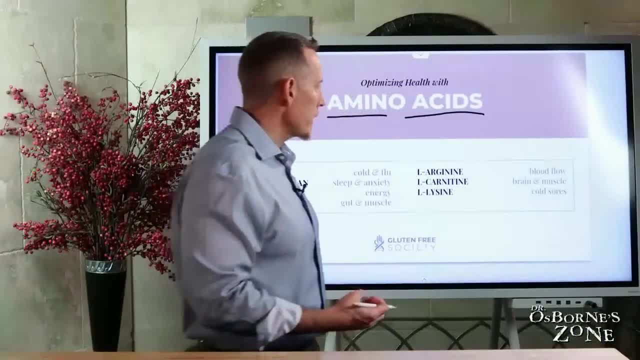 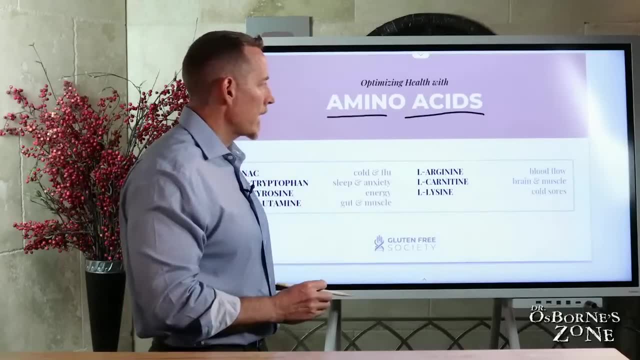 ever eat animal meat again, or you're murdering the earth And I think that's a well. we won't go there. It's a false statement. to make that statement, Humans need protein: Most of your amino acids, the vast majority of your amino acids, the vast majority of. 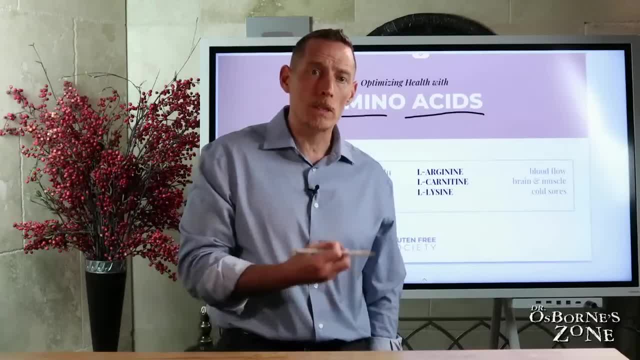 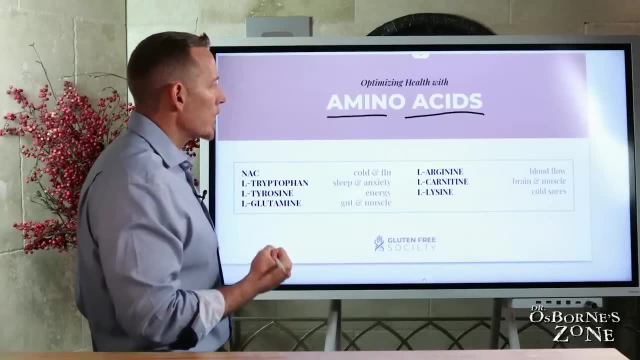 your what we call highly biological valued protein, which is the protein that contains the greatest concentration of amino acids. you've got to get that from animal-based products. Now, if you're on a vegetarian diet and you just, or you have a religious, 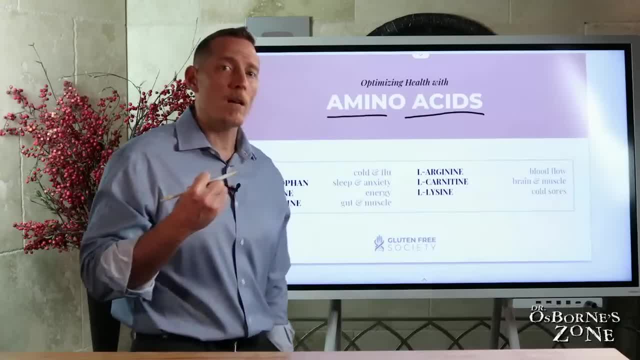 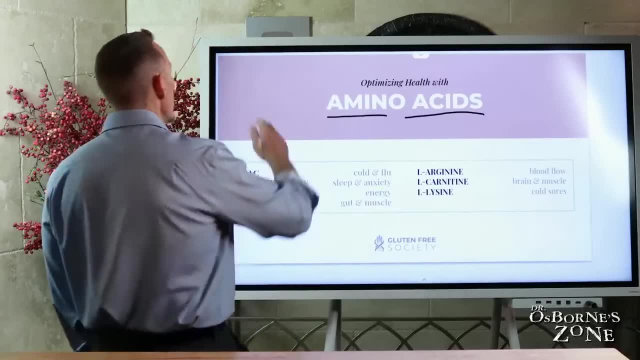 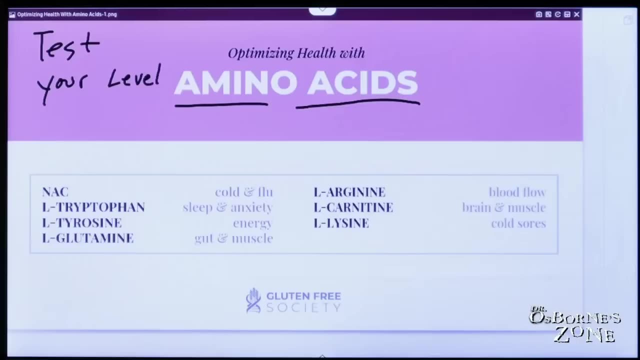 where you are a faith or just a generally, you're just an animal lover and you don't want to go in that direction. not judging, just simply trying to educate. if you're one of those, test your levels, Because I've talked a lot about you know vegetarian diets causing you know the potential. 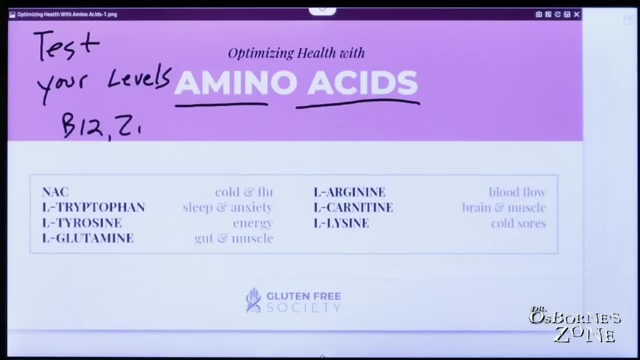 for low B12 and low zinc and low B6 and other- you know other- nutrients, but we haven't really tapped into that. And the reason why we haven't really tapped into this amino acid component- and I've seen this just a lot in people that go on vegetarian diets for long periods of time- is they're. 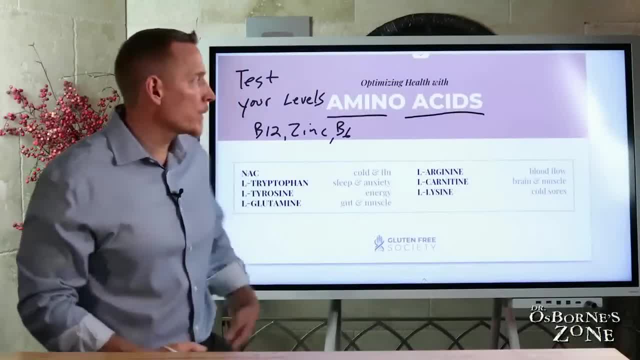 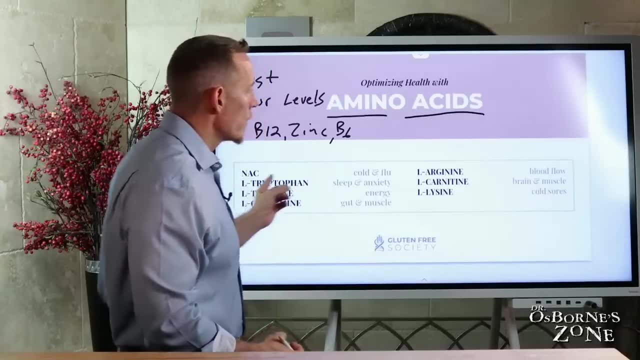 not getting adequate protein. And when you don't get adequate protein, remember what an amino acid is. it's the building block for protein. So you're not getting enough amino acids, then you run the risk of some major problems. Remember amino acids- not all of them, but there are 10 essential amino acids meaning. 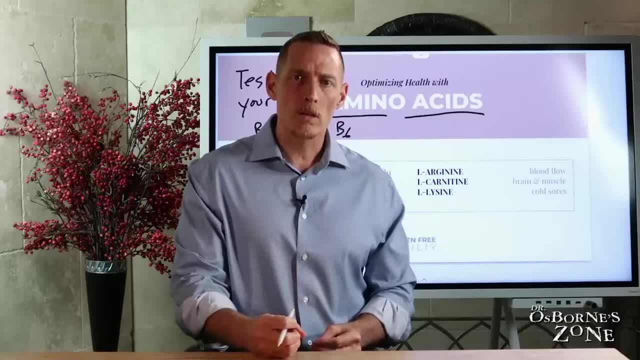 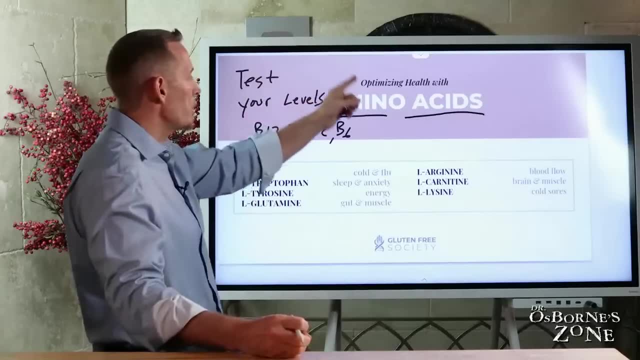 your body can't produce them. you have to eat them. Most of these are found more abundantly And and animal products than they are in plant-based products. So, again, if you're, if you're plant-based, you want to test. test your levels, because 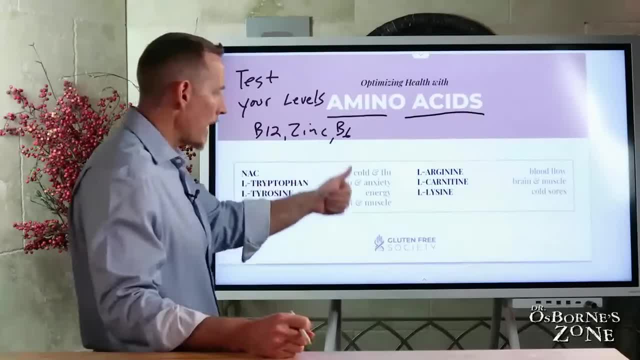 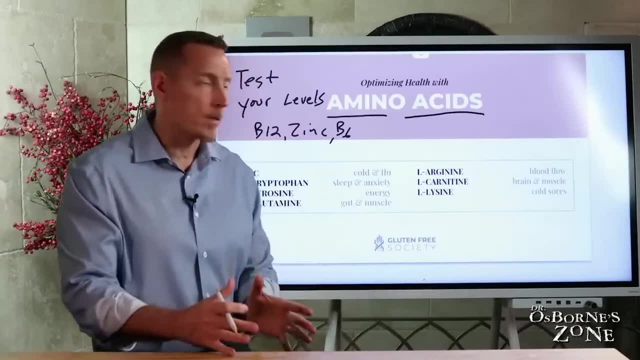 if you're low in these different things and you're developing, you know, high blood pressure, if you're getting sick on a on a more frequent basis, if your gut's blown open and you're trying to resolve leaky gut, whatever it is, it could be because you're deficient in one. 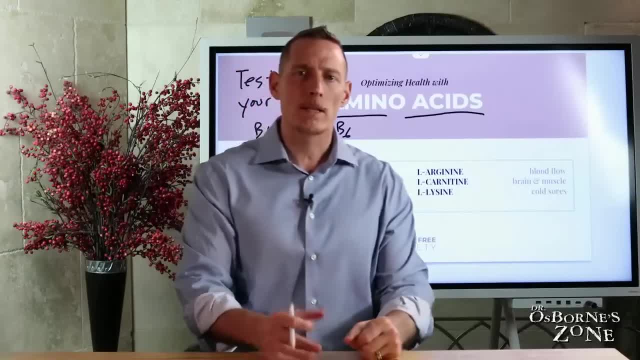 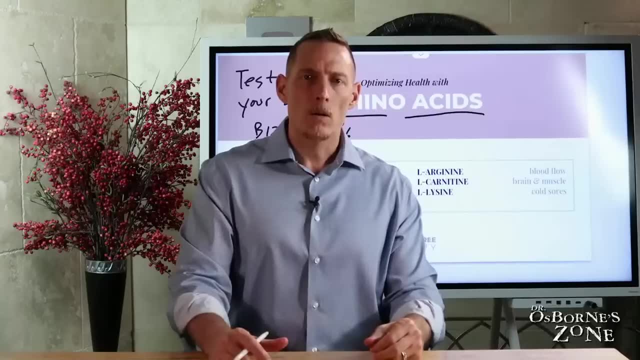 of these many different amino acids And it might just be as simple as getting tested and supplementing again. if you're not willing to eat animal protein, Supplementation, you know, is a possibility in today's day and age and I just encourage. 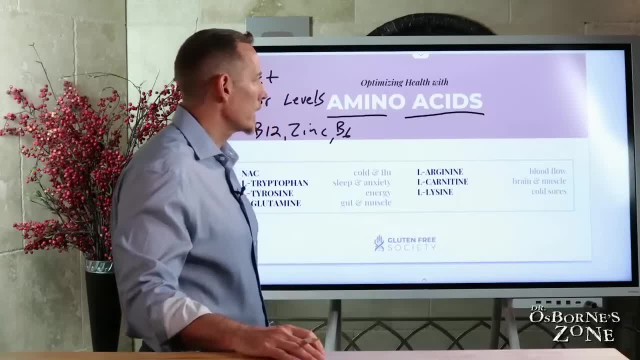 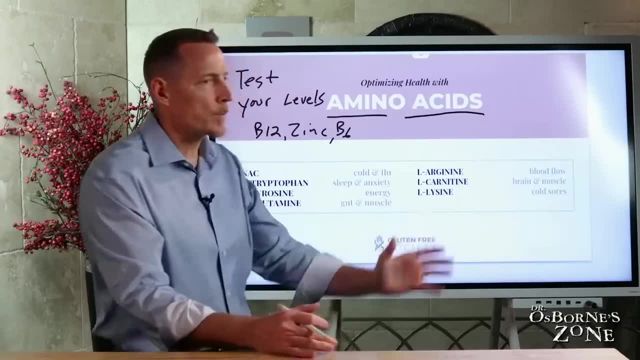 you to look at this and to encourage you to do it, if that's what your diet looks like. Now, those of you that you know aren't necessarily plant-based- you still want to have this looked at, especially if you're struggling with any of these symptoms on the list, because it 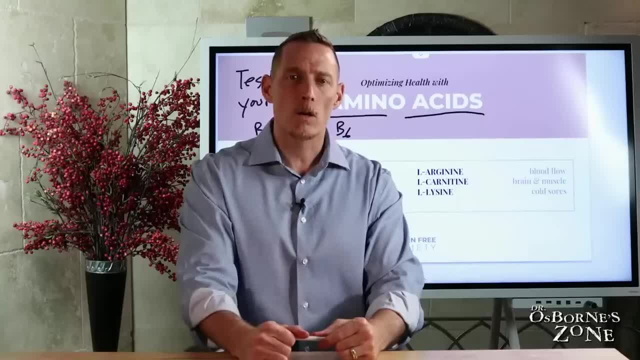 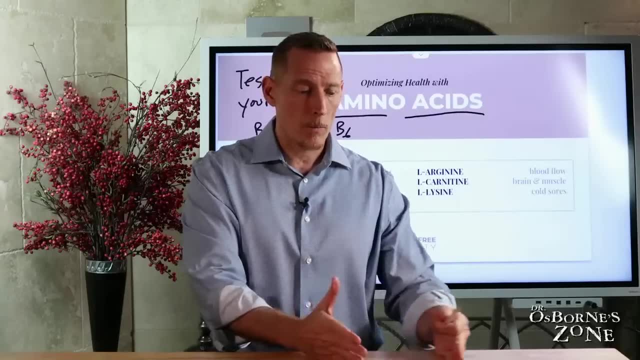 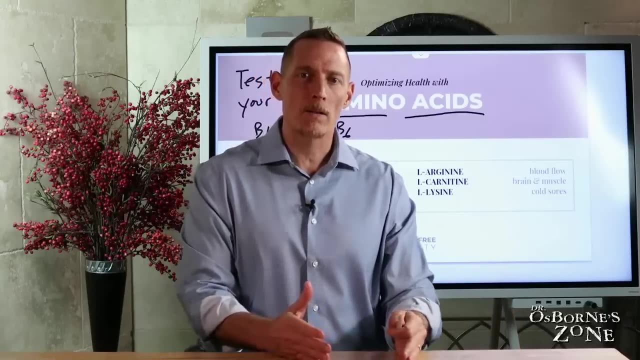 might also for you. your diets might also be too low in amino acids, So amino acids are very, very powerful. They often get ignored Usually. what takes all of the press? Our vitamins like like vitamin B12, and minerals like magnesium, but many people forget about. 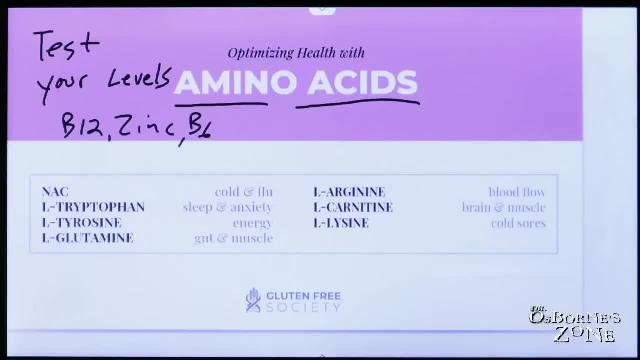 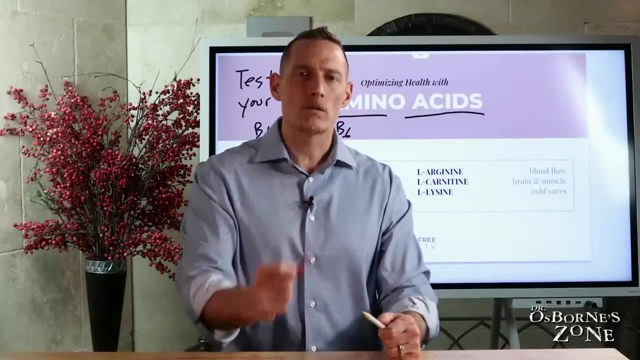 the power of amino acids. Don't be one of them. Now, below this, I'm going to put a link to a number of these different amino acids that we talked about. If you're looking for gluten-free varieties or grain-free varieties, you can check that. 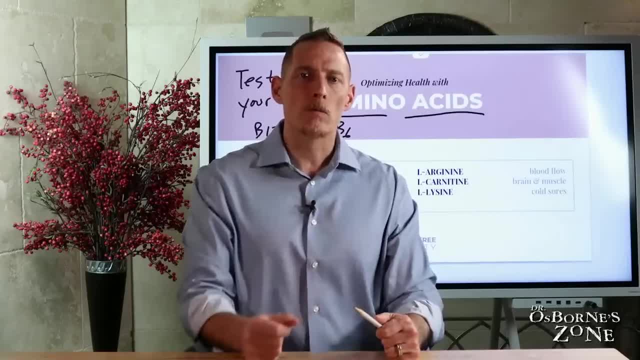 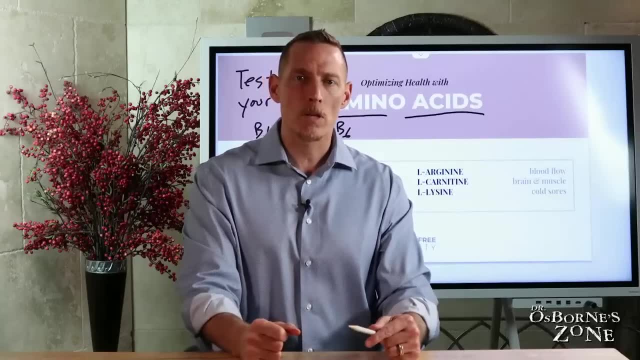 list out again below in the comments. I hope this was helpful for you. Make sure you hit that like button and, if you found it helpful, share it with your friends and family. Our mission here is to help save a hundred million lives, and I can't do that without. 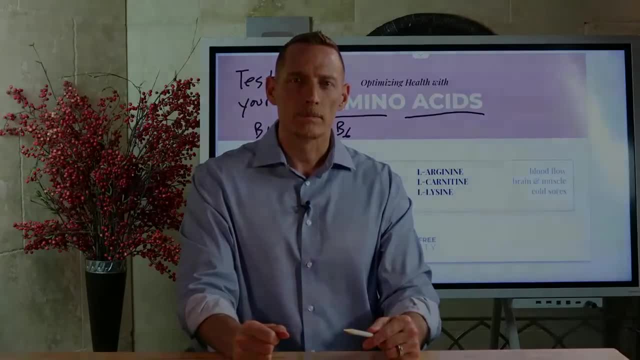 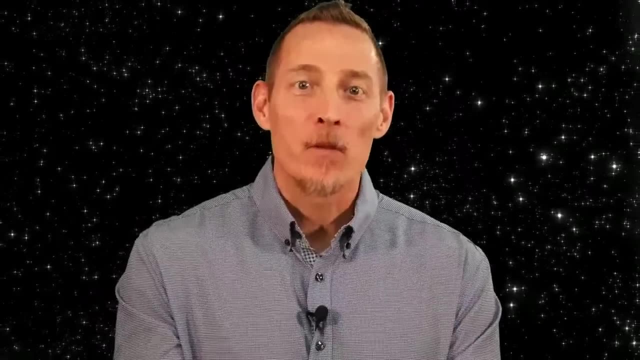 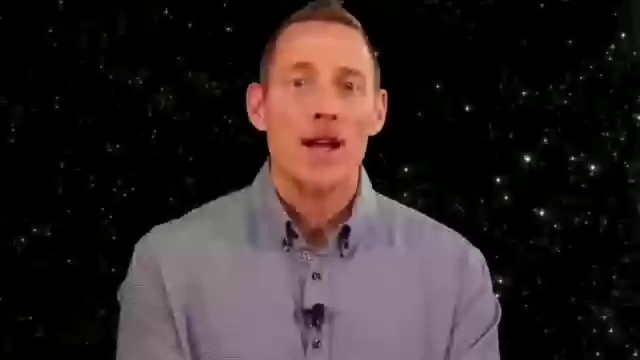 you Have a fantastic day. We'll see you next time. Thanks for tuning in to the Dr Osborne Zone. Don't forget to share, like and subscribe for more content like this and make sure you come back next Tuesday at 6 PM central standard time and Thursday at noon 30 for more episodes. 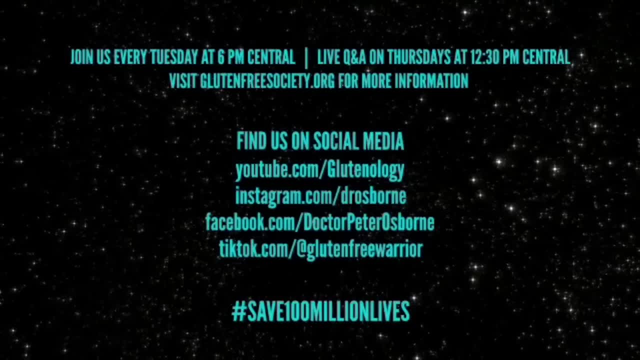 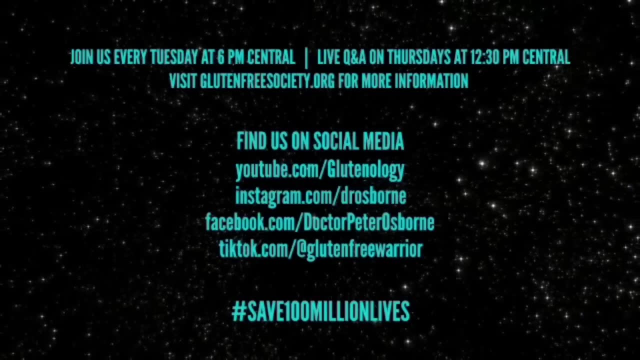 I'll see you then. Bye.